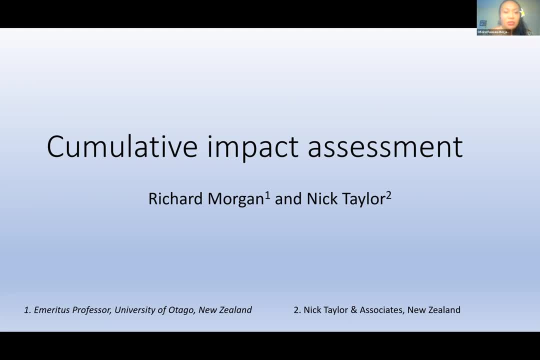 have not registered on the PNEA portal. you need to register so that you can log in and get that information, So do please visit that portal to get the resources that we upload from our trainings. They're all for free and it would be very useful for you to use. 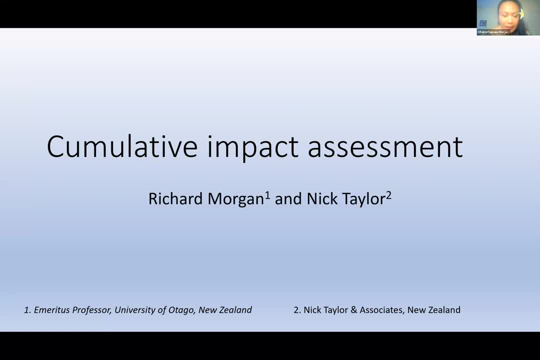 So for our for our session today. as you may all know from our training plan, our presenters for today: today is Emeritus Professor of Geography at the University of Otago-Donita, Professor Richard Morgan. He is the current chair of the New Zealand Association for Impact Assessment and Professor Nick Taylor. 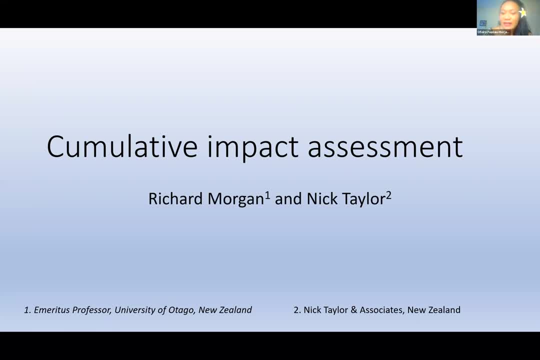 He's a social impact assessment specialist and former president of the International Association for Impact Assessment, And so just a brief overview of our module today on cumulative environmental impact assessment. Cumulative impacts are changes to the environment caused by an action in projects in combination with other past, present and future human actions. 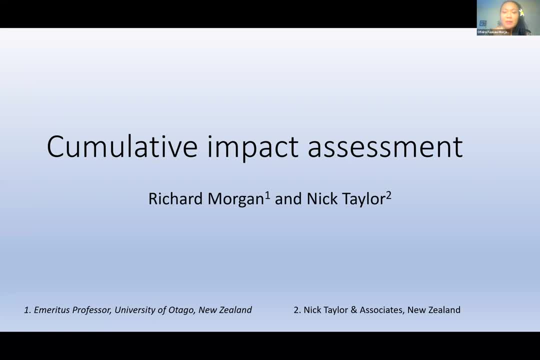 The importance of assessing cumulative impacts. Cumulative impacts is becoming more relevant and of interest among stakeholders because there are an increasing number of examples of conflicts between upstream and downstream users. CIA are useful when information on the combined effects of projects is necessary to provide confidence to developers, decision makers and the public about broader context and longer terms environmental conditions. 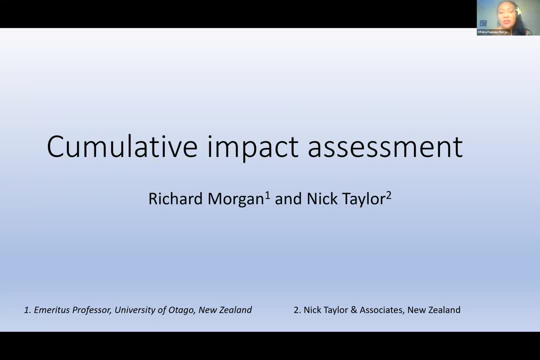 Likely to results from an action project. So this module aims to introduce participants to cumulative environmental impact assessments When they're needed, legal requirements, approaches and tools to describe the general process and steps of CIA scoping, data and information gathering, analysis and review, consultation, finalization and implementation, and share examples of industries that benefit from CIA. 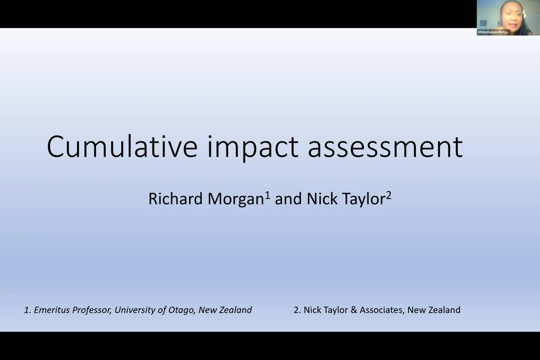 So it's going to be a very exciting session today and we have all been looking forward to Professor Richard and Professor Nick's presentations And just a few housekeeping matters. before I hand over to our presenters today, Please be mindful that our internet connection keeps going on and off. 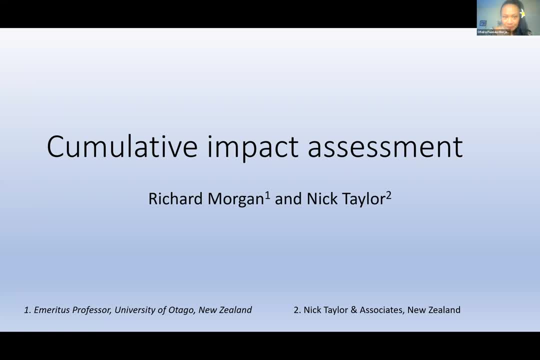 So just keep you up to date on all of the updates we have. Thanks everyone. It's been a really exciting time. Thank you, Be prepared for that. We've got some backup assistance from our overseas support staff, And so just be mindful of that. 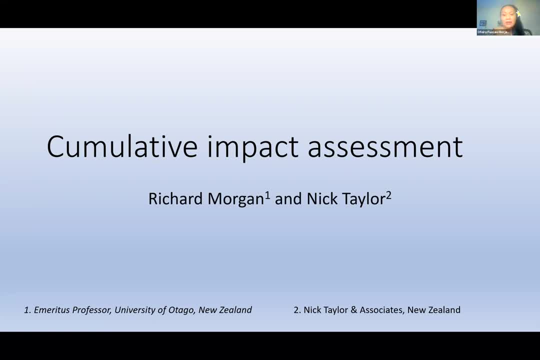 And then we also have our evaluation survey forms that we would really love for all our participants to fill in after our session, And please do click on that link. We will put it on our chat box and you can click on it and then just fill it in. 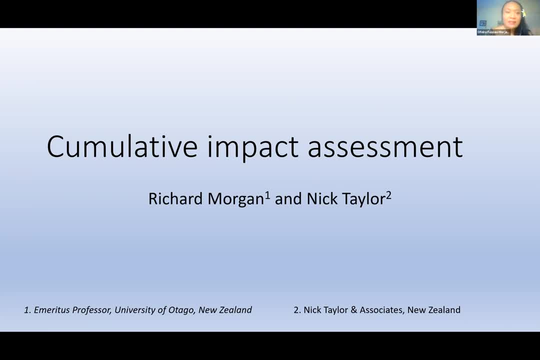 It's only, it's less than 10 minutes to fill in, So please do try and and use that resource for our trainings, which is very helpful for future trainings. And that's about it from my side. We do need to take a screenshot. photo. 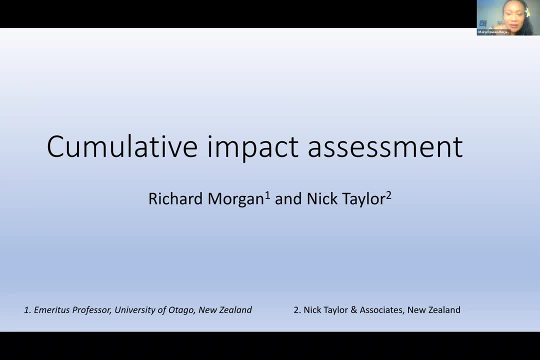 With all our participants who are connecting in. So if you could just turn on your camera and I, then we will take a photo before we go into our presentations. Thank you very much. All right, everyone. Let's see those beautiful faces. Don't be camera shy. 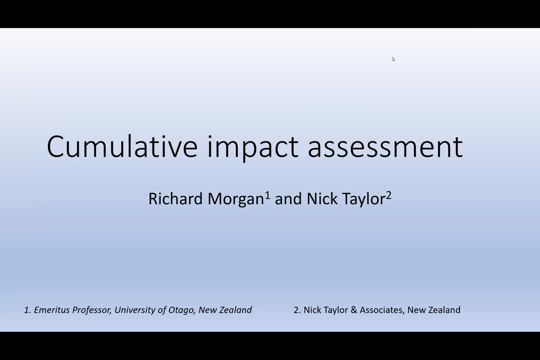 All right, that is good. Thank you very much. Okay, thank you very much. So now I hand it over to Professor Richard and Professor Nick. Thank you very much, sir. Thank you, Afeera Kia ora koutou. 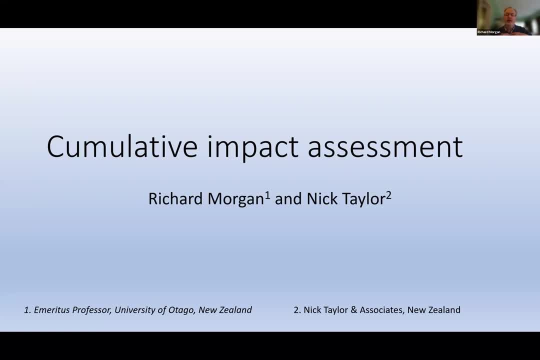 Talofa lava bula vinaka kia ora ana, and after that I'm afraid I'll start running out, But greetings to everybody. It's great to be talking into the Pacific, to our colleagues at SPREP and right across the region. 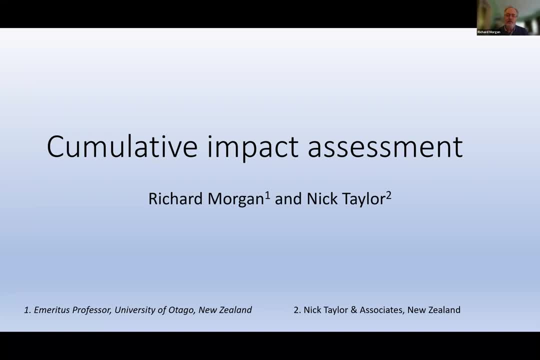 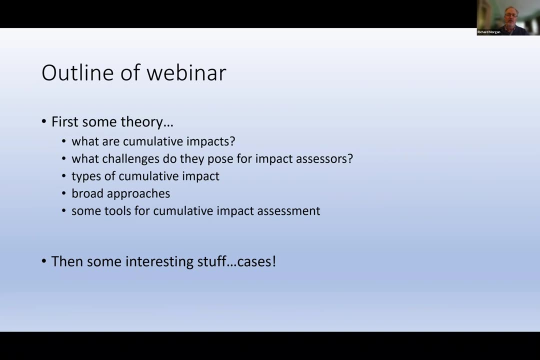 It's really good to be able to share some of this knowledge about cumulative impact assessment to practitioners right across the area. What I'm going to do: start off, I'm going to look after, if you like, what we think of as the theory, but not get too heavy about it- and then we get to the interesting stuff. 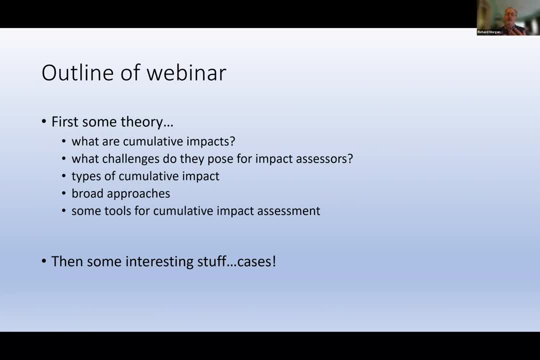 And that's when my colleague Nick Taylor will come in as a practitioner, being able to talk about how some of these ideas translate into practice and link the theory to the practice. Now necessarily going to talk about institutional issues, It's not for us to say how things. 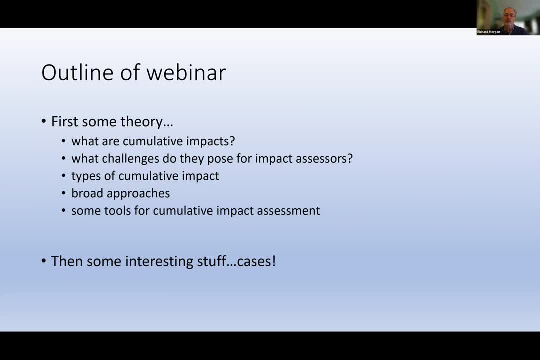 are done or should be done in different countries or different jurisdictions. That's for you people, as the people on the ground who know your systems, You know how to do that. What we're doing is providing our side of the partnership, which is talking about these processes, so that you can see. 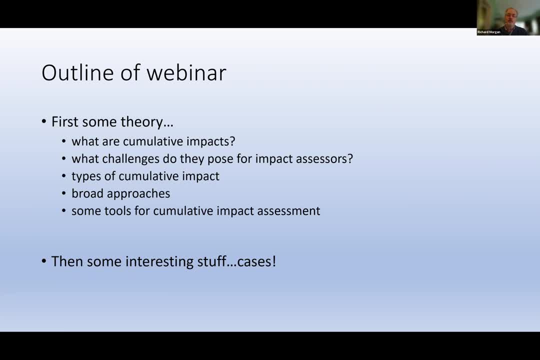 how they might be used in your context, in your jurisdiction, for problems that you deal with. So you know we're always willing to answer questions around that sort of material And hopefully we'll have time at the end, Or if you want to pose questions as we go through. 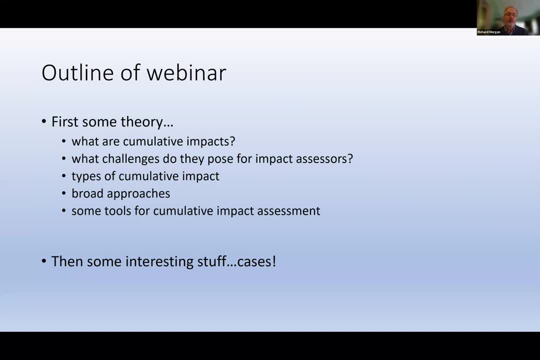 through the chat room. that's fine as well. Anyway, let me get underway. What I'm going to do in this first section is talk about what are cumulative impacts, and Afeera covered that quite nicely at the start. I'm going to reiterate that and just tease out a couple of things there. What challenges do they? 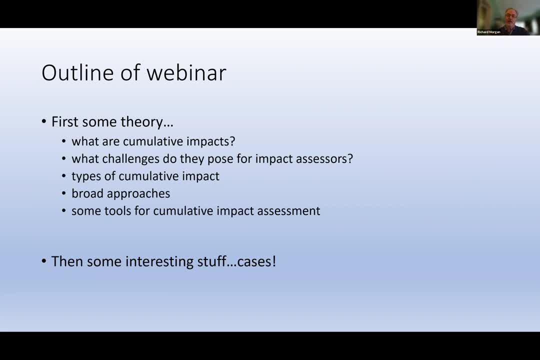 pose for assessors, especially at the project level. And that's really saying we need to think, perhaps not just through the project but at a rather higher level, a more strategic way of thinking, A little bit about types of cumulative impact, Something about the broad approaches and 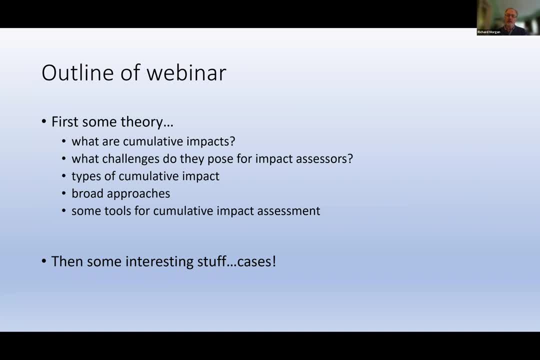 a little note about tools Now. as we go through, you'll see there's quite a lot of words on the slides And that's there so that afterwards people can go back and read some of that stuff in detail. And I'm not going to actually go through all of the detail, but I want enough to be there that it'll. 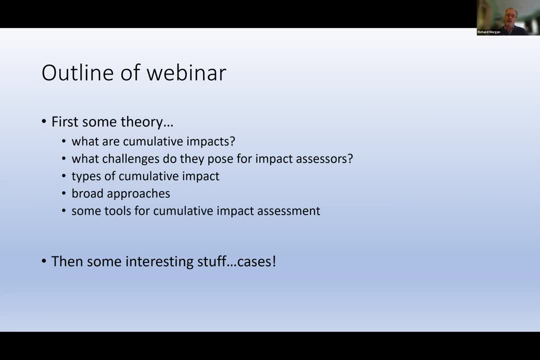 be useful afterwards. And also you'll see there are links to particular sources, guidance documents and things like that, where I've gone in and stolen things from and put them on my slides. You can go back to those guides and read more about it, And all except one, you can just click on a high-level link. 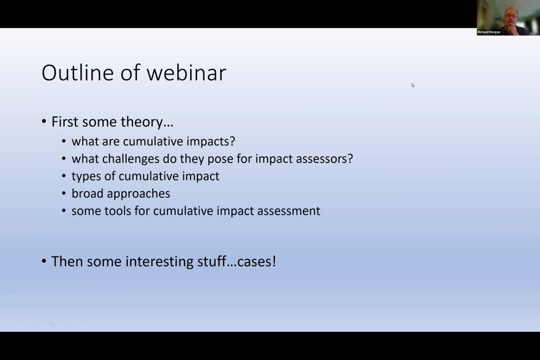 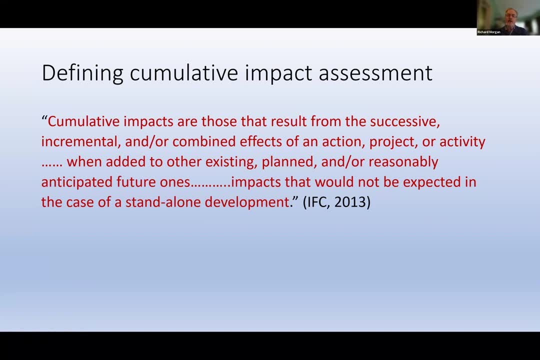 You can go back and read at the top and read these links and all. So there's a bunch of things that you can get from a library link or a paperlink and get over the Internet. So what are cumulative impact assessments? Cumulative impacts are all of those things. 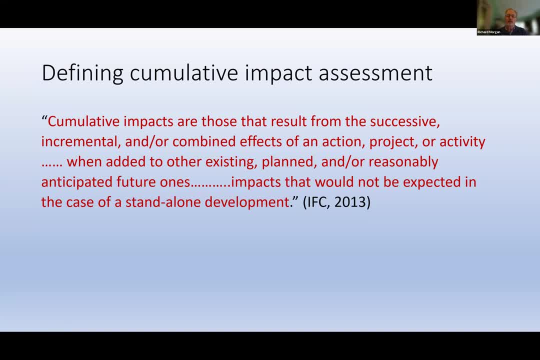 that we experience with a project, The successive incremental and or combined effects of an action or a project or an activity. So the things we we try and capture with a project impact assessment, something like that. But that's a pretty broad picture, aren't you? 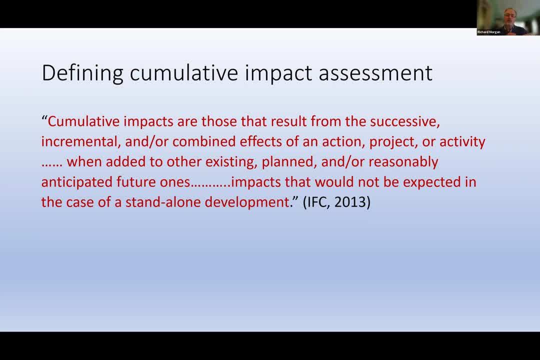 then we look at it in addition to other existing or planned or reasonably anticipated future actions. so we're looking at our proposal and we're thinking what else already exists or might be underway being constructed or, quite reasonably, in the near future, say the next decade, we know. 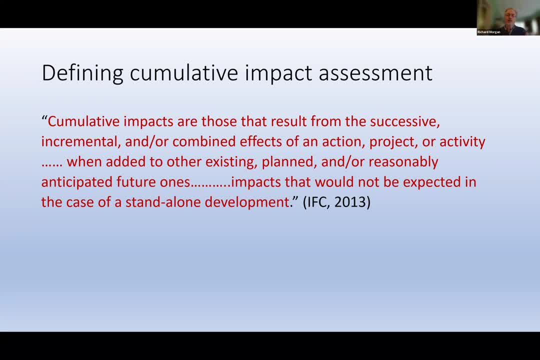 there will be things coming through and we're trying to put our project into that bigger picture and think about the cumulative effects of our proposal plus those other actions, and these are impacts that we might not expect if we just think about the standalone development, the one proposal. 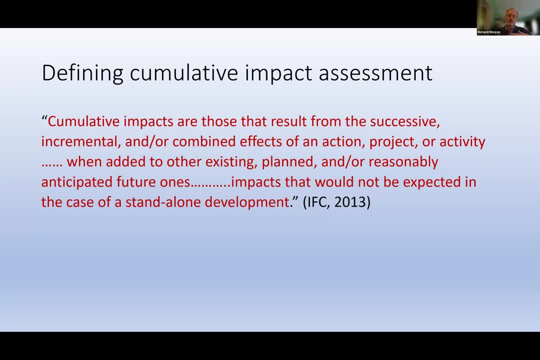 that we're looking at. so it's it's asking us to look more broadly and think more widely in time and space. and you see, that's taken from ifc, the international finance corporation. they've got a really good guidance document published in 2013. that link will be on the. 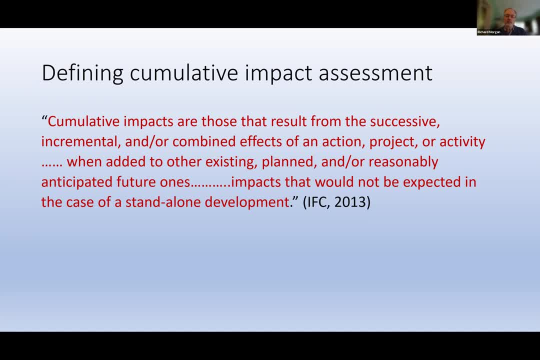 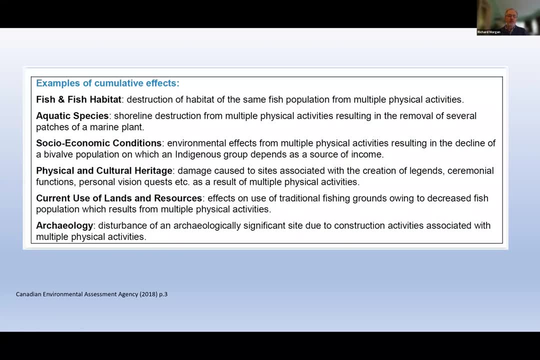 last slide of the, the powerpoint, so you'll be able to see where that is and access it. just mining some of the other guidance document- this is from a canadian guide- 2018 examples of cumulative effects. um, i'm not going to go through all of these, but just note that. 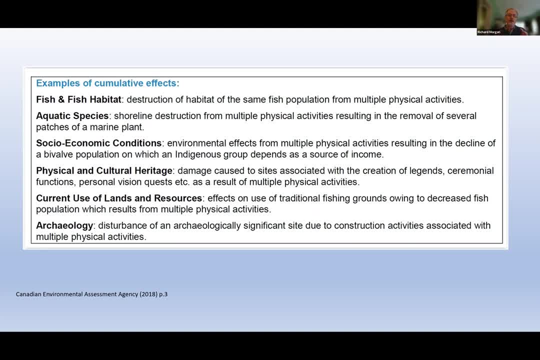 perhaps reflecting changes in the way canadian impact assessment is going. all of the examples seem to be aquatic and a good number of them relate to indigenous communities. first, nation communities, which is uh, which is interesting. that's something that's really grown in the canadian context. so they're examples of cumulative effects, for instance, a fish population. 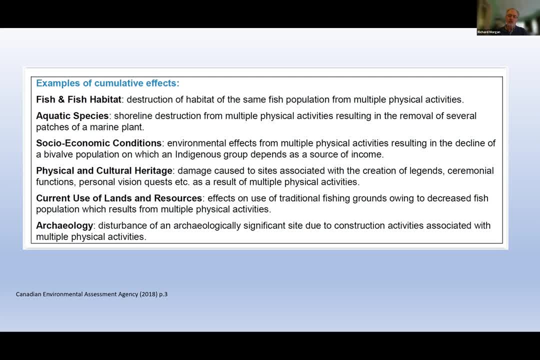 its habitat is being damaged, destroyed by multiple activities. so it could be drainage from the land, could be over fishing, it could be marine- sorry, marine mining and so on, different activities that might be individually subject to their own assessments, but from the point of view of the habitat of the fish, here we have cumulative. 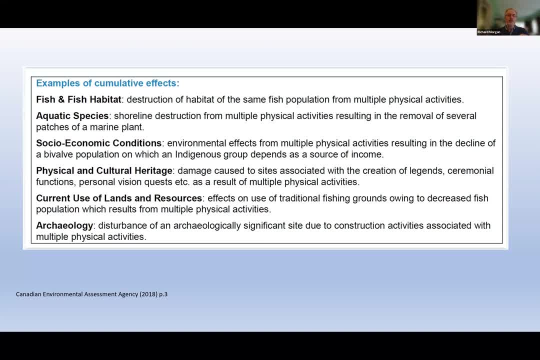 effects affecting that habitat. and the other examples are of a similar kind: the current use of lands and resources- traditional fishing grounds- being affected by multiple physical activities that lead to a decline in fish population and that ripples through to affect the communities dependent upon that fish population. so they've got a number of examples there. all of them emphasize multiple physical 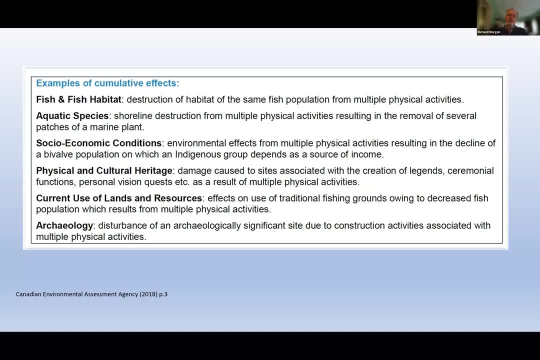 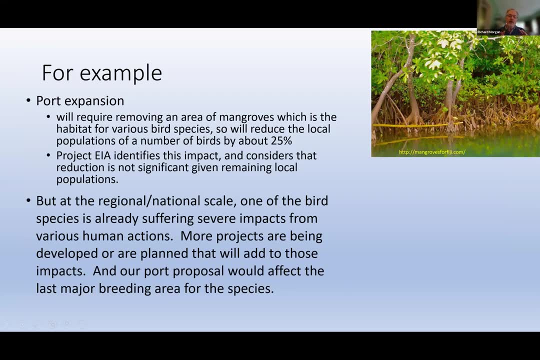 activities combining to affect a particular resource or an area, something that's valued. we're going to come back to that as we go through. i'll try to sort of put that into a little example. so if we can imagine a port on any of the pacific islands, an existing port, and we've got a proposal to expand it, 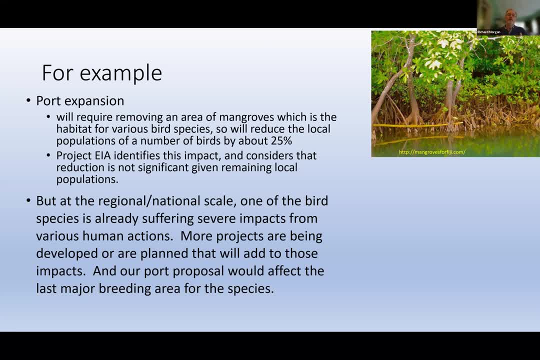 and that expansion will require removing an area of mangroves which have previously been protected- not protected but saved from any development. so we know we're going to have to remove mangroves in order to expand our port. we know those mangroves support a number of bird species. 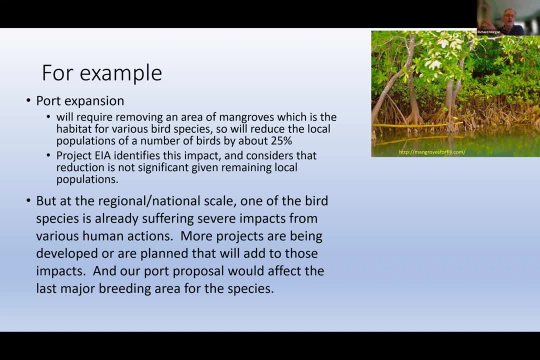 but we're only going to take a proportion of the mangroves, so we're only going to knock the bird populations back by about 25 percent. that leaves, you know, 75 percent of the existing population of birds. so not too much of an impact to that. 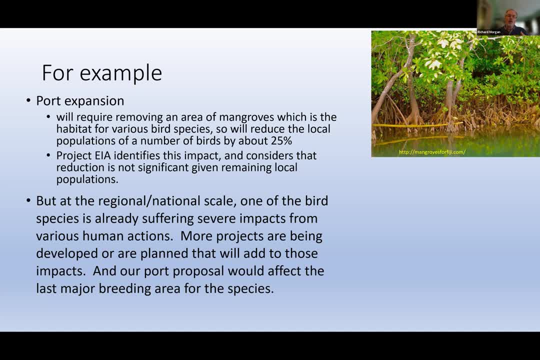 and so that's the impact. we think the trade-off for jobs and economic expansion and quality of life and so on is worth just a that little reduction in local bird populations. the project eia that we do for that expansion emphasizes the impact but feels that it's not. 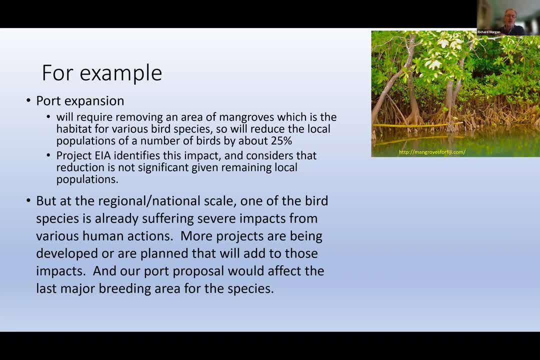 significant because we've got three-quarters of our local population still there protected. but if we then look at the national scale or the regional scale, we might see that one of the bird species that's in our local area is already suffering severe impacts from a variety of different human actions. it might be removal of mangroves. elsewhere it might be pollution. it. 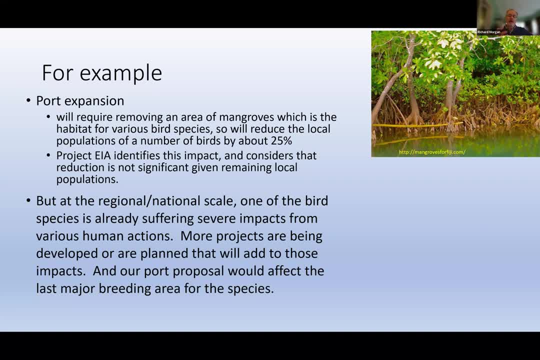 might be loss of fish that they feed on, it could be all sorts of things, and there this one particular species might be really suffering from all of those effects. and we know that continuing projects of that kind, continuing pressures, will add to those impacts. and then we find that our 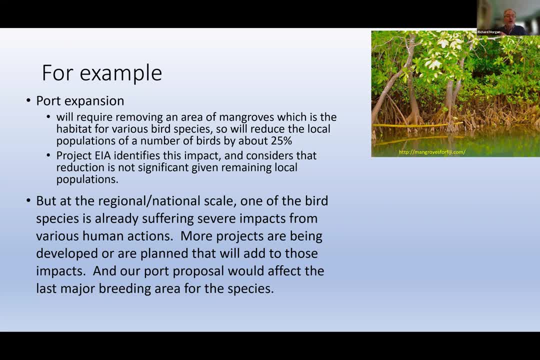 port proposal. expanding our port would actually be affecting the last major breeding area for that species and that changes our the way we look at that. loss of only 25 of the breeding population that now becomes quite a significant impact once we put it into that wider scale and recognize the cumulative impacts on that species from different activities. 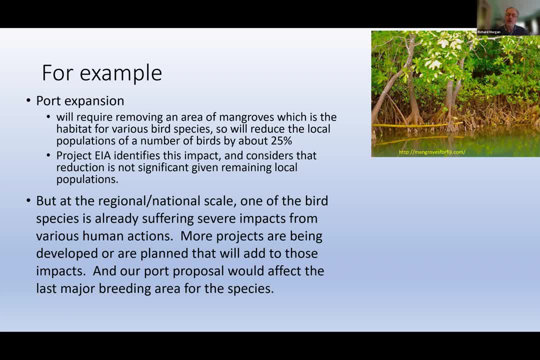 elsewhere, and so it raises the argument. first, we need to have some sort of cumulative impact dimension to our project assessment. so part of the project impact assessment. but it also suggests that we need to be looking over the resource across the area, so an area-based assessment of the status of that. 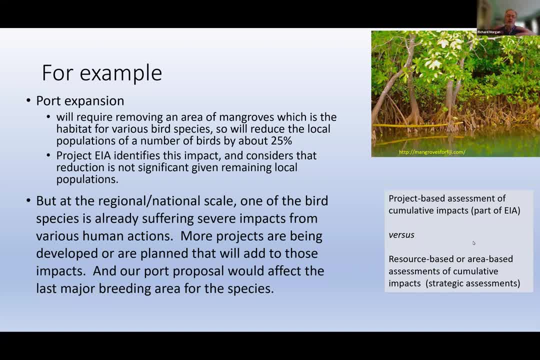 resource- in this case that bird species- and thinking about the cumulative action of all the different things that are putting stress on it. so we can attack this from the project side and extend the cumulative impact considerations in our project eia, but where we might also want to. 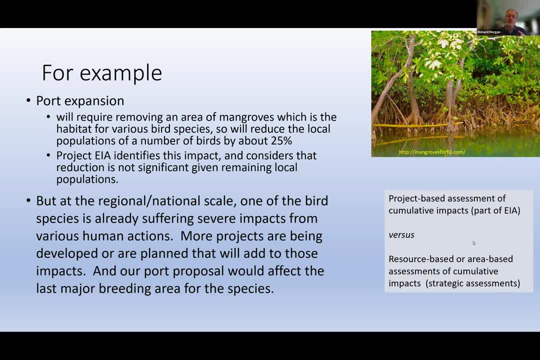 think about doing a regionally based assessment, an area-based assessment of that particular resource, that species, and that's what we're going to see as we go through uh. you know this theory, but also next uh examples that sort of interplay between the project producing some information about cumulative impacts, but also the benefit of taking a more strategic 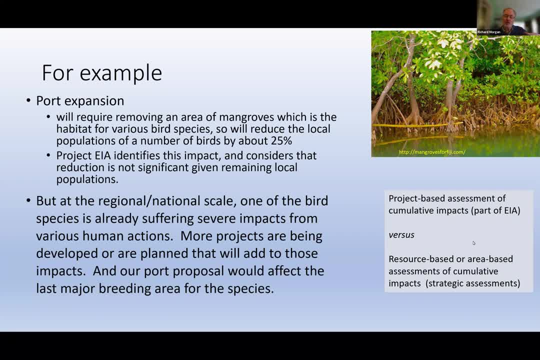 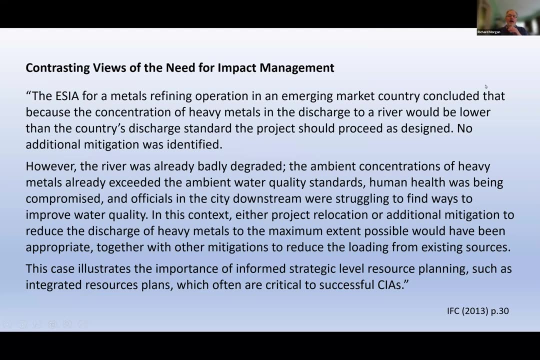 perspective, and a lot of the literature now is pushing that resource-based, area-based assessment of cumulative effects as being perhaps the way to go. more generally, uh, i think i'll skip this little example, because it's really just saying the same thing, but it's a direct strategy, but it's a more systematic and it's not a very strategic one, but it's a more. 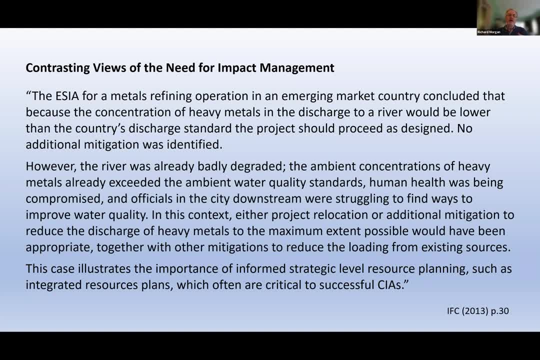 objective and it's really not a very strategic one. so this is one is one you've got to take into account if you only have a particular resource and another is not necessarily a, a native resource element you're just going to think about, uh, and i'll leave you with quite a few. 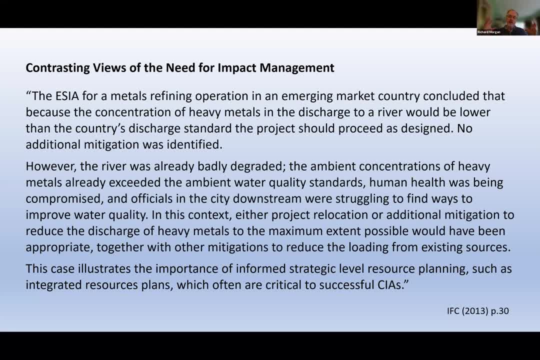 and so we actually need to step back and think about that bigger picture and not just authorise projects simply on the basis that they meet a simple standard. so it's that one might be worth having a little read through afterwards, but it's saying the same, the same message, can't just. 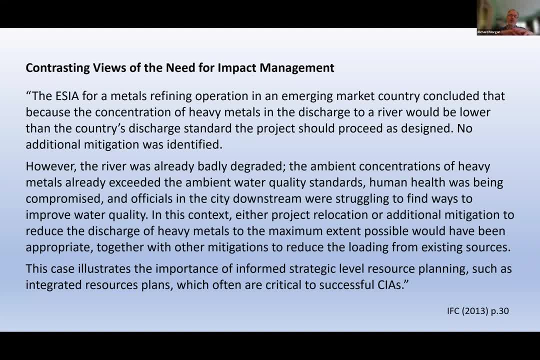 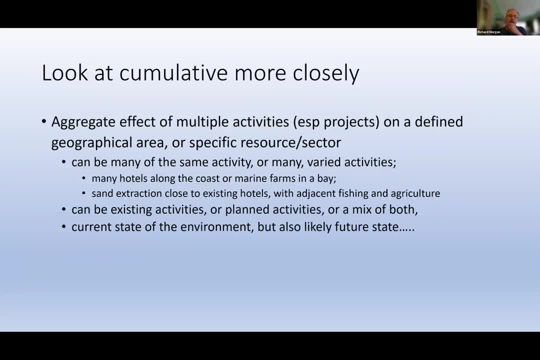 necessarily rely on straightforward project assessments. we have to step back and look at the the bigger picture for some of these issues. so looking at cumulative effects, cumulative impacts, a little more closely. so we've got the idea that we're looking at the aggregated effects of multiple activities in a defined geographical area. so it could be. 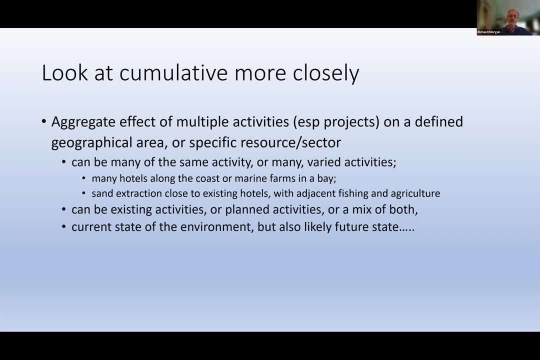 across a whole island in the pacific. we're doing perhaps lots of similar kinds of agriculture or won't come as too much of a surprise- maybe lots of hotels around the coastline, or maybe we're going to promote lots of marine farms in an area, a marine area. lots of repetitive. 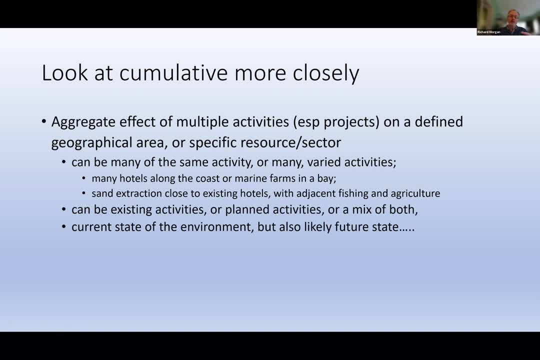 the same things in an area, but it might also be different activities focused on a particular area. so sand extraction close to hotels, close to in-shore fishing, with agriculture nearby using fertilizers and pesticides, and the totality of that, the aggregation of impacts, may be affecting local communities. 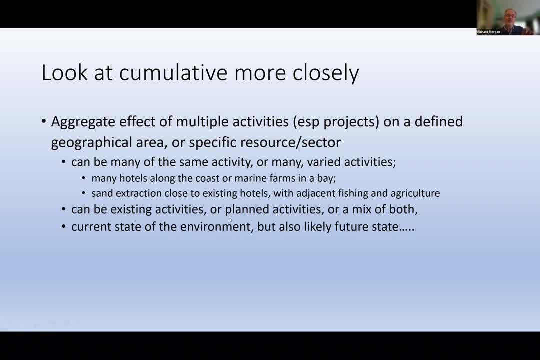 so there can be also existing activities. there can be activities that are planned, not yet existing. usually we're trying to mix both of them and, with sort of looking at the current state of the environment and that might be already affected by multiple activities, we're also projecting the environmental changes into the future and that in particular, means we're 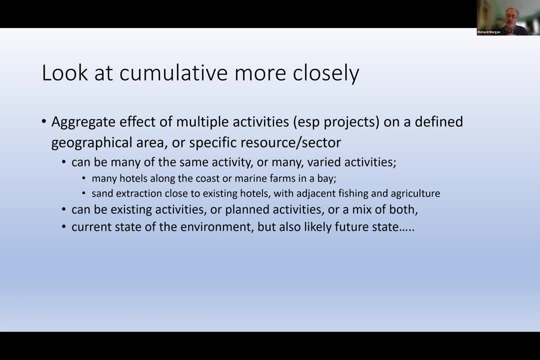 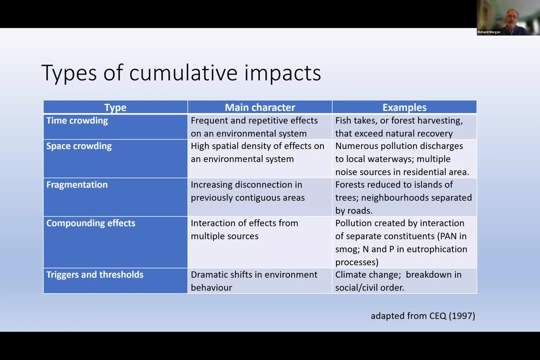 trying to factor in things like climate change, which is becoming, of course, absolutely critical to all of these uh considerations. now, uh, i've taken this from a us, the council for environmental, environmental quality, which is their core administration unit for impact assessment. it's an old document and i've just stolen some of the ideas and updated them again. i don't want to. 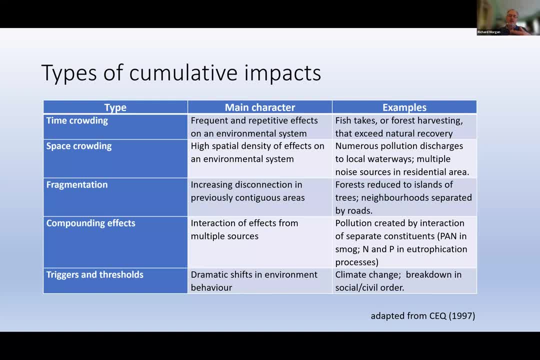 go through this in great detail. it's sort of a resource and you can follow up in some of the guidance. what it's doing is saying: um, we think of the cumulative impacts in in some different ways and it might be that we are using elements of all of these when we're analyzing impacts. 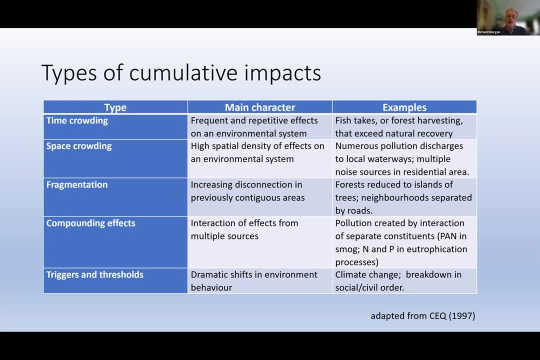 so typically we would look at, say, space crowding, that is, lots of activities in a defined geographical area. so it might be the example of pollution discharges to a river from different sources, different noise sources- in a residential area affecting a core population fragmentation is an interesting 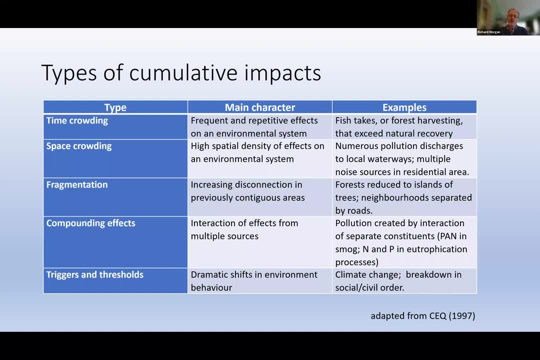 one because it it's not one we think about, naturally, but, um, if we are looking at a forest area on a geographical area and we start taking out some of that forest to leave islands of trees over a long period of time, we end up with little islands. what we're dealing there. 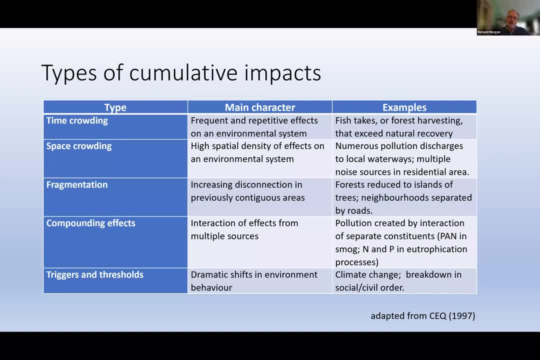 is a cumulative impact on that forest that steadily reduces its ability to to function as an ecosystem. we isolate key parts um it. it separates breeding populations of birds, animals and so on. regeneration fails and it gradually will hit a tipping point when the whole system fails. and you can do that with uh neighborhoods separated by roads if we keep. 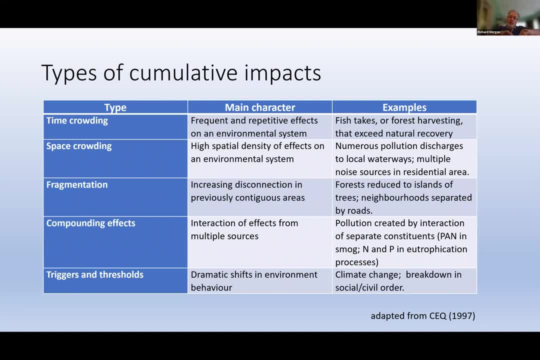 separating, putting roads through an urban area, we're slicing up the neighborhoods and we're we're destroying the social um the neighborhoods, the social processes, the amenity, the economic side of things, simply by putting roads through. and that's a cumulative effect over time of individual actions and can be, you know, really important, something that's often 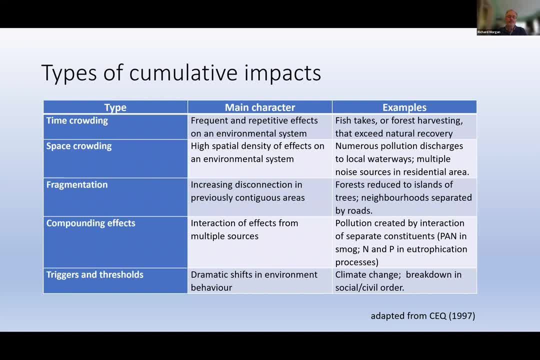 talked about for cumulative impacts is interaction effects or compounding effects, often associated with um pollution of different kinds, where we bring different constituents together and they can interact and create more of a problem than just the the problem of the individual constituents. the classic one in the literature from the old days is what we call pan, which is uh. 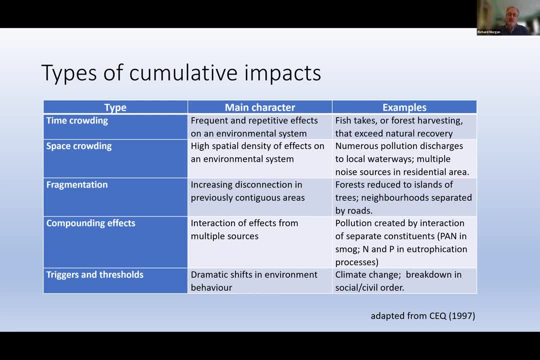 photochemical smog, peroxyacetyl nitrate, i think, from memory pan and in california it was, you know, nitrous oxides and ozone from car pollution, ultraviolet light promoting a reaction that produced this peroxyacetyl nitrate, which was a very nasty 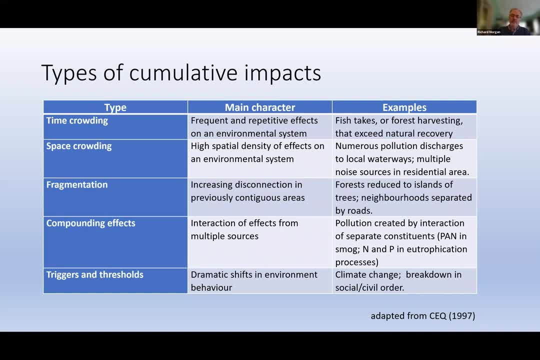 pollutant of uh natural life- i was seeing plants and such like- but also is a real health problem as well: nitrogen and phosphorus going into waterways and so, um you know the the amount of water right now in the waterways is quite high. uh, the amount of water that has been produced in those many Bundesländer and the waterways. 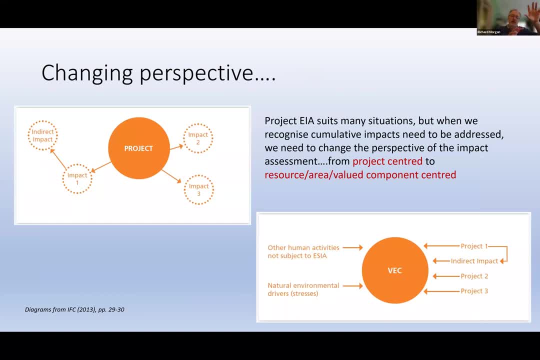 in the waterways is probably like eight to 10 percent of the water that's produced in those communities, so, um, so the other things i think is important in terms of the allergens is the um, um, gross and the, but there were some other things coming up there but, as i said, we have 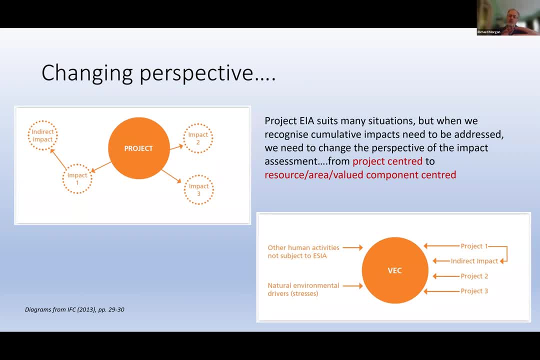 you know, as i said before, the Subaru and ferris wheel were justお waterway and i think that they were just getting a little bit more of trying to understand what those cumulative effects are over a period of time, things that we need to recognize and respond to. 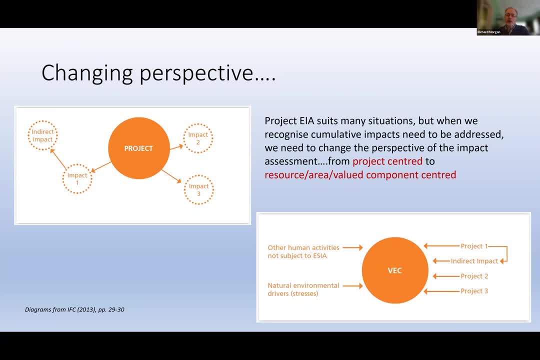 So that's the challenge And the changing perspective that's required often is to move from simply focusing on our project and doing our project impact assessment and just thinking about the immediate impacts and indirect impacts and trying to capture that in an impact assessment. 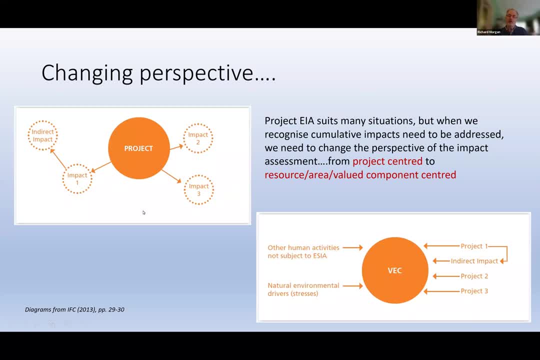 and moving through to think about the wider picture and therefore thinking about our project and its impacts, but also that there might be other existing projects, other activities, there might be other activities that are not going through the assessment process, and there will be natural environmental drivers. 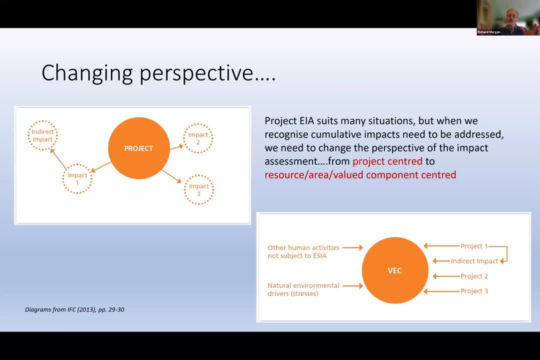 such as climate change over time, And all of these are going to be affecting a particular geographical area or a key resource, or what we call a valued component, And I'm sure many of you will have come across the idea of valued environmental components, VECs. 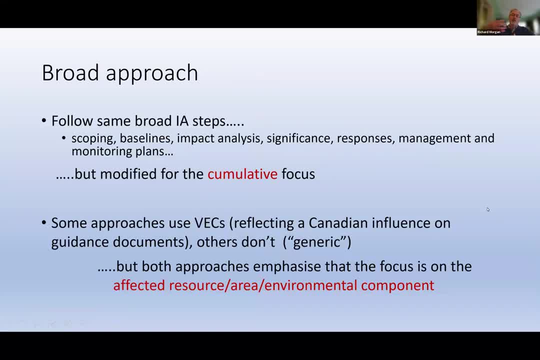 introduced by the Canadians and wherever Canadians have an influence on impact assessment and wherever Canadians have an influence on impact assessment, you will see that referred to. Personally, I have one or two problems with it, but I think the idea of focusing on valued components 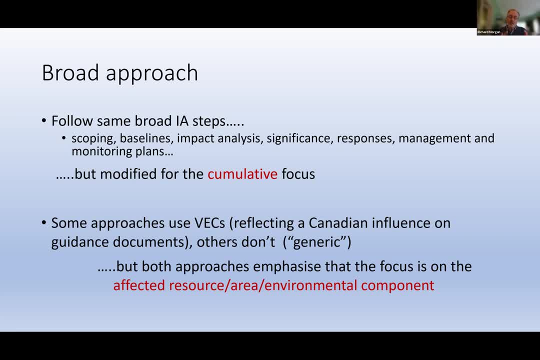 is a really good way of thinking about some of these particular issues. So when we talk about approaches to cumulative impact assessment, the broad approach is very much based on classic impact assessment. So when we talk about approaches to cumulative impact assessment, the broad approach is very much based on classic impact assessment. 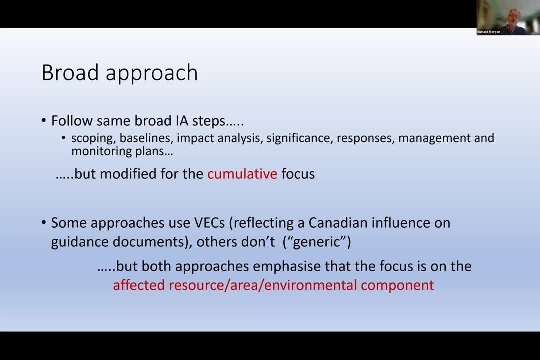 So we need to do a scoping of the potential impacts, establish our baselines, do the more detailed analysis of what the cumulative impacts might be, think about significance, therefore decide what we need to respond to, how we're going to do that. 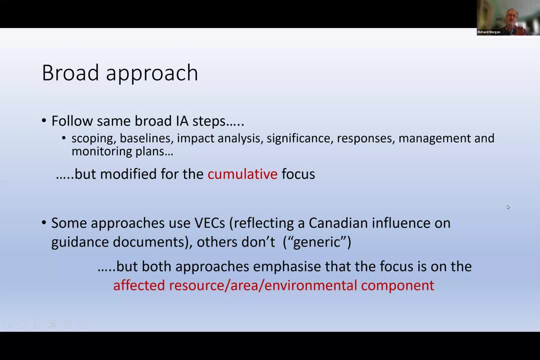 and then implement our action and manage and monitor those impacts. monitor our management and then implement our action and manage and monitor those impacts. and then implement our action and manage and monitor those impacts, as well as the specific impact demands. 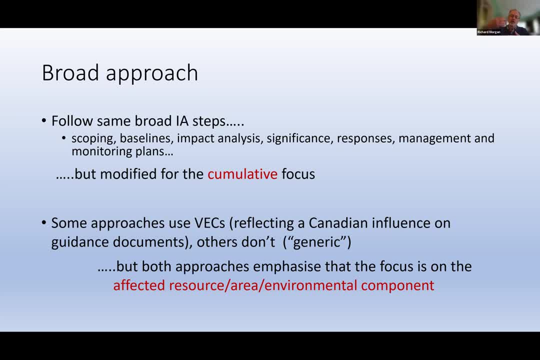 So very familiar steps for any impact assessment process. So very familiar steps for any impact assessment process. But of course it's got to be put into the cumulative context. But of course it's got to be put into the cumulative context Now as that previous. 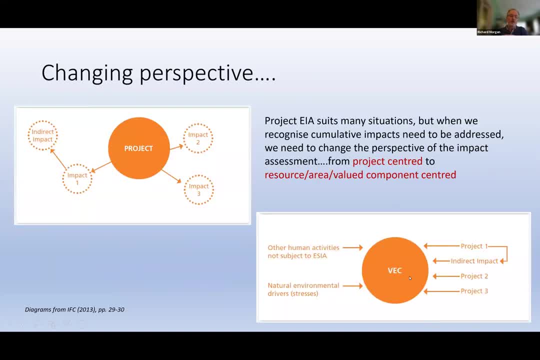 Oops, sorry, it goes the other way. Oops, sorry, it goes the other way, As that previous slide suggests, some of the guidance, and the IFC guide, which was written by Canadians, has this in it. They're suggesting that we use explicitly: 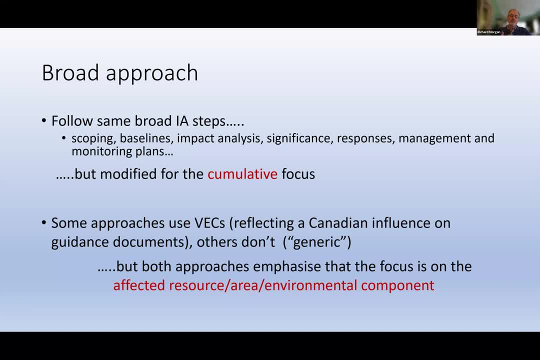 the idea of VECs. that's fine. The idea of VECs, that's fine. For some people that's a you know- makes it a very straightforward way to think. but some of the other guidance documents, especially coming out of the US and various other places, don't use VECs. 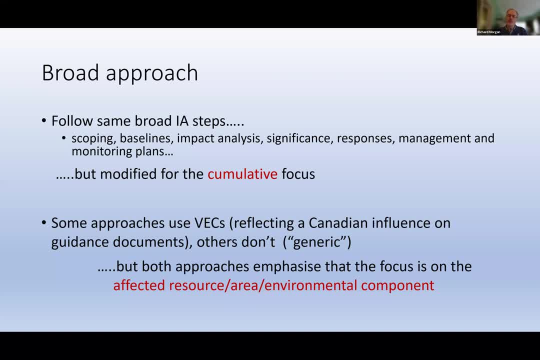 Now I'm thinking of those as generic approaches, But in fact they share the same basic idea: that we emphasize the shift in focus from the project through to the affected resource or the affected area or the valued environmental component, ie a resource, species, a river or whatever that we want to, you know, look after. 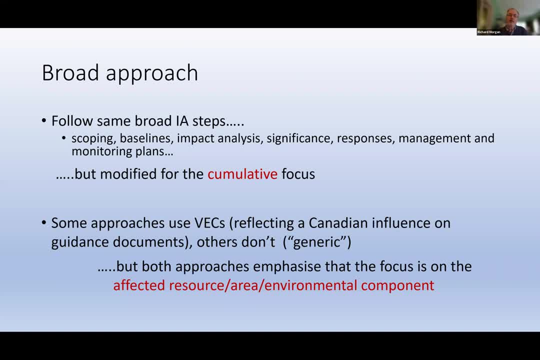 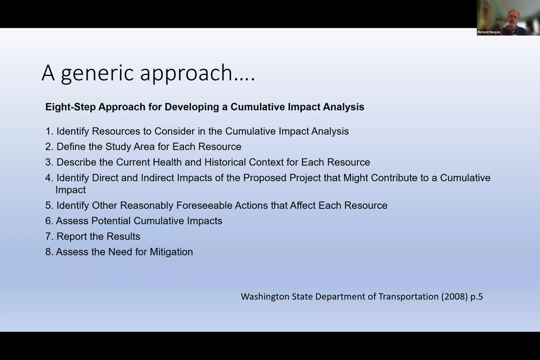 So it's that change of focus is the key thing. So I've picked out a generic approach that is being promoted in various states in the US. This is an example from Washington, Washington State, their Department of Transportation. They stole it from the Californians, who stole it from the Texans who, you know, they all borrow. 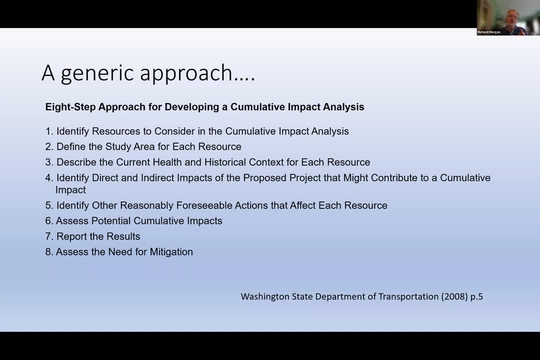 So that's good, We're going to borrow it. The reason I've taken it as an example is that it's quite straightforward. It follows a good traditional impact assessment process. The steps are quite straightforward and they provided a nice little hypothetical example which allows us to see how it actually would work in practice. 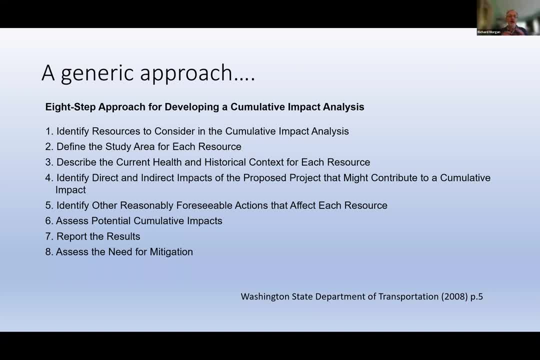 So when you look through steps one to eight in their eight step approach, you can recognize it's quite a straightforward thing to do: Identify the resource That you want to focus on in this cumulative impact assessment. So straightaway we're moving from a project focus to a resource focus. 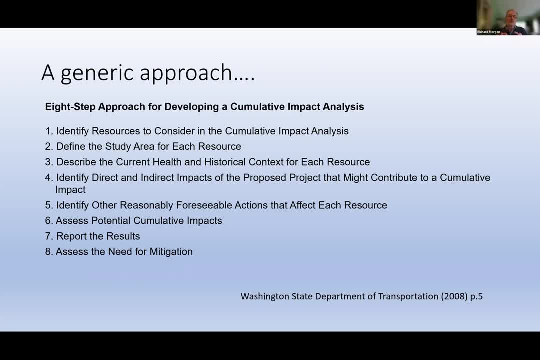 Define the study area for your resource. So we get that spatial but also probably a temporal extent sorted out: Current health and historical context. So those are our baselines. if you like Number four, then we do the analysis: Direct and indirect impacts of our proposed project that might contribute to the cumulative impact on this resource. 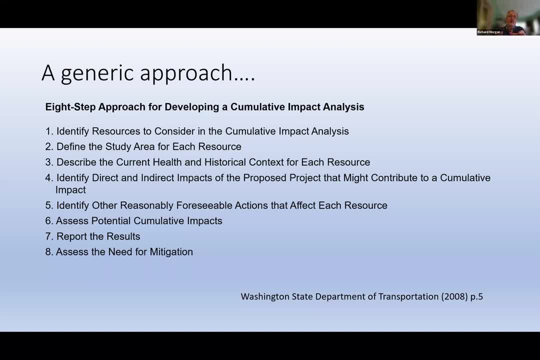 So we're looking at what we're going to add as impacts on the resource And then, step five, what the other activities- reasonably foreseeable activities in the future- might add. So we've got the current health, so it might already be stressed. 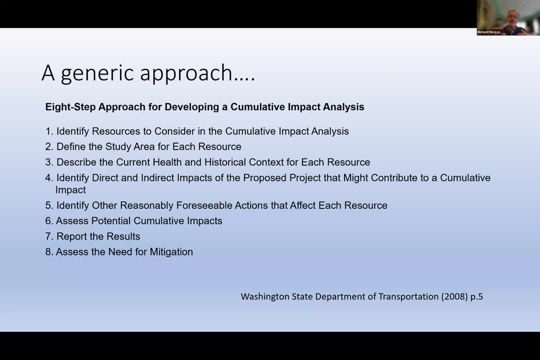 Then in number four, we're looking at how we're going to add to that potentially, And then number five, how other activities might add to that And therefore the cumulative effects of all of that on this key resource that we're concerned with. 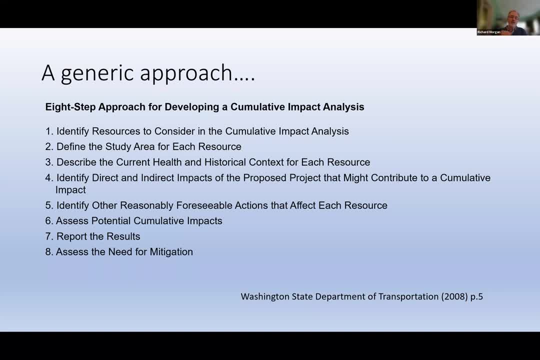 And that's number six is pulling all of that together- Assess those potential cumulative impacts, Then report them and assess how we're going to deal with them in terms of mitigation. That's quite a familiar way of working in an impact assessment way. 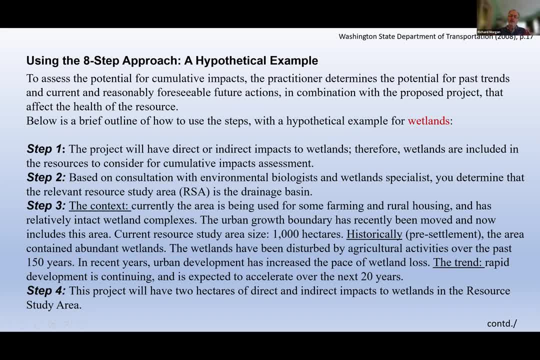 The eight step approach. a hypothetical example you'll be very pleased to know, as this goes over two slides, I am not going to recite this word for word over the next 15 minutes because Nick, my colleague, would definitely go to sleep. 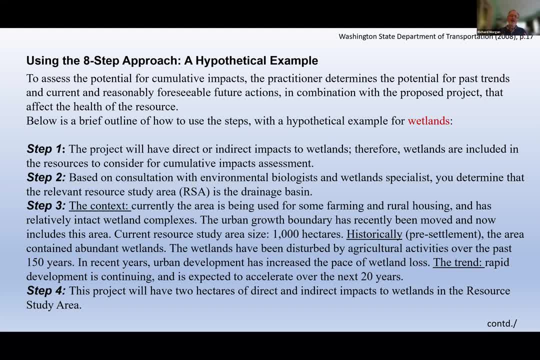 I see he's on mute so that the snoring can't be heard. Thanks, Nick, But what I want to do is this is: you know, this is something that you can go back to afterwards and look through the detail yourself, But I'm just going to pick out the key things so that you can see how it's working. 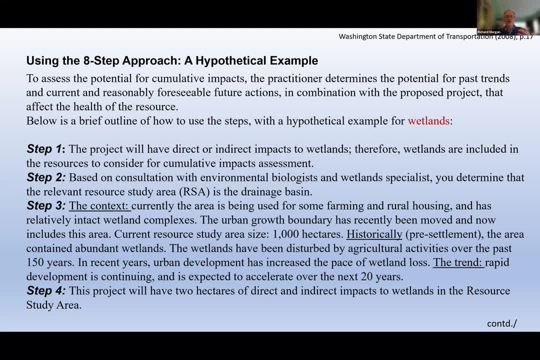 So imagine we have a project. It could be the port expansion, It could be a major tourist development project. So tourist development doesn't matter. We've got a proposed project But it's near, in this case, a major wetland area. 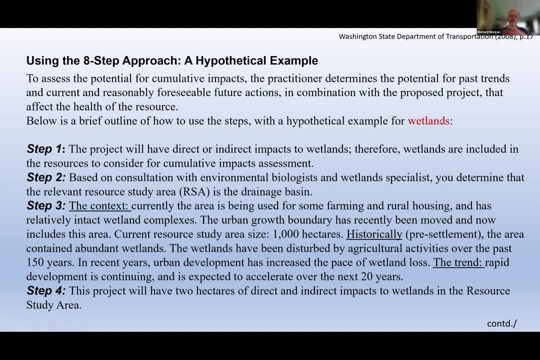 So I've made wetlands in red there. That's our key resource. So step one project will have direct or indirect impacts on the wetlands. Therefore, wetlands are included in the resources to consider in our CIA. There might be other resources. 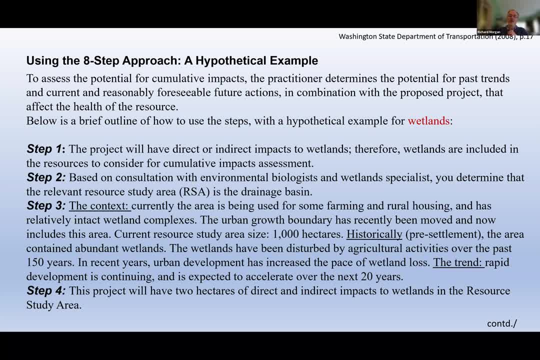 There might be the regional community- you know people and other things- But in this case we're focusing just on the wetlands as a key part of our cumulative assessment. We talk to knowledgeable people, define the study area. In this case they decided the drainage basin as a whole would be the unit to look at. 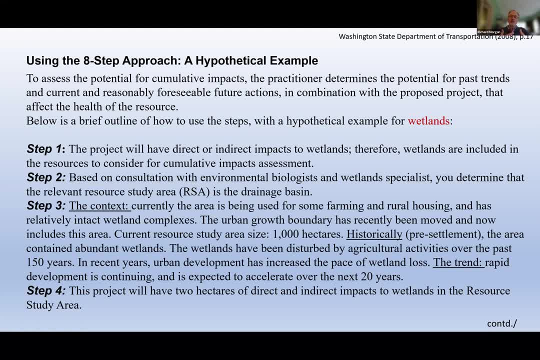 And then we look at the existing context, Existing land use around it, The historical context, As they say, pre-settlement- This was taken from the US- And then the impact of settlement and agriculture and urban development and so on, And from that identify the trends, the changes that are taking place in this wetland area. 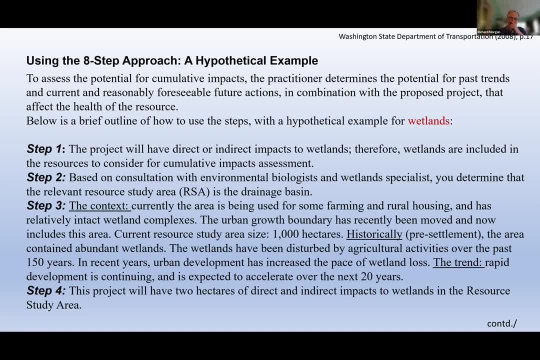 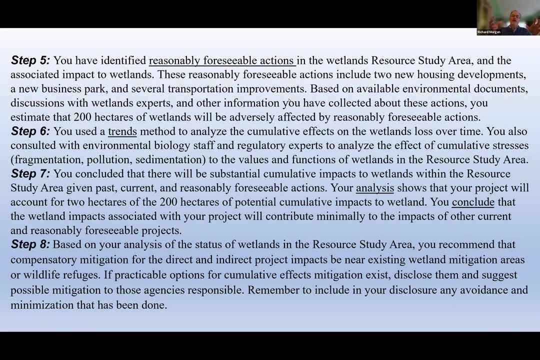 And what's likely to happen in the future. And then we say, well, our project is going to look like this. This project is going to affect only a small bit, two hectares, directly, indirectly, in this wetland area. So we've assessed our footprint, if you like, from our project. 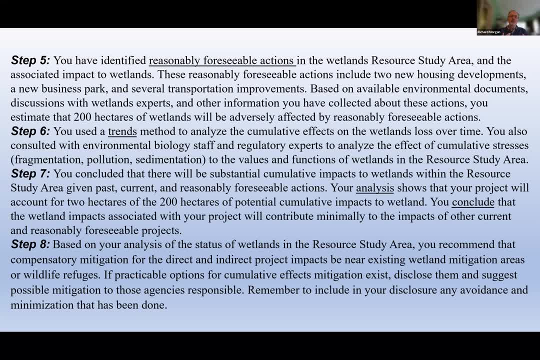 What about the future of this wetland? Reasonably foreseeable actions- We look at what those might be, Talking to the local planners and developers And identify that And try and get a handle on what that might mean for changes And we find that that could affect about 200 hectares of the wetlands from foreseeable actions. 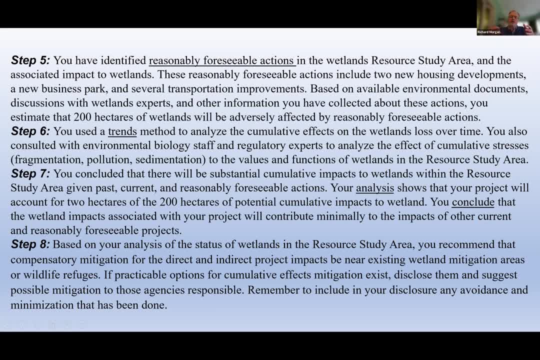 And so we start pulling this together and say, okay, we've got the trends of change over time. The climate's drying, So the wetland's going to be shrinking. We've got this development that might affect 200 hectares, So we can start getting a sense of what all of the cumulative impacts might be. 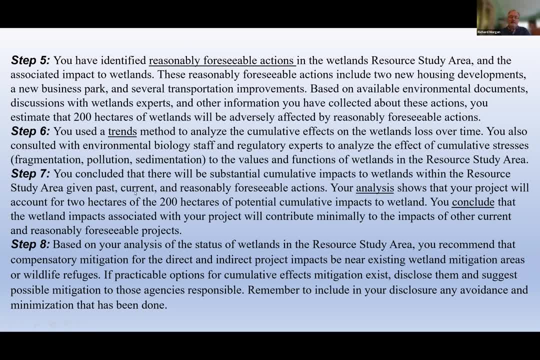 Gains and losses over the next 20, 30 years. And we put our project into that context and say we're only going to affect two hectares, So it's not that much compared to all the damage everything else is doing. So maybe our project could go ahead if we can mitigate those two hectares. 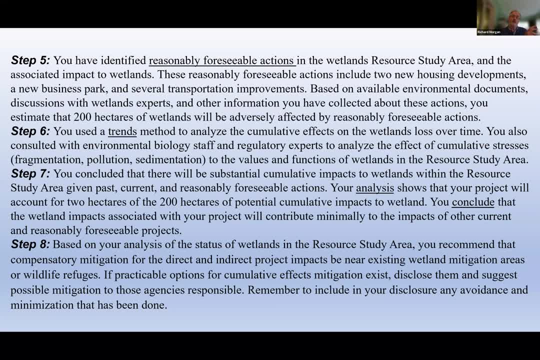 Perhaps restore some wetland elsewhere, Maybe six hectares we can set up somewhere else to offset what we're doing through our project. And so we go ahead and we devise our mitigation and all of those things, Write it all up And take it to the decision makers and hope that they say: yep, go ahead, because you've done a brilliant job. 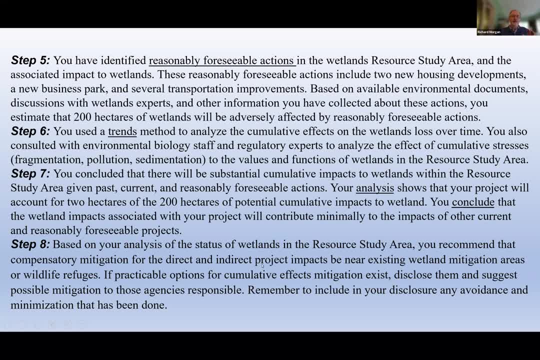 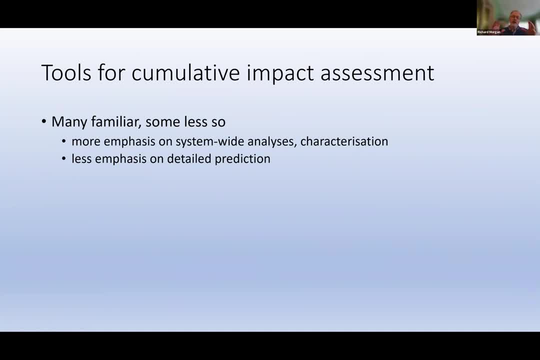 Or not. You know what regulators are like. So there is a way of approaching it. It's based on impact assessment And it's quite a common sense way of doing it, But it does require us to shift our thinking a little bit from the confines of the project to embrace a much bigger area. 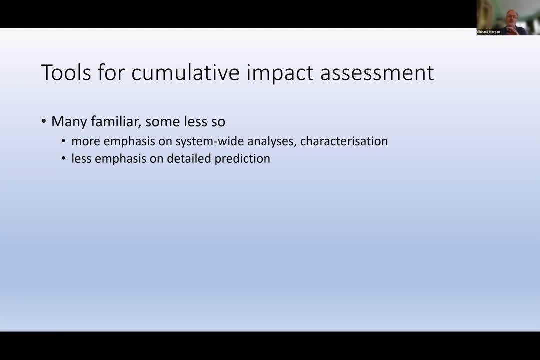 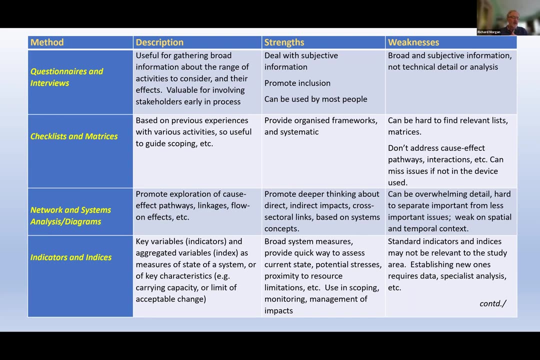 And therefore more challenging in terms of the tools and techniques that we use, Because we have to think about system-wide, area-wide perspectives. Now again, this is a resource I think I've taken from the Canadian- I'm not quite sure- IFC. 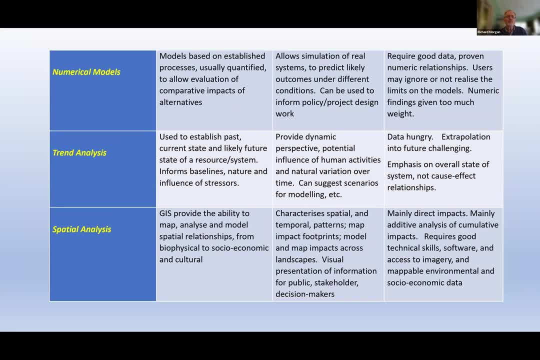 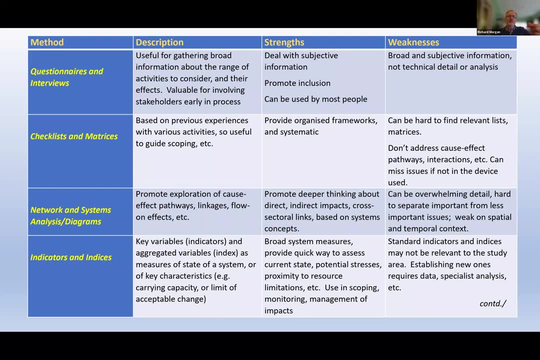 It's on the next page. Let me just no, I haven't put it. Anyway, again, I'm not going to go through it in detail, I'm going to just pull out one or two points here. Down the left-hand side are some of the methods that are used. 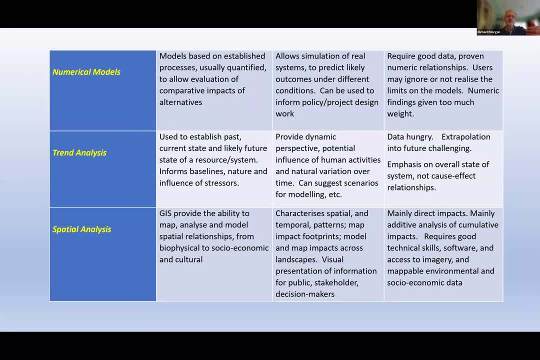 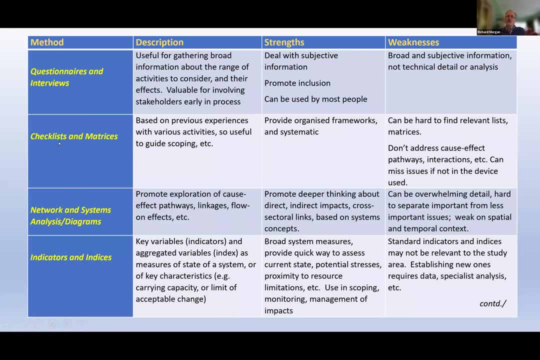 And it's a two-page diagram From very simple Questionnaires and interviews. And then you'll see checklists and matrices Beloved of impact assessors, or at least the textbooks everywhere, Then networks and systems diagrams. Again. that's, you know, classic textbook stuff. 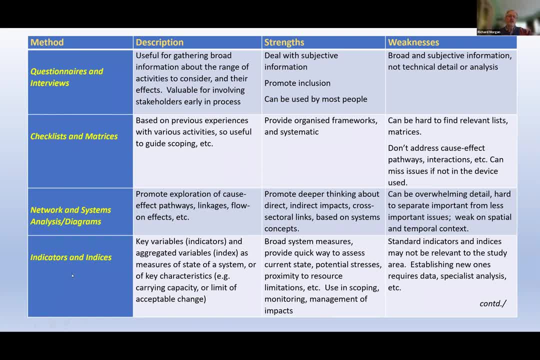 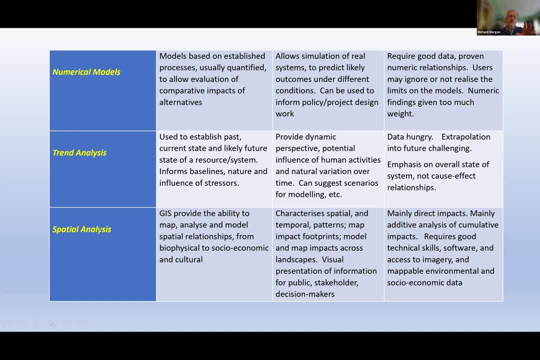 But then things like indicators and indices, Models, trend analysis and then spatial analysis. Now, impact assessment, we're familiar with using models, We're familiar with using GIS, Trend analysis perhaps a little different. Use of indicators is a little different. 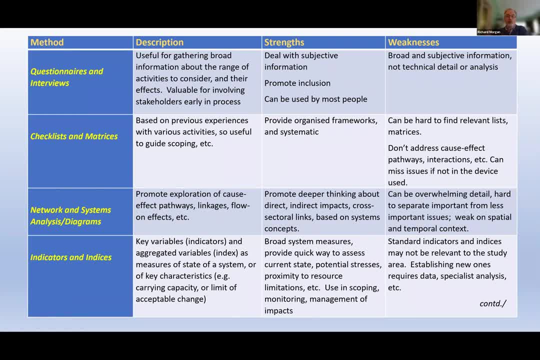 Questionnaires and interviews might be used in social impact assessment, But here we're using it as a wider tool for cumulative assessment. And it's really saying: the first thing to do is open up, talking to people, Not just specialists, But local communities, stakeholders and so on. 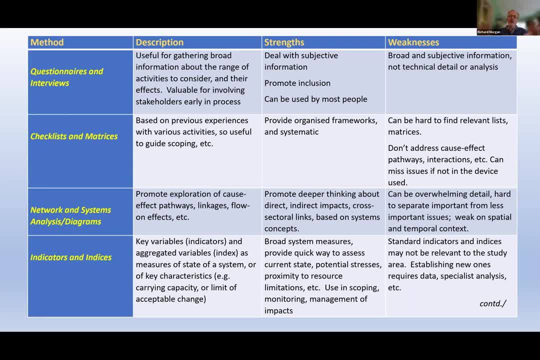 So that we can start Identifying existing activities: Historical knowledge, Traditional knowledge, All of which is going to come into Our eight step approach, Providing context, Providing historical context, And so on and so forth. So talking to people is important. 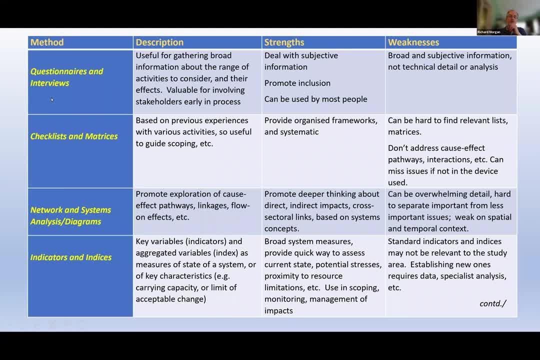 Hence There's quite a lot of emphasis on Using the tools, And then we might use things like checklists and matrices to help us Think through some of the Activities and the sort of typical impacts they might have on The environment. 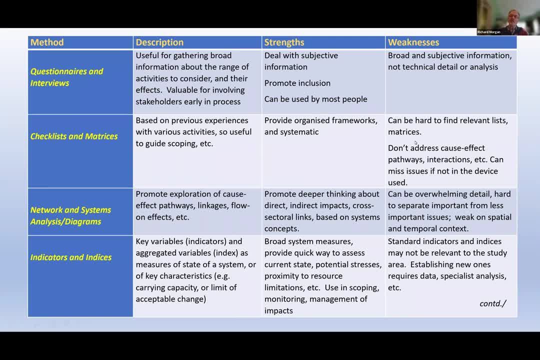 Strengths and weaknesses. So, with weaknesses, Things like checklists and matrices And not very good on Cause effect pathways, So we rely on Systems And so on, And then we might use Things like Statistical data analysis tools. 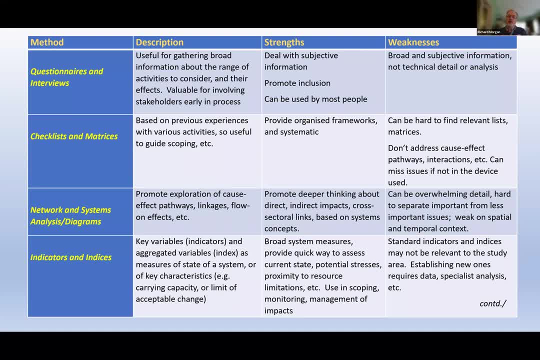 And such like To really help us with that. But early on, As with all impact assessment, these tools help us just structure our thinking And, as we, if we need to be more complicated, A deeper analysis, Then we use those extra tools. 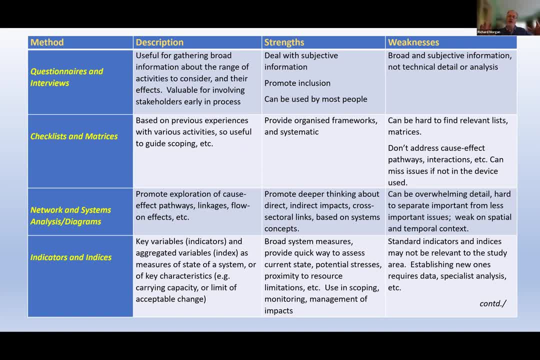 Indicators and indices Suggested as one way of Trying to capture across a whole system. So if you can imagine if you're looking at a drainage basin with a big wetland in it, we don't want to be counting all the individual species of plants, insects, aquatic. 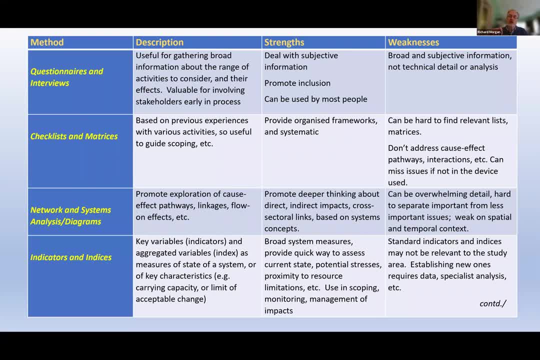 fauna and so on. We want some indicators of the health of that system. So it might be that we use biological oxygen demand and we use some sort of species index, a compound index of the presence of key species either in the. I'm trying to dredge up my ecological knowledge. I'm 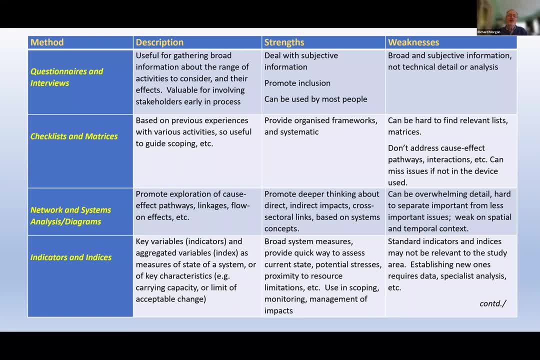 an ecologist, This is dreadful. Maybe we're looking at the key predators, some of the keystone species, or we look at some of the key plants In a wetland system that are required to maintain its structure and resilience, So we don't have to. 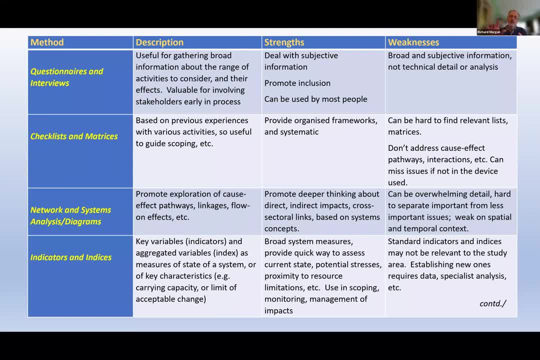 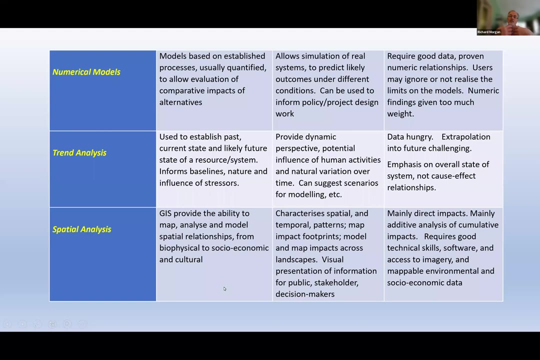 measure everything. We want to find key indicators that give us a big picture view that we can then monitor in future to ensure that we're maintaining the health of the system. That's more important with cumulative impacts than usually with project level impact assessment, Our numerical models. we're used to that with things like air pollution from a chimney trying to. 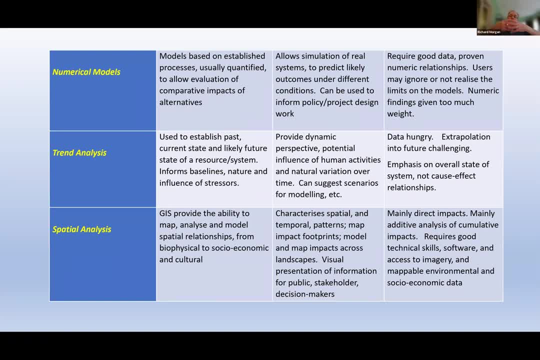 model how it's going to affect a local area. Now we've got to do that across big area, area wide. So we hand all of that over to the techies. let them get on with it. The same with trend analysis. the same. 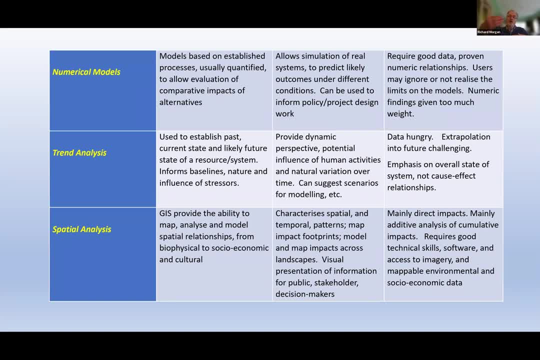 with spatial analysis, GIS, As we now onto these more complex things. they all require more information, more data, And so there's a, Again, a tension between trying to do a decent job without getting into too much expense of gathering too much data. And that's where remote sensing becomes really important, And especially with spatial 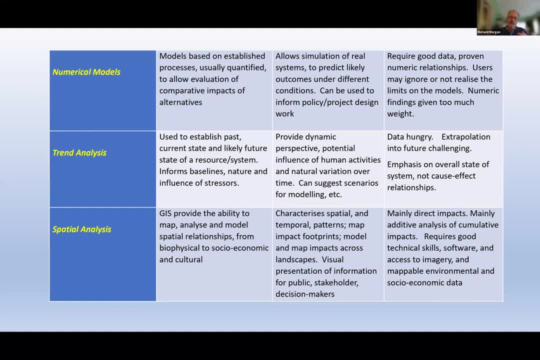 analysis. Now, sadly, as the Ukraine conflict shows, there's a lot of sensors up there that we can go to for imagery and start using in this sort of analysis. Other data may be more expensive to get, but we can do quite a lot with what's available. 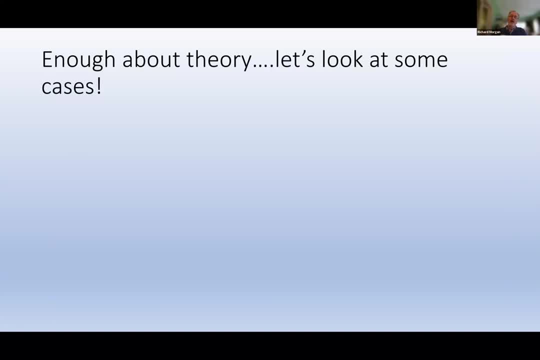 Okay, that's the theory. I've gone through it quite quick And I keep saying: go back and look at some of those points in detail, go to some of the guidance documents, But now I'm going to. I was going to say I'm going to. 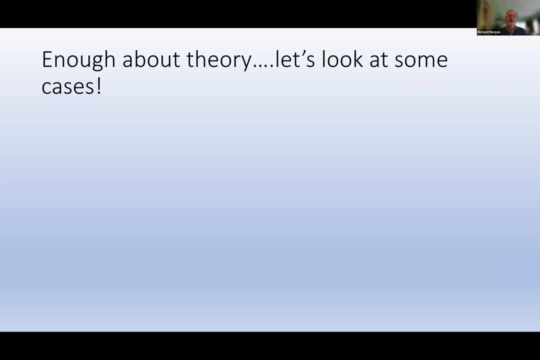 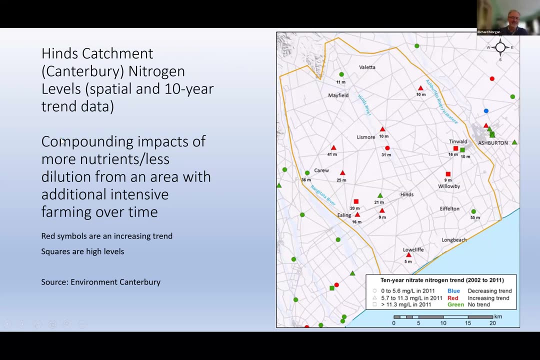 take a snooze, but I can't because I've got to keep flicking the slides through And I'm going to pass over to Nick who's going to come on off mute before he starts talking. Very funny, Okay, hi, everybody. Kia ora tātou or kia ora ana, as I'll return to the Cook Islands later in my examples. 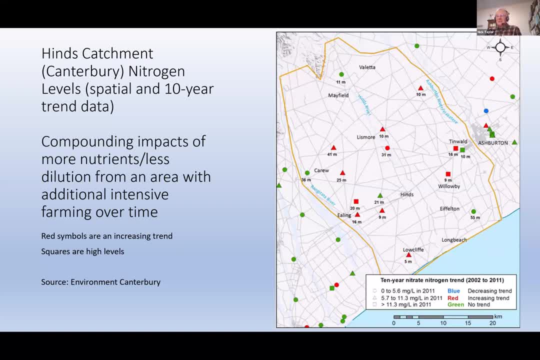 hopefully opening up for some discussion. So what I'd like to do is just add to what Richard has been saying by giving you some illustrations. There's going to be a couple from New Zealand and then a couple from the Pacific Islands, And what I hope to do is kind of connect back to this theory and the context that Richard has been setting up with his examples and his methods, but also to hopefully get you to get involved in this as well. So maybe at some point you'll start liking to. 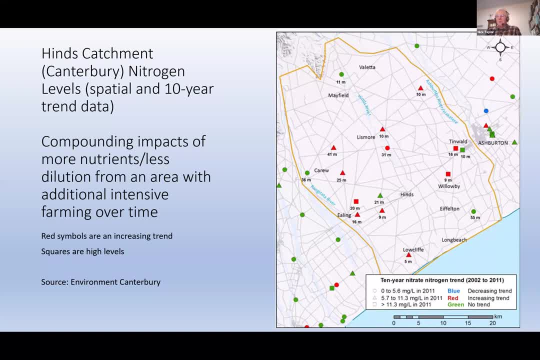 put in some questions and we'll address them as we can later on Now. my examples also include in them ways in which we could think about responding to cumulative assessments. So I don't want to just talk about what they look like, these cumulative effects, but also some of the methods we actually have within environmental impact assessment as a whole. 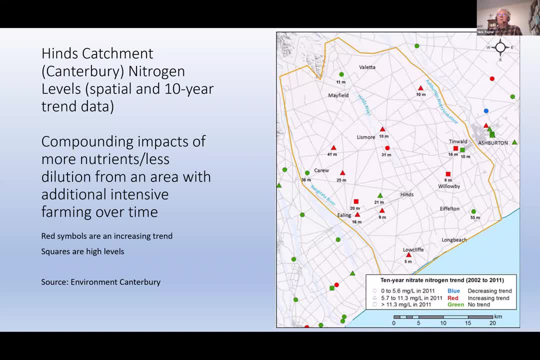 for dealing with them And in that sense I will talk about both project level assessments and also strategic assessments. I'm assuming you will you're all familiar with. the notion of strategic assessments is being more focused on policies and plans, And certainly that's where this first example fits. So 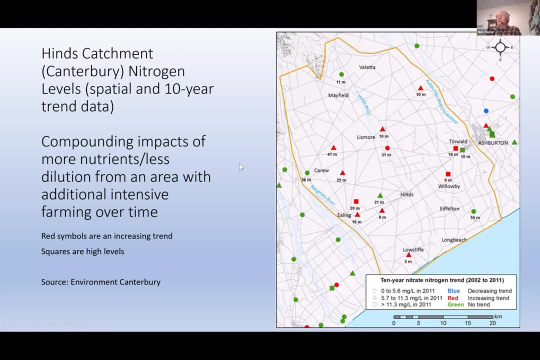 on the surface. you'll see a map here of a catchment and the catchment is in Canterbury, So that's all you have to worry about at the moment. You can see it's a catchment between two rivers: the Ashburton River- if any of you know Canterbury- and the Rangitata River to the south. 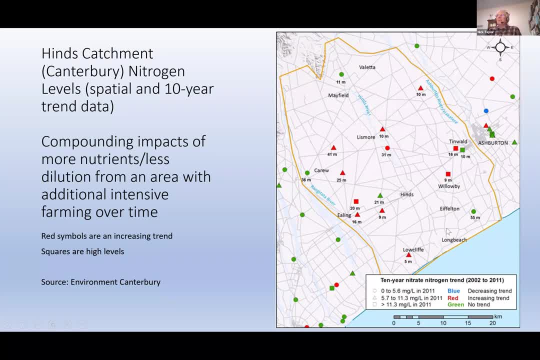 Richard has control over his cursor, so he may be doing some pointing as we go around here. So what have we got here? Well, we've got this catchment that's surrounded by that yellow line, and the catchment is one in which, over the last 10 to 15 years, there's been considerable intensification of agriculture based on irrigation. 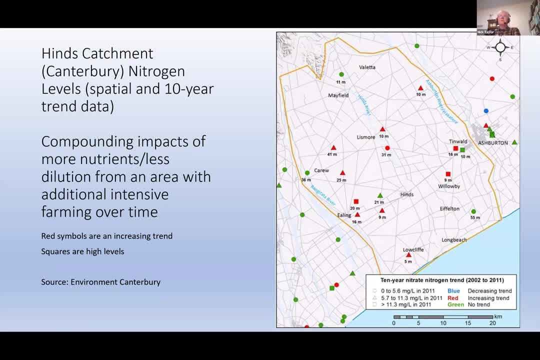 And this irrigated agriculture has, by and large, seen, in particular dairy farming, which wasn't present in the catchment in any region, To an extent really previously expanded in this area and at the same time there's been increasing interest and concern about the levels of nitrogen in waterways. 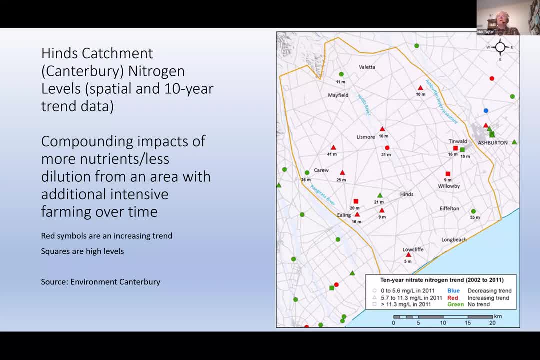 So this map is just simply showing you some data which is both spatial, so at a catchment level, but also trend data. So in these little symbols on the map that you can see, the little red and green symbols you can see- reflected some trend data which is the increase in or decrease, but largely it's all increase in the levels of nitrogen discovered in test wells. 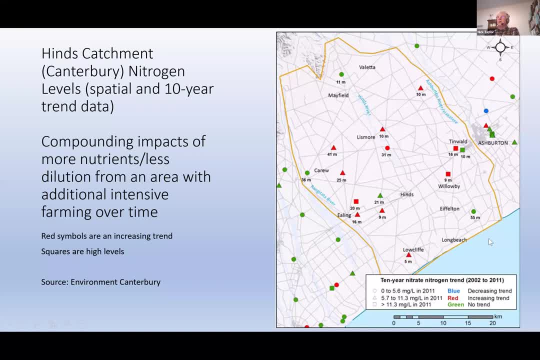 So these are wells where sampling's being taken for nitrogen levels and tested and measured, And what it shows is that over a 10 year period- the measurement was going on- that there was a real increase in the level of nitrogen in these waterways. 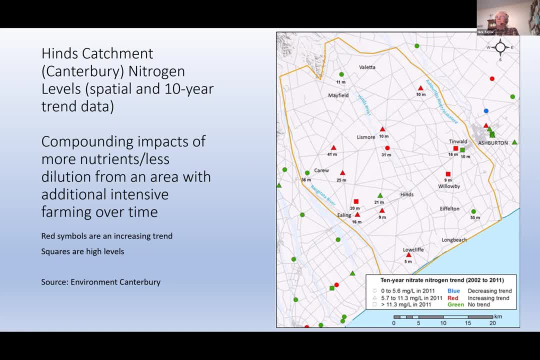 So this was a catchment we were doing some strategic assessment of for land and water planning and therefore this information was really interesting Because of course it's from a compounding effect from a number of farms. It's not just one farm, there are a whole lot of farms that are converting, have been converting, to dairy farming. 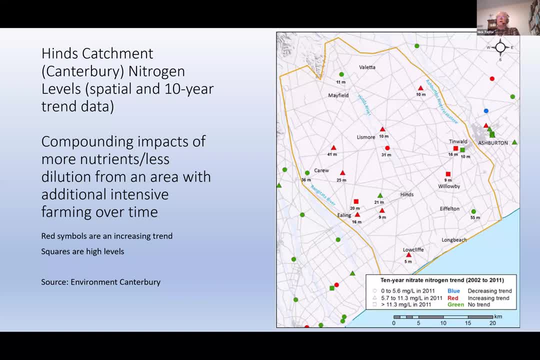 And therefore adding each of them to the compounding impact of more nutrients in the waterways and at the same time- and it gets complicated, so I won't go into all of the detail, but basically you've got less water in surface water and also in groundwater due to 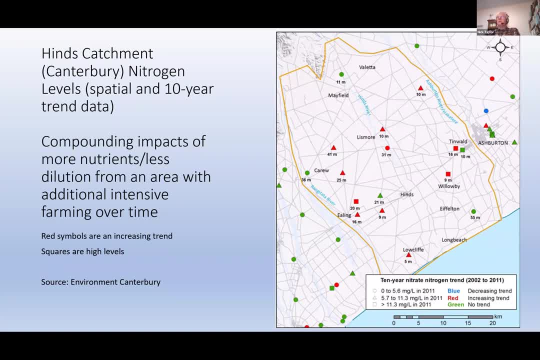 extractions from the system for irrigation. most of the irrigation water comes from the river to the south, the Rangitata river, and is conveyed out to all the farms in the area. so this is an interesting kind of cumulative effect, very much recognized as a cumulative effect for what was 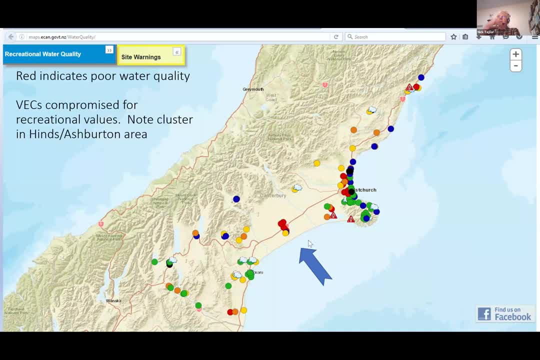 happening. next slide: Richard. Richard, have you gone to sleep? no, you're up, and so here is a wider shot of Canterbury, and this is interesting because it shows water quality for recreational purposes, basically for contact recreation. so this is based largely on pathogens in the water and also as a result of nitrogen in 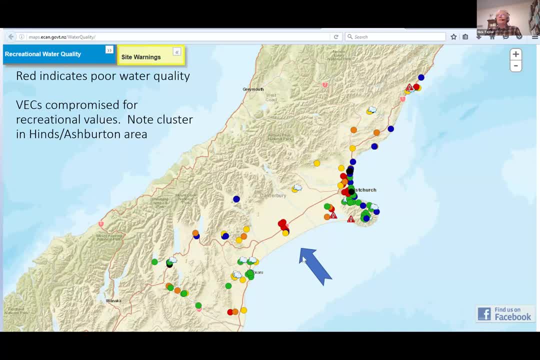 water that is creating, or nutrients in the water that's creating, growths of phytoplankton or unpleasant species in the waterway, with algal blooms and so forth. so these are detracting from the valued environmental conditions. so this is a very interesting component in this case, which is the recreational value, and 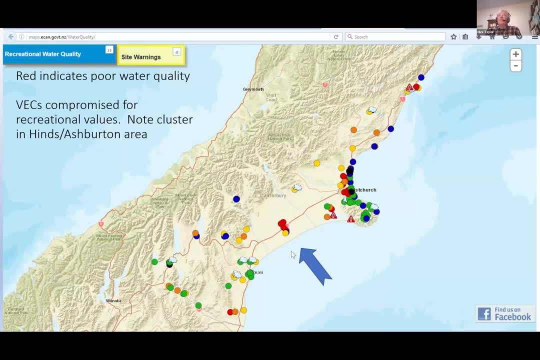 particularly the swim ability of these waterways, and you can see where the arrow is pointing right in the middle of the map. it's not the only area, but it's one of the areas, which is the Ashburton Hines area that I'm talking about, where there has been a considerable increase in this, these red 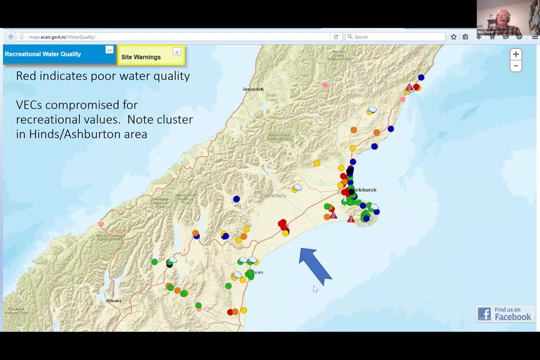 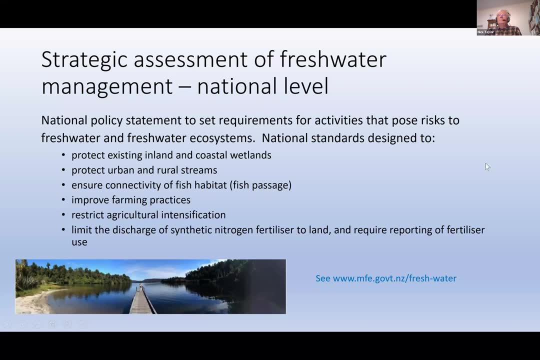 dots, which are the ones which are very poor water quality for swimming. next slide, please, Richard. so what are we doing about it? well, this decline in quality of water is a problem, and fresh water is a problem throughout the country. this is not just in Canterbury. it's particularly highlighted in Canterbury. it's a big issue in the 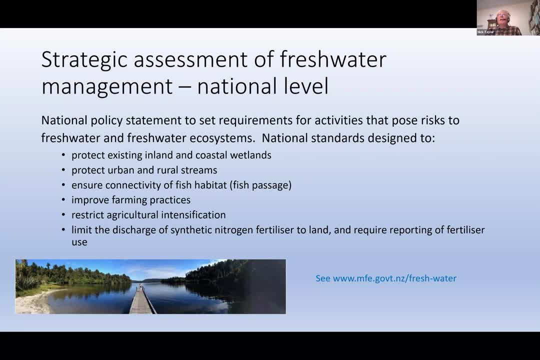 Waikato, in Southland, really anywhere where there's dairy farming or intensive agriculture. so the government a few years ago, over time has set out to develop some national policy statements about fresh water management and the current national policy statement has actually moved to the level of 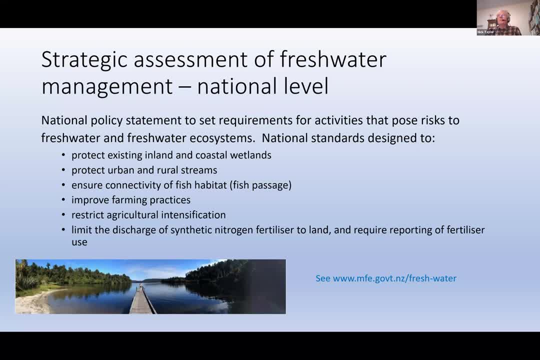 setting national standards, national environmental standards, and these standards are designed to protect existing land in land and coastal wetlands, urban and rural streams, fish habitats and so forth. but they also set rules that are in intended to improve farming practices through farm management plans, farm environmental management, 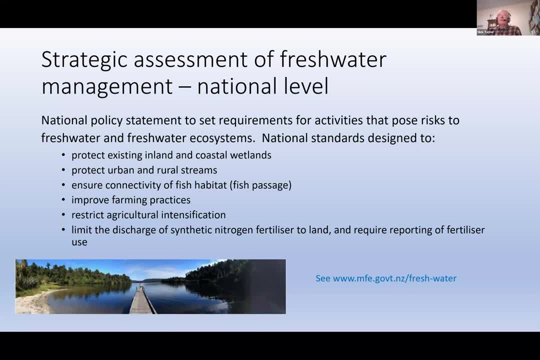 plans and to actually at the broadest level also to restrict agricultural intensification in some situations and certainly to limit the discharge of nitrogen fertilizer to land. Now you can see this in the website of the Ministry for the Environment, where there's quite a lot about the 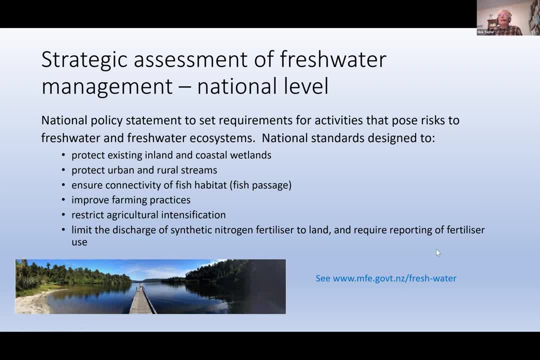 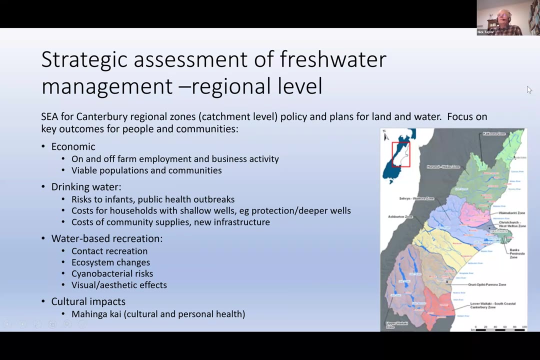 whole national policy statement and national standards on freshwater management. but basically, all I wanted to point out was that the problem that existed at the catchment level was actually is actually being addressed at the national level. It's also being very much addressed at the regional level. so that's the next slide. Richard, And that was being done by on the right hand side, you can. 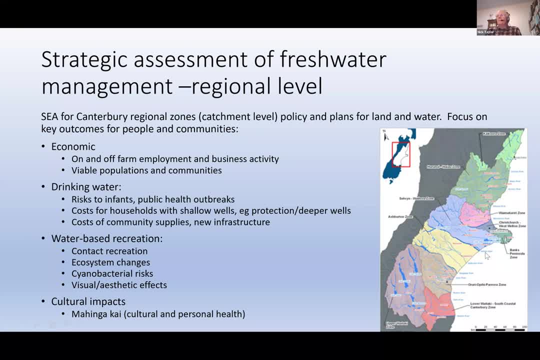 see a map of Canterbury and it's divided into some colour And these were zones which are largely catchments or sub-catchments in the, in the region And at the regional level. the regional council, or ECAN as we call it, was responsible for setting limits on the. 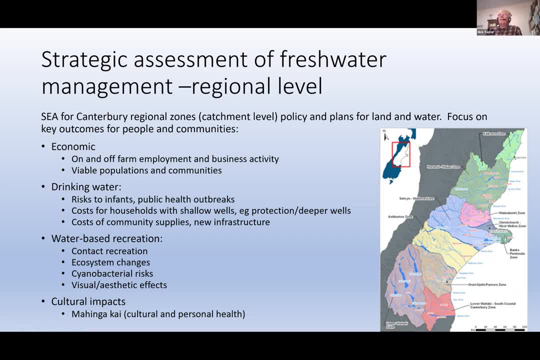 use of water, the amount of water you can extract and also what you can discharge into the water, And this is done through land and water planning. So these are strategic. these are plans being developed at the regional level where SEA was specifically applied and looked at the ecological impacts, the groundwater impacts. 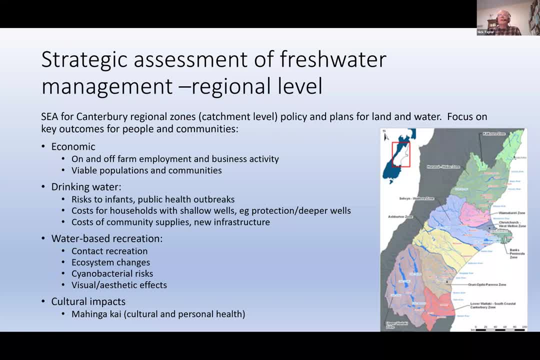 a lot of modelling- Richard mentioned quantitative modelling before- a lot of modelling of water, groundwater, nutrients, where they're all going, what's happening to them and so forth, And this was actually taken out and the parts that I and my team were working on in particular was: 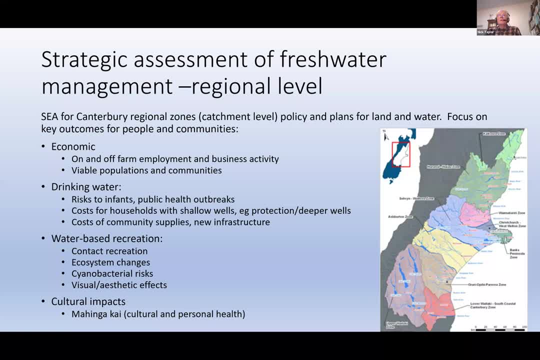 looking at the outcomes for people and communities And this was looking at balancing the economic benefits of on and off farm employment and business activity and the viability of rural populations and communities in particular, which obviously farming contributes to, balancing that with the other effects that were happening, which were impacts on drinking water, where there were. 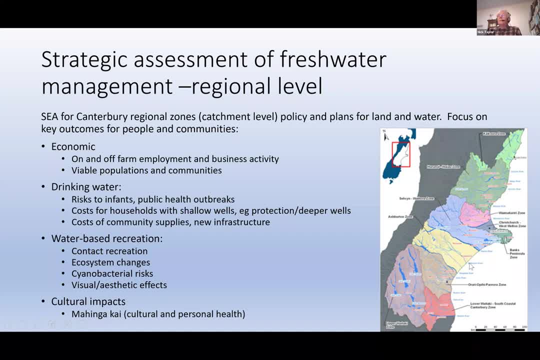 risks to, particularly from to infants, from drinking too much water with nitrogen in it, public health, outbreaks of pathogens and water which were causing problems in some communities, costs for households who are having to deepen their wells to get to better, cleaner water. as the water infiltrates down, So deeper you go. 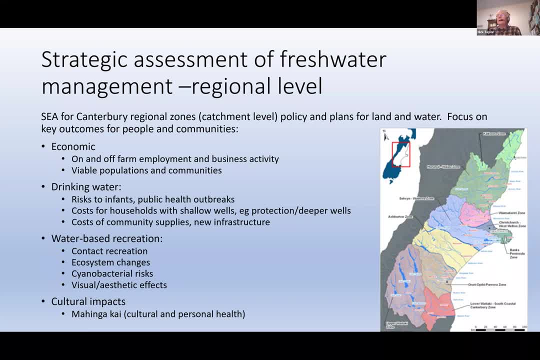 tends to be the cleaner it is, and the cost of community supplies and new infrastructure. So communities also are having to dig deeper wells and councils are having to put in investment in new infrastructure. And then we looked as well at water-based recreation and the impacts that were happening there, as well as cultural impacts, particularly for mahinga kai, or the cultural and personal uses of food supplies and so forth, collecting of particularly some species for cultural purposes. 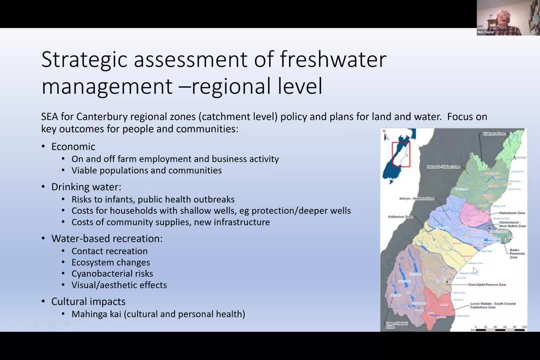 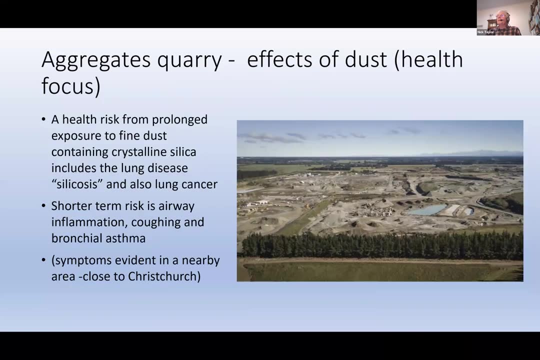 So all of this was bound up in the strategic level assessment to try and address the problem of these accumulating or cumulative effects from many distributed activities in the catchments. So, Richard, I'll move on to the next example, please. So, just to be totally different, instead of looking at nice, pleasant green farmland, let's look at some big holes in the ground. 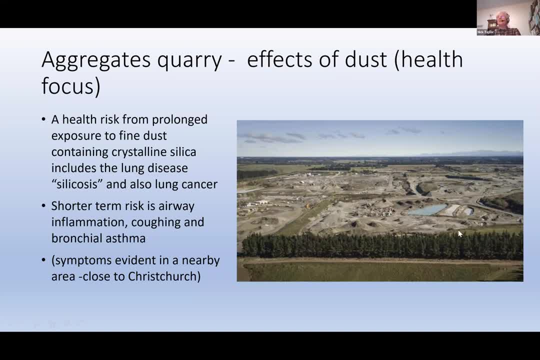 And if you're flying into Christchurch, these are the big aggregate quarries that you'll see out of the side of the plane. So it's actually quite close to the city of Christchurch And in the earthquake recovery period a lot of shingle was needed for urban development, subdivisions and so forth where new housing was going. 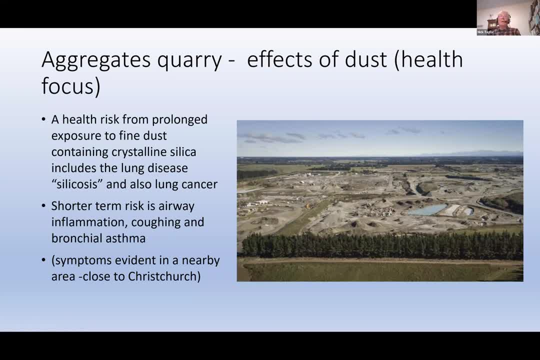 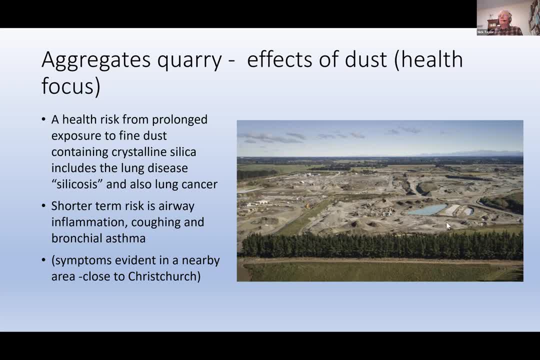 Aggregate mining. Aggregate mining: This was actually done by individual operators. So these holes you're looking at here, which is out at Yalthurst near Christchurch, are actually a series of privately owned quarries And each quarry has tended over time. each quarry operator has tended over time to acquire more land and go further out. 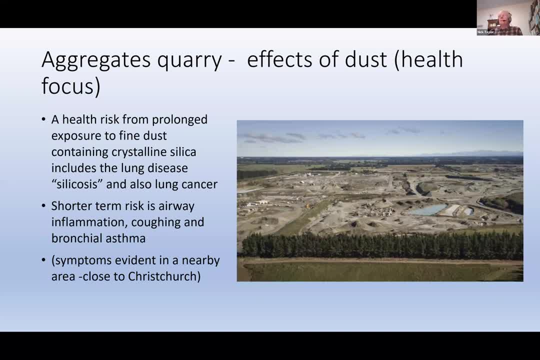 And basically, as they push out these quarries, they're pushing into land where people have acquired. And basically, as they push out these quarries, they're pushing into land where people have acquired lifestyle farming properties, So small farms where they're living for lifestyle reasons. 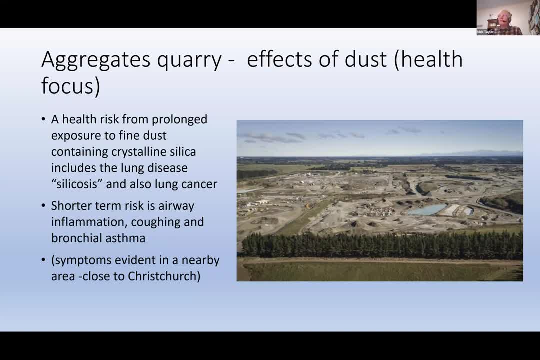 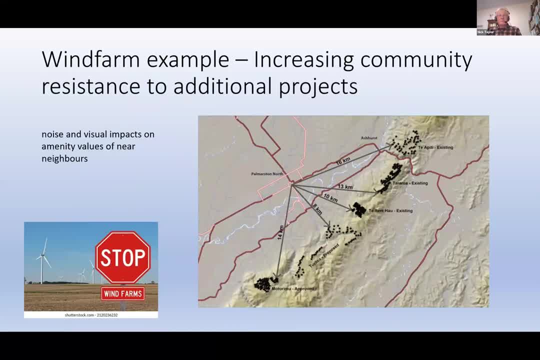 And these quarries have been very clearly shown to have a health risk from prolonged exposure to fine dust which contains silicosis. Next slide, please. I just threw this in as a- kind of an additional thought. I just threw this in as a kind of an additional thought. 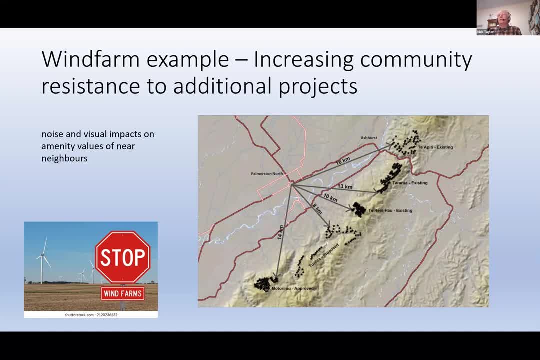 What actually happened with the quarry case is someone came up with the idea of another quarry at an additional site not far away again from that one I was talking about, And that there was a real resistance from the community. There were demonstrations, People with placards. 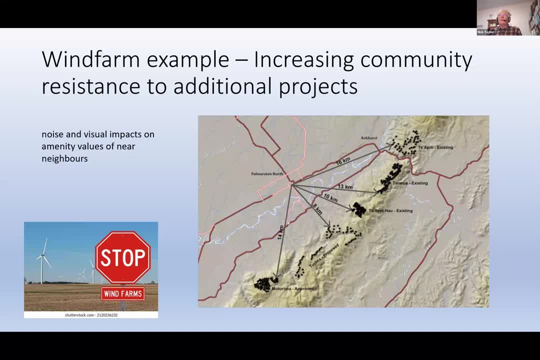 saying: stop the quarry, stop the quarry. a lot of stuff in the, in the newspaper and the media. they didn't want the quarry. and what's interesting here? this is a picture of um, just some wind farms on the big picture on the. on the right the map, um is wind farms on the tararoa ranges which you, if 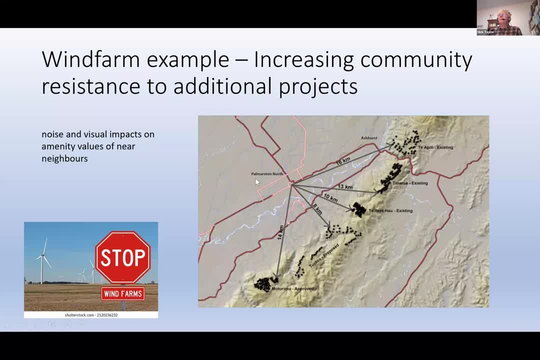 you're familiar with them if you've ever been to massey university. um are the range which are above palmston north and the north island. so this is the range of hills that sit along to the south east of palmston north city, and these are very windy ranges. they're the best wind sources in the 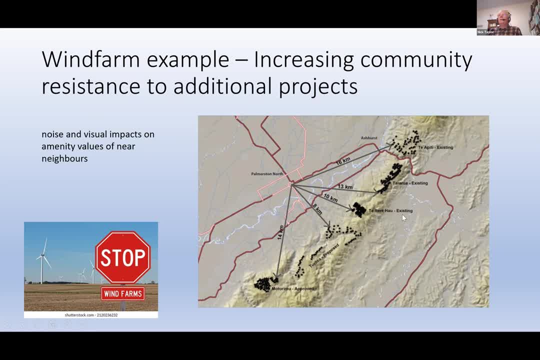 world for generating wind power, and what happened is- you can see, the black dots are wind pylons and over time, a number of different developments have gone in along this range, and there was a another one proposed, which was in the towards the bottom, the turritea proposal. 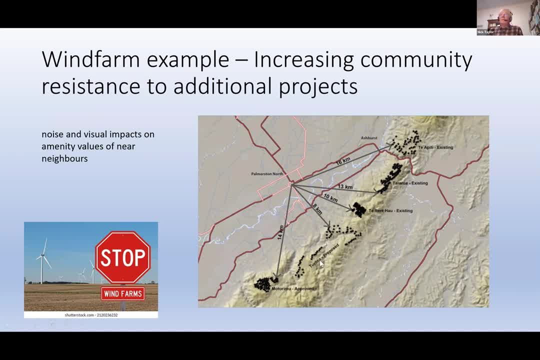 um, it's just just there, richard. yep, that one um which was being proposed, and um, there was a real concern from the people of the area to say what we've had enough. we've we've had enough wind farms, and we actually did some research on the impact of these wind. 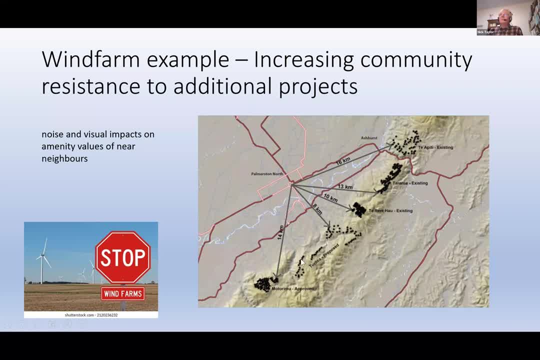 farms on the local residents and we found that there was a definite effect. within probably two kilometers of a windmill, people were having an impact on their amenity values. just as i discussed for the quarries, the same thing was happening here. not dust in this case, but noise and landscape change and there was increasing community. 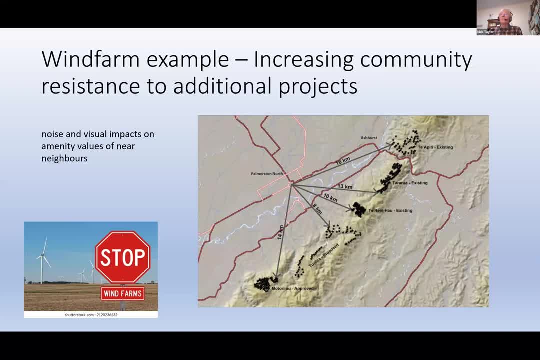 resistance. so we did a survey of residents of palmston north and found that, whilst in the beginning they were very, very supportive of wind farms because of the fact that they produced energy, by the time they had all these additional wind farms along the hills there was actually. 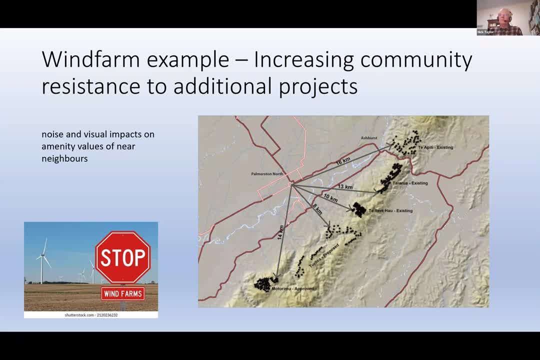 quite a concern that enough is enough. we've got enough windmills, let's put the rest somewhere else. and you're seeing this around the world, actually a resistance to green energy, because people are saying, ah, um, we've had enough. so i just sort of i think you're getting a situation now, just like 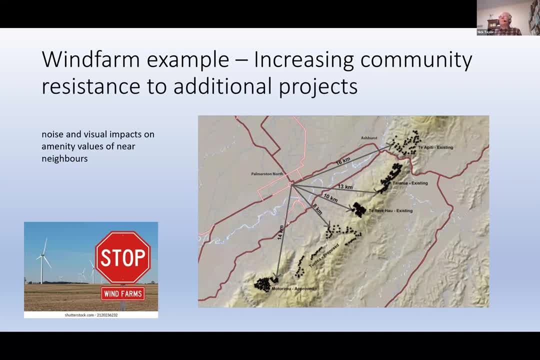 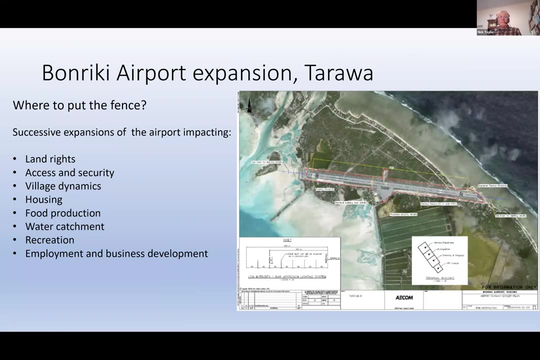 with the quarries where there's increasing community resistance to some proposals, because people are saying, well, we've had enough of this, change, okay, next slide. let's go to a pacific island example. i don't know how many people we've got from um kiribati here online. we maybe have a few um. so this is bonariki airport in tarawa. 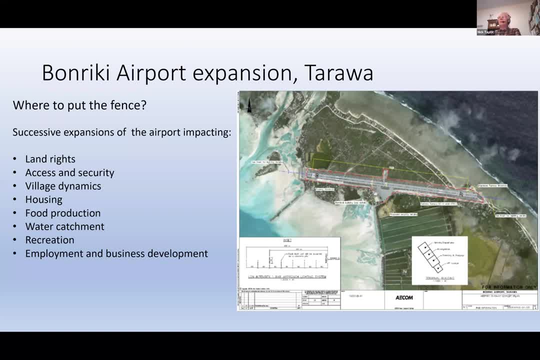 i thought this was an interesting example because, um, you can see the airport in this aerial shot laying across the atoll there, and this is an example where you have a piece of infrastructure, in this instance an airport. the same could be applied to a port, and very typical. 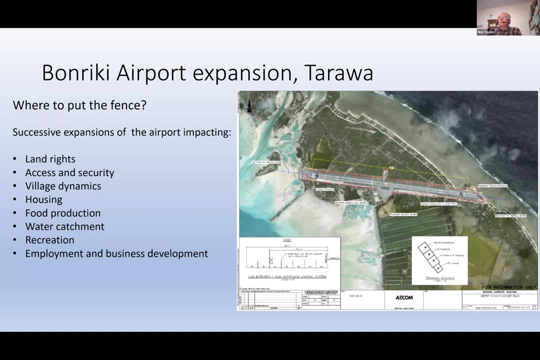 of these sorts of facilities: airports and ports. also a lot of urban facilities, where the facility starts growing over time, keep adding to it. so port expansion, airport expansion, is very, very typical around the world. so this is a really good example of infrastructure that is growing and when you start increasing, 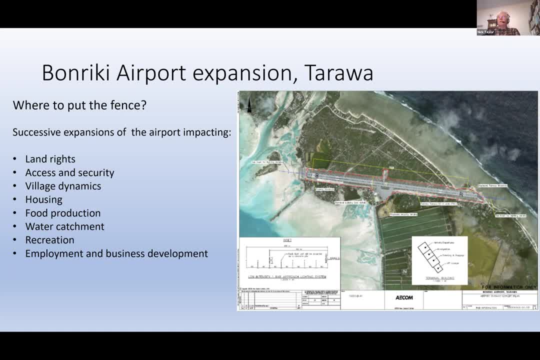 even at one site you have the same issue of cumulative effects. so it's not like from multiple sites, but it's from expanding on one site, and in this instance the airport has been expanded back from the second world war. it's been expanded for over one year and it has taken a series of developments over time. 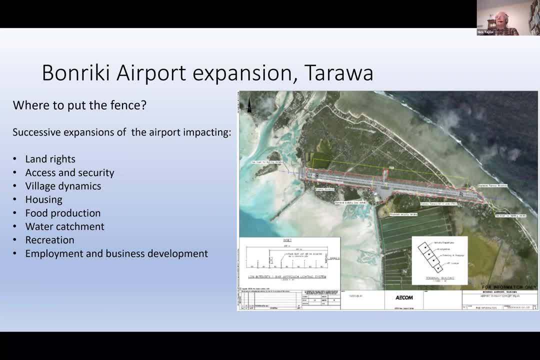 taking up additional land and pushing out to the sides. and most recently in recent years, there was a proposal to redevelop the airport to particularly to reseal the runway but also to install a security fence around the runway. now, if you'd have stepped back and said, well, 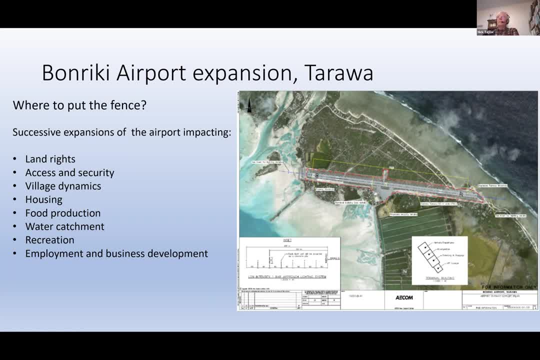 what have these successive expansions of the airport done? over time had an impact in a number of ways on local people, particularly around land rights, people having land taken in effect for airport expansion, and there were all underlying issues of royalties and whether royalties had been paid, should have been paid and typical of customary land. 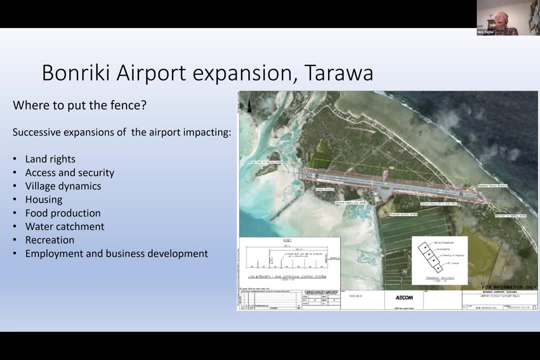 whose land was it anyway? who had the rights to the royalties, etc. so there was a certain level of grievance around land rights that was underlying this airport. there were increasing issues around access and security, which have been particularly being brought to light in the jet jet aircraft era, where jet pilots are not too keen on seeing vehicles on the runway or people. 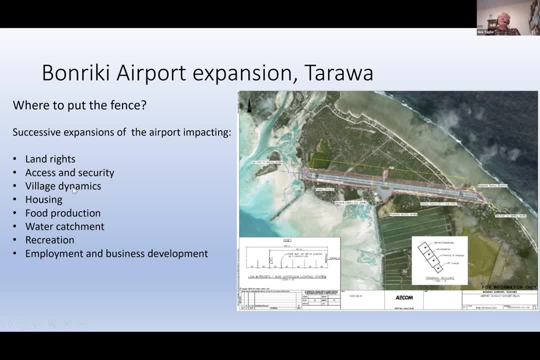 or animals on the runway when they come in to land a jet. so there are increasing issues around land rights, including previous attempts to put a fence around this runway, and there's also an impact on village dynamics because people walk across and drive. they drive around the ends of the runway, but they actually drive across the runway when there's no planes around and or 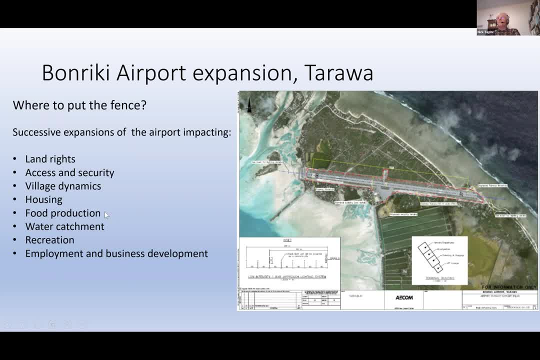 walk across the runway and you can see in the picture the tracks that they've made as a result of that um, and if, in effect, people are living on one side of the up the northern part of the north side of the runway, and actually they're attending um church and schools, for instance on 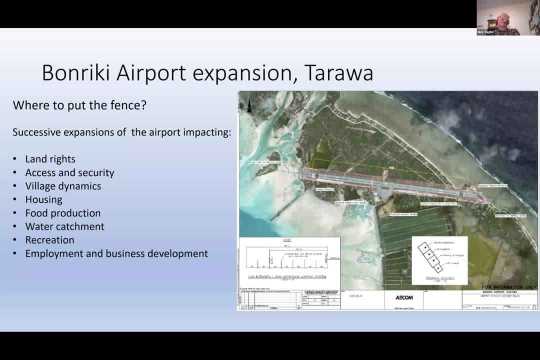 the other side of the runway, in the main bonriki village, which is to the south of the runway there. so, um, that is a, that is a um, an issue in rounds, village dynamics, housing. increasingly, as the runway expands, it reduces the land available for housing and for expansion of 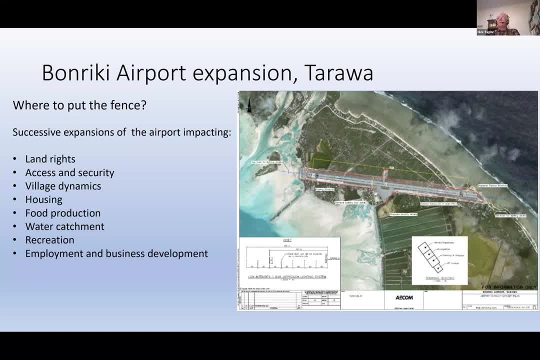 the village for housing and also for food production. so the wider the runway gets, the more you've got to take out to create safety areas and the more particularly food producing trees and um cultivation areas are reduced. so food production is affected. the water catchment is affected. so to the north of the runway is the main as a principal water catchment lens on tarawa. 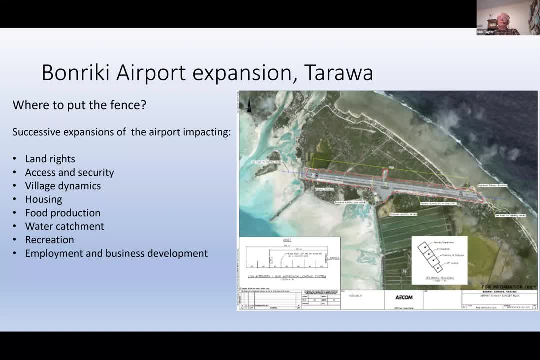 so it's a really important site for collecting water, recreation um. interestingly, because the Because there was open space around the airport runway, people went out there to play soccer, for instance, football on land on one side of the runway. And also, of course, there's employment and business opportunities. 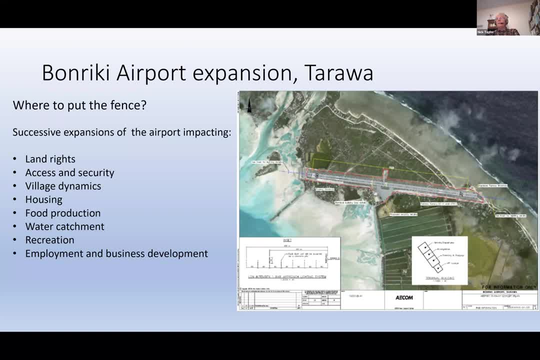 So as the runway and the airport expands over time, like any airport, it's creating opportunities for business for people servicing visitors, for transport firms, taxis and so forth Logistics companies. they can start positioning around a runway like this, So there's employment and business opportunities created from expanding the airport. 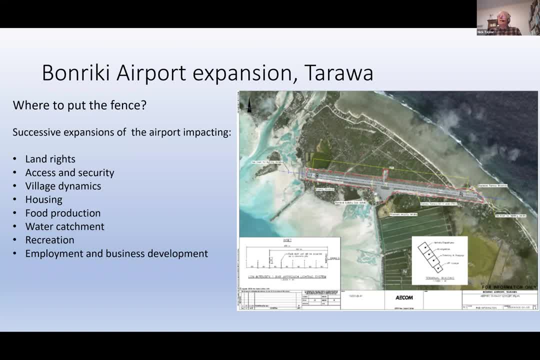 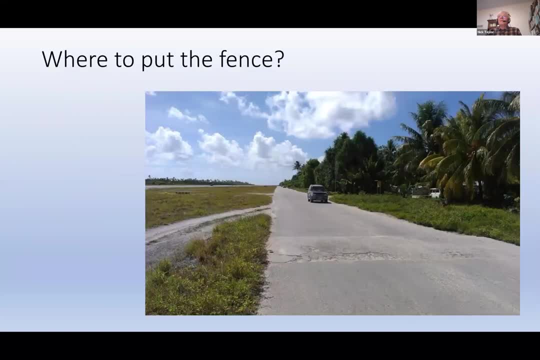 So these are successive changes that happened over time, But the big issue was the fence. Where would the fence go Next? slide, please, Richard. So this is the road on the side of the runway, with the main Bonriki village on your right. 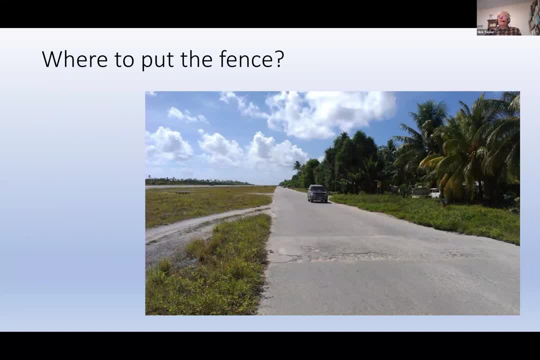 And you can see here. this is how people use this road around the edge of the runway. They also use the runway itself for driving up and down. So the question was: well, the airport people wanted to put the fence on the right-hand side of that road. 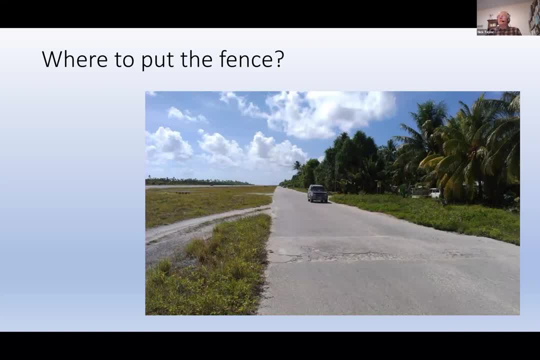 They wanted the fence in fact to go into the trees and into the village It was. the original plan was to build the fence and take land that actually went in and in fact would have taken up Some of the housing. Now, some of that housing was informal housing. 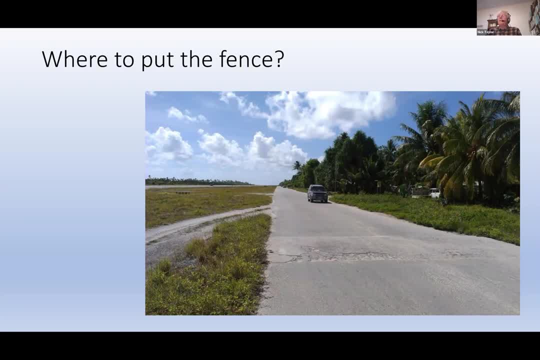 The additional living units that have been built on people's land- relatives and so forth- moving into Tarawa. So there's housing as well as food trees, as you can see along that edge of the runway, which would have been taken up by the fence. 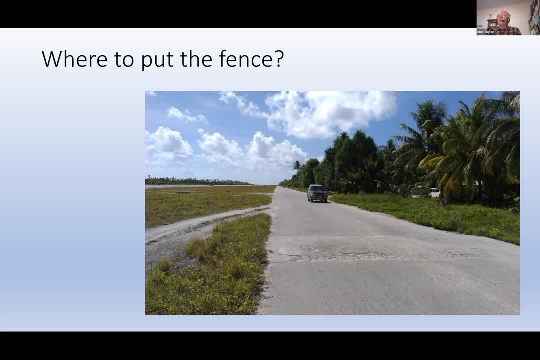 But also it would have had a much more effect on access in and around the airport If you put the fence on the other side Of the road. So after a lot of discussion between the engineers and the aviation security authorities and authorities, they actually decided to put the fence on the left-hand side of that road rather than the right-hand side, which actually made a lot of sense. 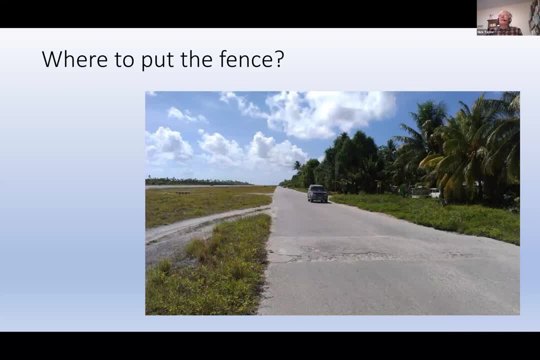 So this was an interesting, I guess, response to some of the cumulative effects was to say, well, we can actually adjust the design Of this airport so that it doesn't keep pushing into the land, and the villages on either side of it would still have an effect on access, for instance, and they had to develop some mitigation strategies to deal with that. 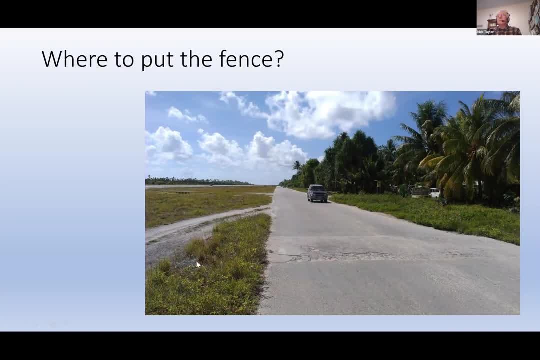 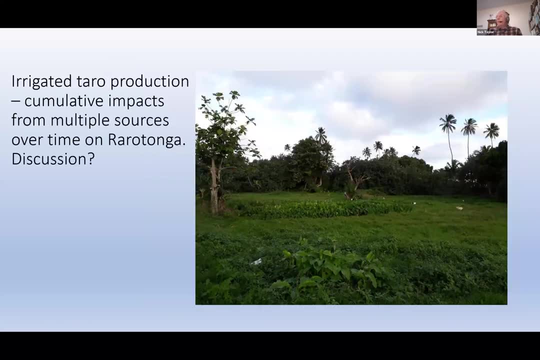 But I won't go into that because it's getting into too much detail. Next slide, please, Richard. All of that, by the way, also required a whole lot of consultation with the local Communities to get them involved in working out what to do. 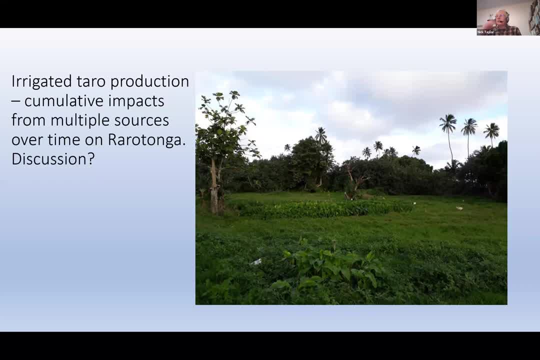 So this is my final example and hopefully pushing us towards the discussion side of things. I hope you will be able to help us here to accumulate some discussion. So I want to talk briefly about taro production in the Cook Islands. So we're not talking about dry land taro. 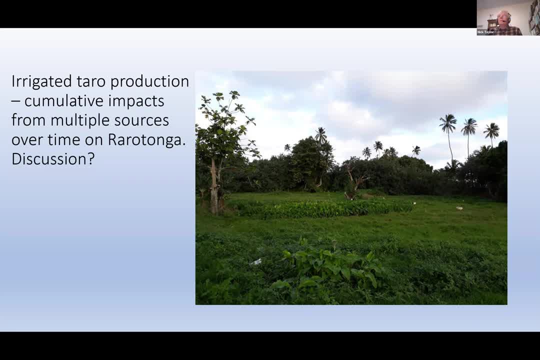 Here we're talking about irrigated taro. So what you're seeing here are the remnants or remains of an irrigated taro area area on Rarotonga. This is the irrigated taro, or taro vai was a key part of Cook Islands traditional society and agriculture and very bound up with the local culture and the way of life, with social organisation. 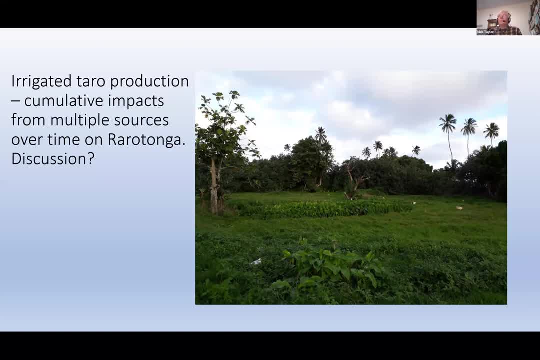 To ensure that, So that water from the streams running off the hills was able to be utilised in these lowland swamp areas or wetland areas next to the coast, so that you could grow irrigated taro. Not everyone on the presentation will be familiar with irrigated taro, but it's a really key part on many high islands in the Pacific. 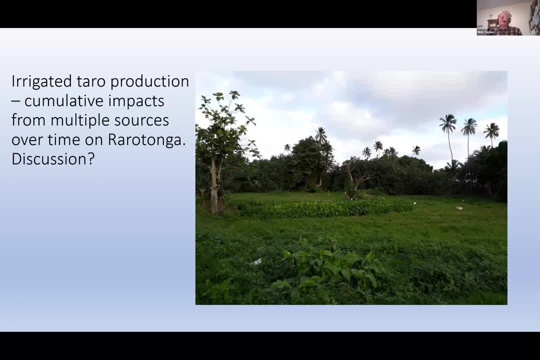 It's not just on Rarotonga, It's also found in Mangaya and Achu, in particular In the lower Cook Islands. So irrigated taro over time, as you can see, has deteriorated And a lot of this land is now just used to graze goats. 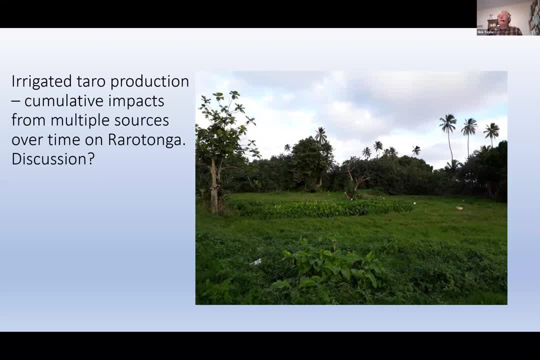 It's weedy, There's no sign of any irrigation system And the taro that is cultivated. Richard, that's in the taro right in the middle, the taro patch in the middle of the picture, If you move your cursor there. 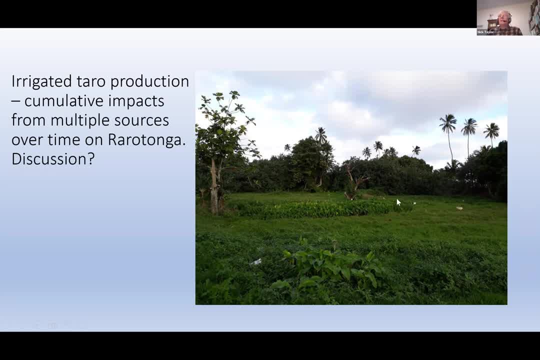 Yeah, that bit there That's actually been grown. That's actually been grown on a raised bed known locally as pai. So this is a raised bed taro which doesn't require irrigated water to keep it growing, And you can imagine that actually to have irrigated taro you have quite a complex system of management to deliver the water in a uniform way to the taro cultivation patches or areas owned by particular families or run by particular families. 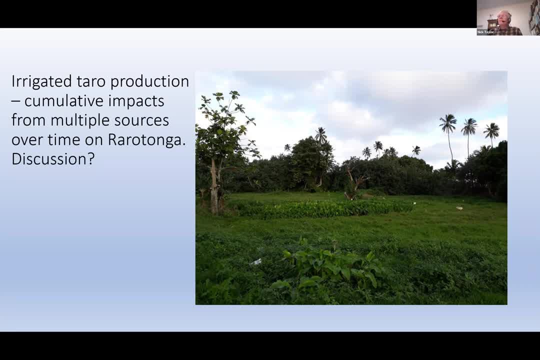 So I'm just interested in what you think might be the reasons why these areas of taro production have declined over effectively quite a long period of time. Certainly the last 20 to 30 years they have reduced considerably in area. I'm just hoping we might now use the chat. 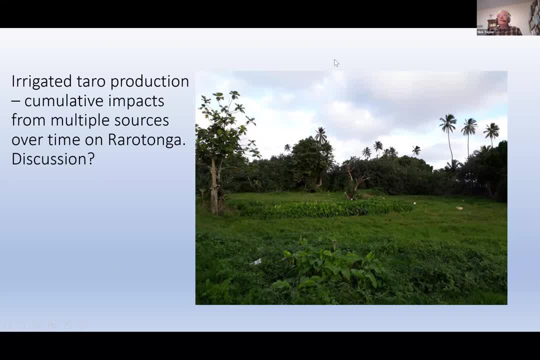 To Get you to jot down some quick thoughts as to what you think has happened here. What have been the sources of change to this very what was a very valued environmental and, I would argue, environmental and cultural components. So it was certainly a valued vector in the Cook Islands society or Rarotongan society. 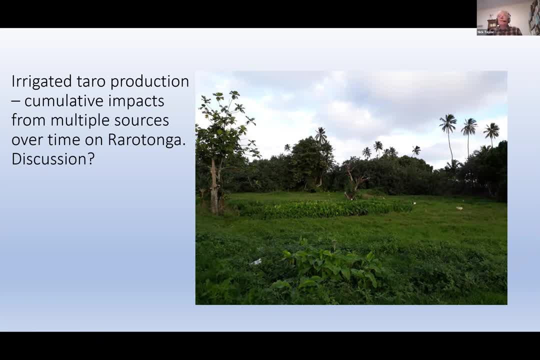 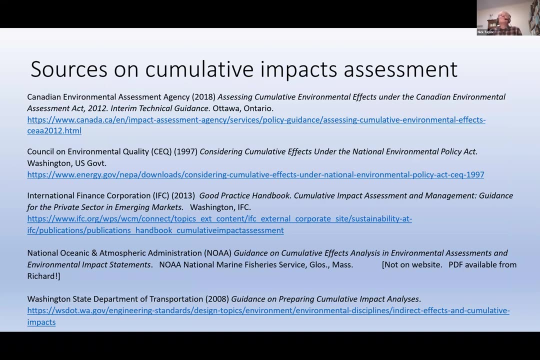 And I'm interested to know what you think might have happened here. What might some of the sources be? Let's go to the chat. Give you a couple of minutes to jot down some quick thoughts. I'm now bringing up my chat so I can actually see it. 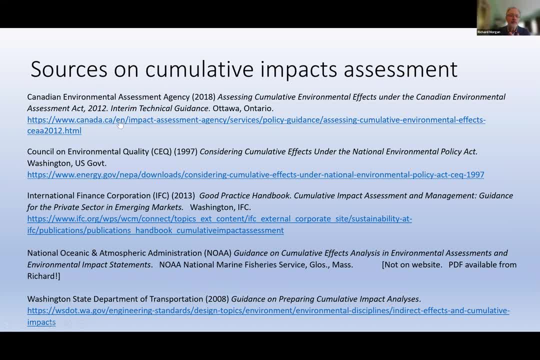 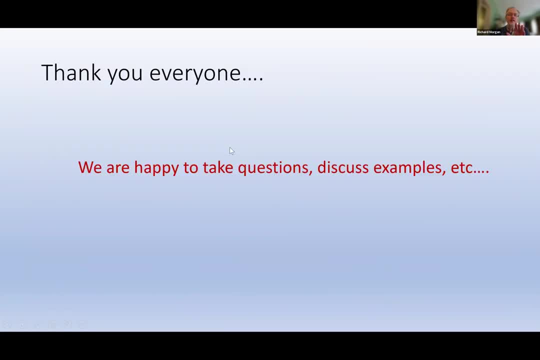 I'm just going to run the last, This slide of sources, Just to point out it exists And thank you everyone, And so we're happy to move on to talking. That means I can stop sharing the screen, which I think will make it easy for. 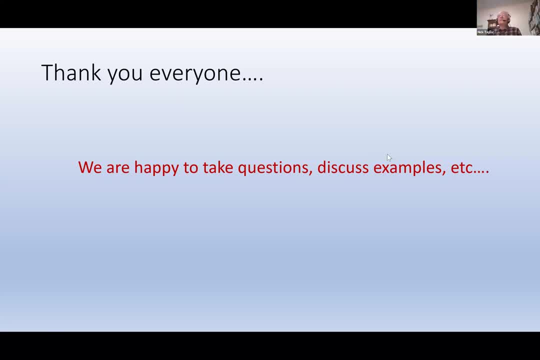 Oh for the chat. Thanks, Richard. Yeah, It's hard to see the slides of the chat at the same time, isn't it? Yeah, I think that's the way it might work. So thank you everybody for listening. 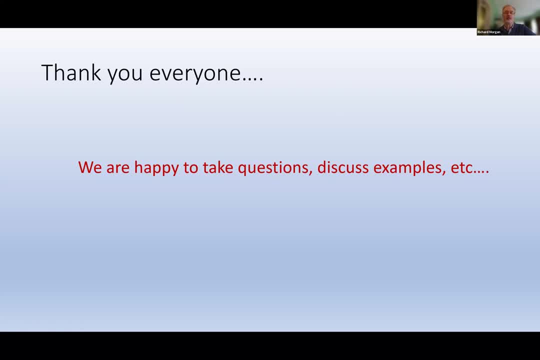 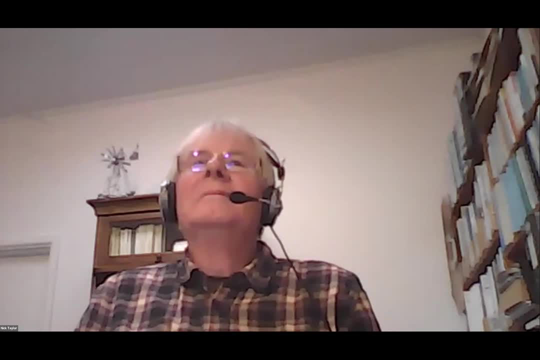 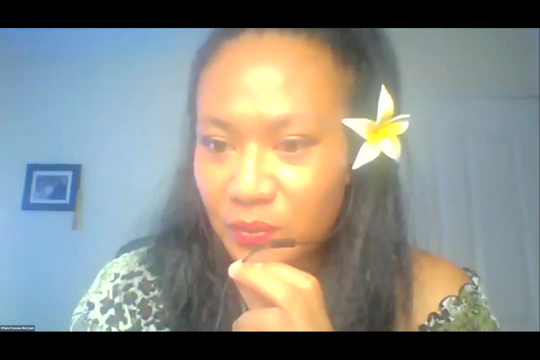 Now let's promote the interaction, Promote the interaction side, Interaction time. Here we go. I've got one of the chat there. No Thanks, Professor Richard and Professor Nick. There we go. We've got some answers there in the chat box. 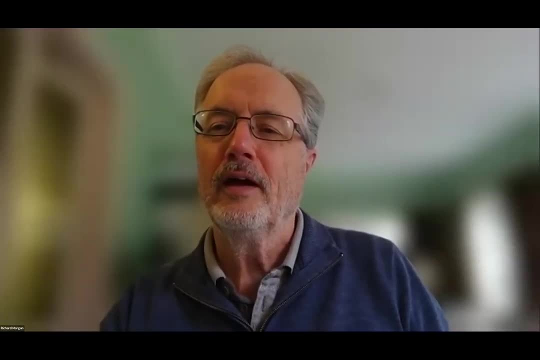 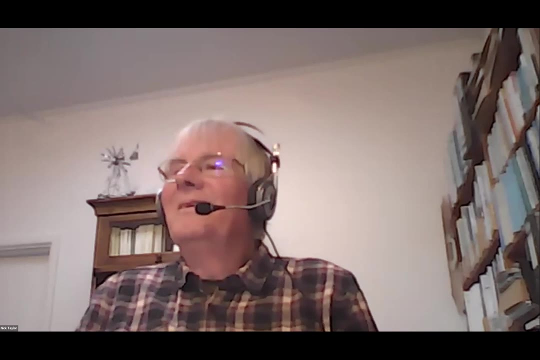 Wow, Yeah, Just trying to work out which is the beginning and end of the chat. So the first one: there is Overuse of land over time. Yep, Good Raising animals. Yeah, Rice is cheaper, That's a good one. 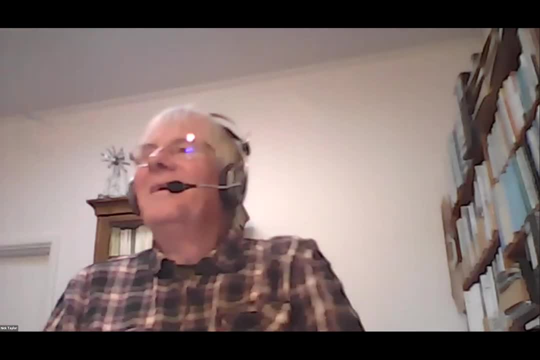 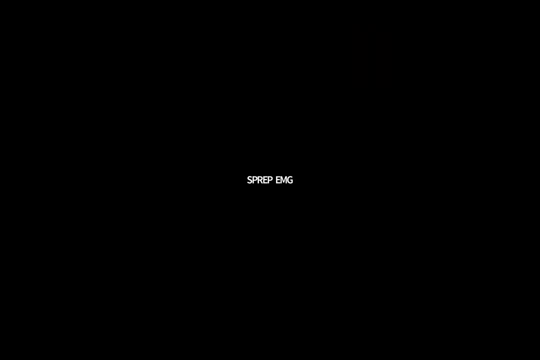 Yep. Rice is cheaper So it takes less work. Maybe saltwater intrusion? Yeah, Saltwater intrusion, Yep, Yep, That's a good one, Particularly where the, where the puna is close, The swamp is close to the, to the coast. 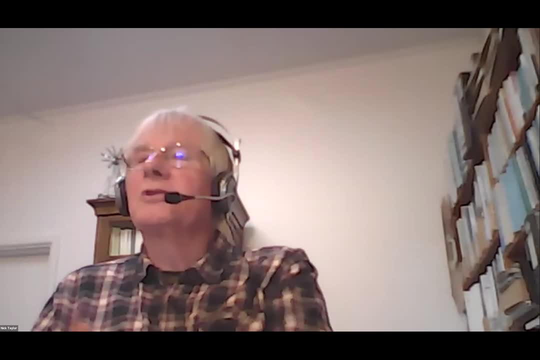 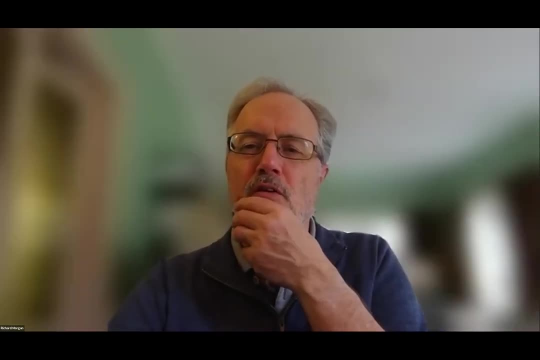 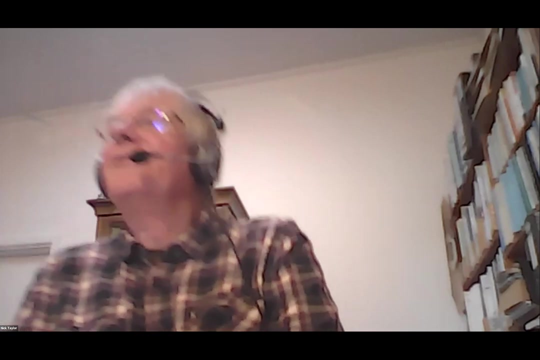 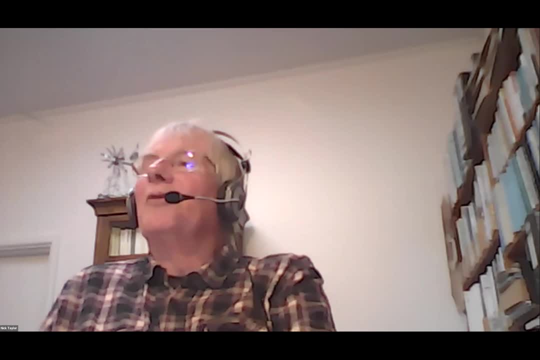 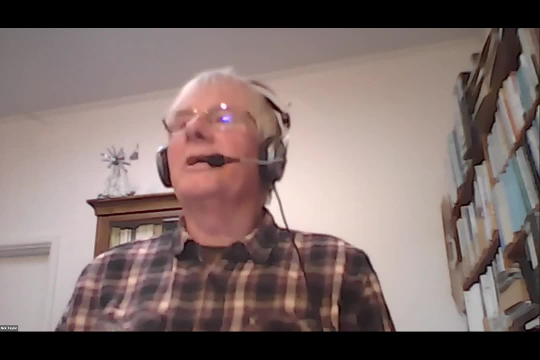 But it's also certainly more about people not taking part in agricultural cultural activities because, as you say, a cash economy- let's just say a cash economy- has seen it has been a part of the reason. So actually you have a combination of social and environmental changes. 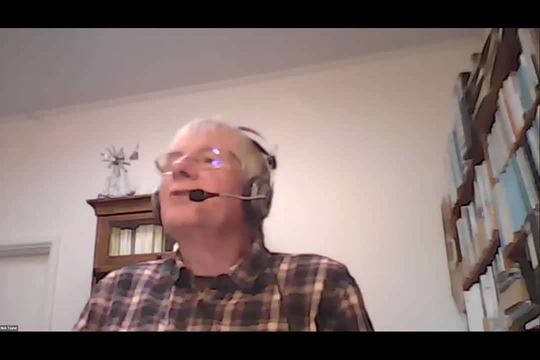 Let's have a look at some of the other ones. Overuse of land Infrastructure: Certainly infrastructure development has had a big impact. So road building, footpaths, all those sorts of things interrupt water flow and make running a complex irrigation system quite difficult. 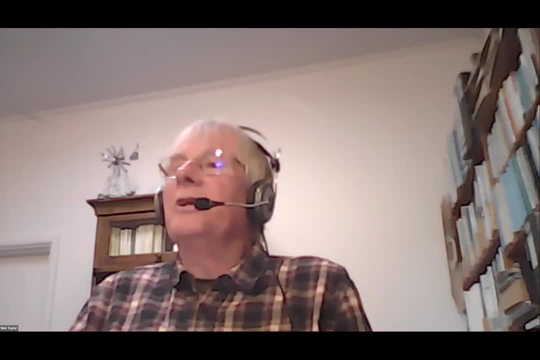 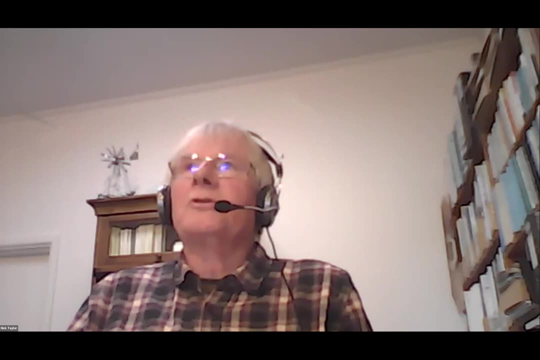 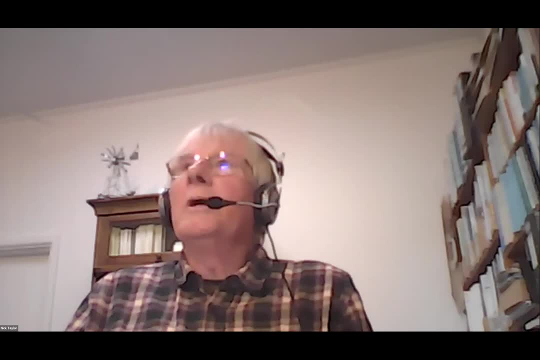 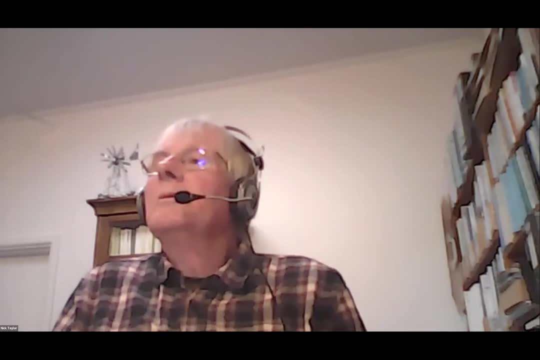 Cerebass is an example of how much less, Much, much less. Obviously there's a lot of competition for land on Cerebass misnomer, So taro cultivation has certainly gone away or been reduced to our conversation earlier. 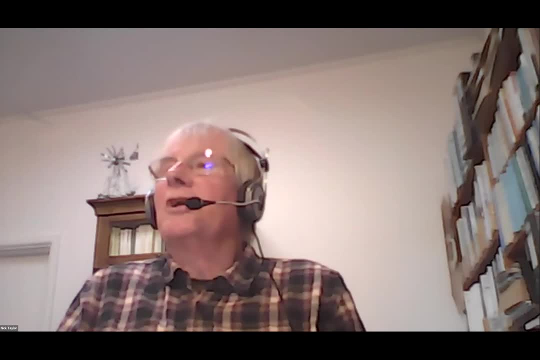 to increase absorption and distribution. Thanks, Thanks, Go on, boyfriend. how do you think that would change? immeris говорю kai marsi, tai e maore, Which forest is for you? because you property is most likely more Springs, when, on occasion, 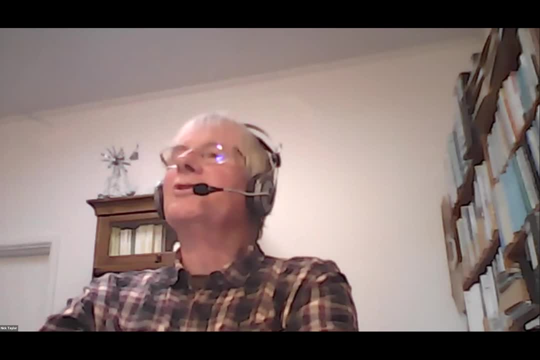 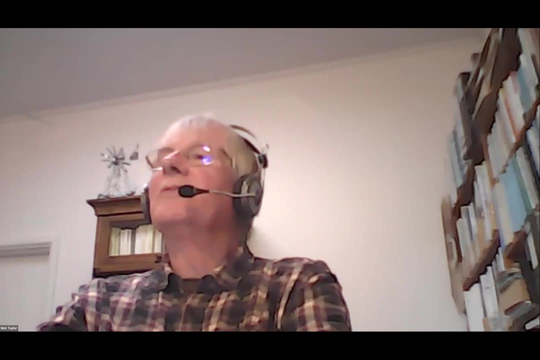 I've vomiting grass and then you苦ach. nothing to do with people Right? Thanks considerably. in Tarawa, Modernisation is an overall sort of thing. yep, Flooding or cyclone damage Heavy rainfall. you're absolutely right, it is an issue. 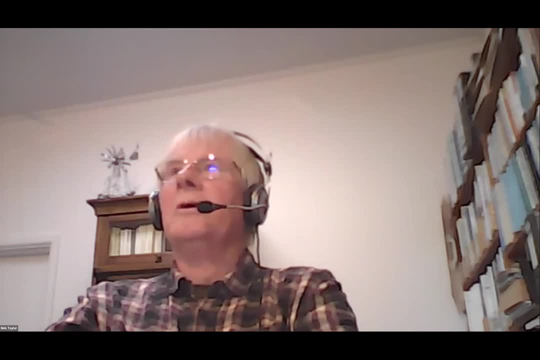 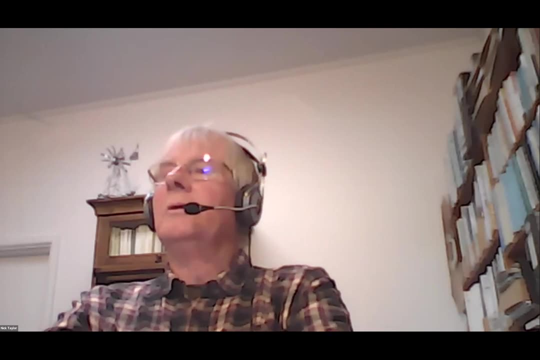 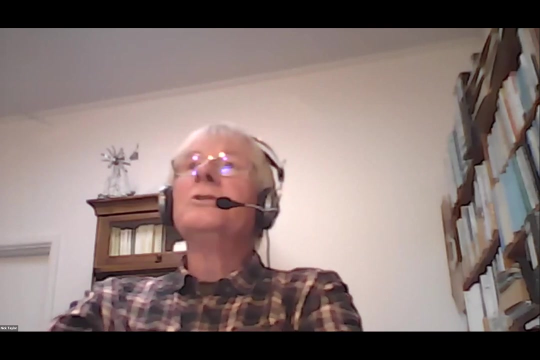 particularly in relation to sedimentation. So in a lot of instances, Tarawa swamps have been damaged by increasing sedimentation as a result of heavy rainfall events. So we've got the dietary change again. Yeah, different types of irrigation. So you'll certainly see instances of where the agriculture is produced. 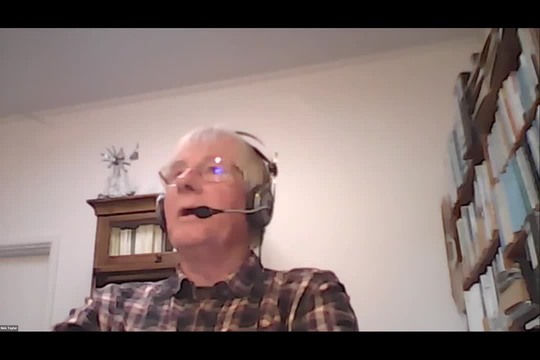 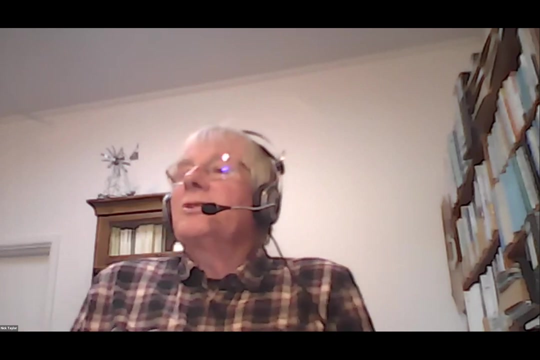 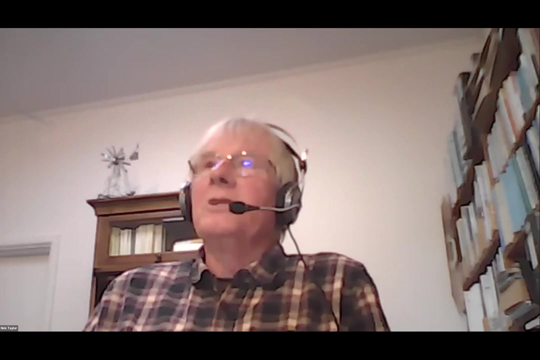 and produced in these lowland areas. you will see spray irrigation now, Small amount of trickling. We've got chemical irrigation going on. Pests and diseases of taro- actually I'm just skimming down here- was definitely an issue because we've seen imported taro varieties. 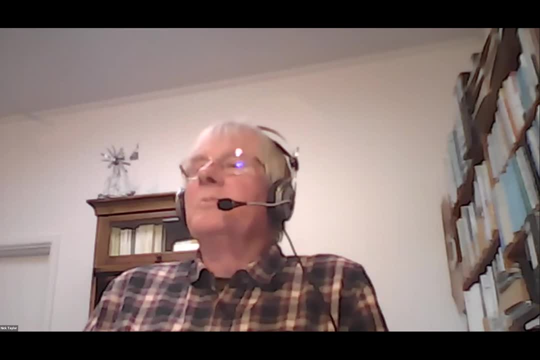 being brought in and in some instances, yep, there's been diseases introduced, So that's an issue as well. Okay, so we've got. let's stop there, Richard. Thanks everybody. We've had lots and lots of good reasons. 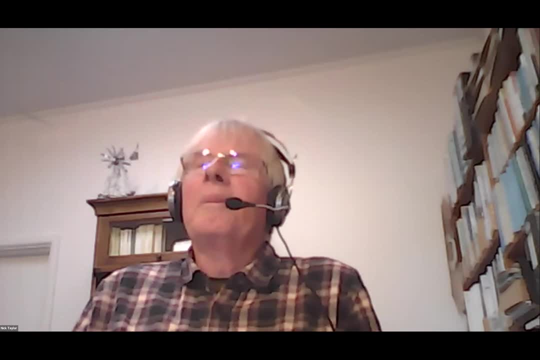 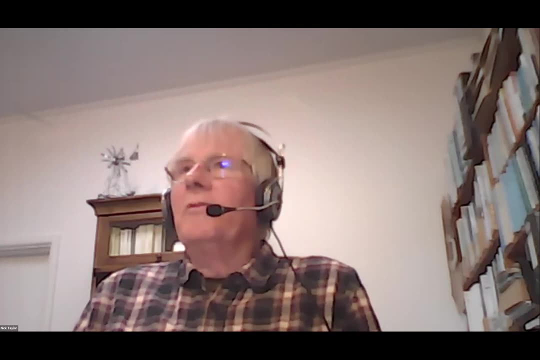 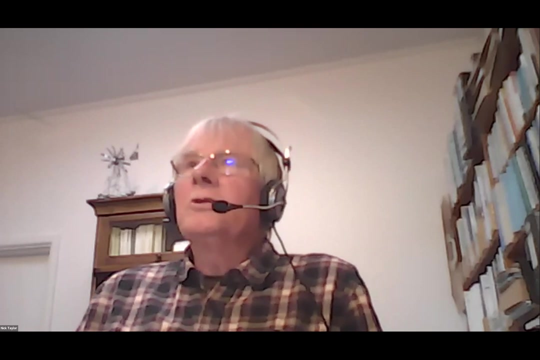 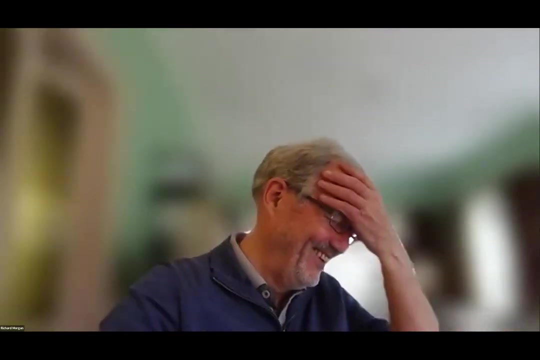 So what you're seeing? there is actually a problem that has multiple sources that have compounded together to give you a cumulative effect on traditional food production systems. So what, if anything, would we want to do about that? Richard, do you want to lead off that side of the discussion? 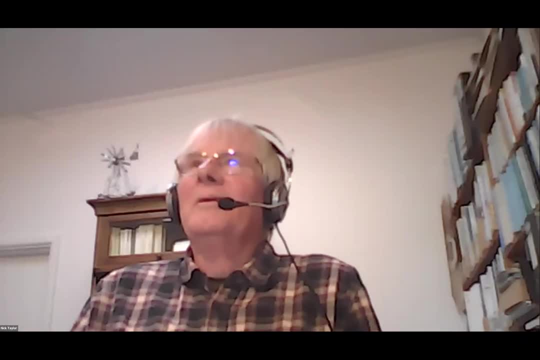 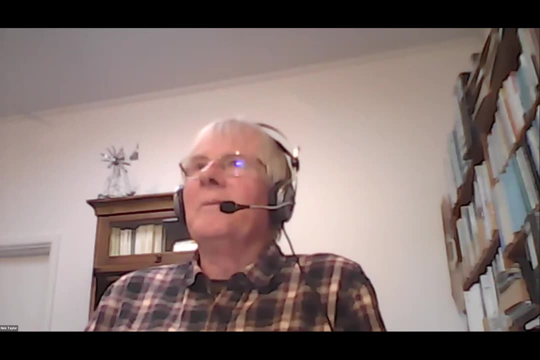 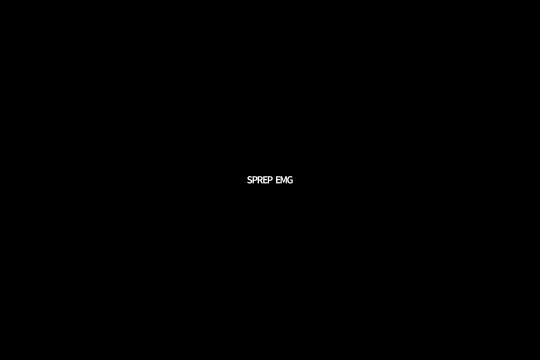 How would we respond as environmental planners, in terms of environmental management and utilising the tools we've learnt about today? Sorry, Nick, just one more that popped up towards the end. There was a couple more that popped up. There was actually one from Ness, from Cook Islands themselves. 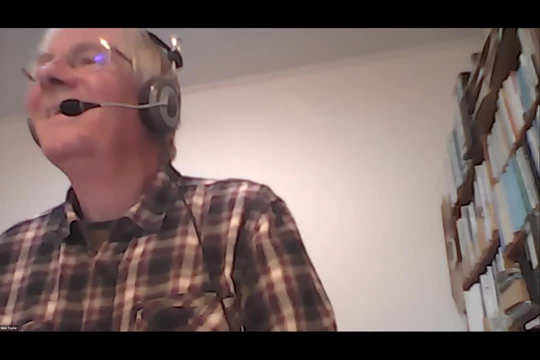 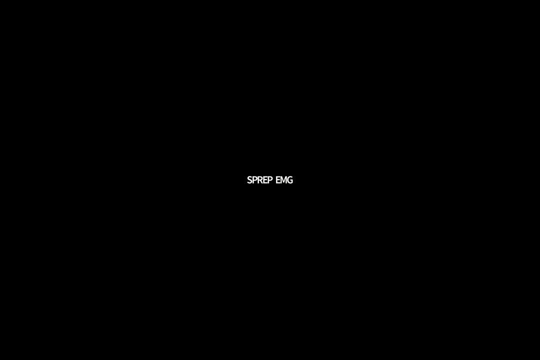 So lack of knowledge of benefits of wetlands. So maybe want to let everybody know that Cook Islands is posted there. Sorry, I'm going to turn my mic off again. Is that what Ness is? is it Okay? National Environment Service. 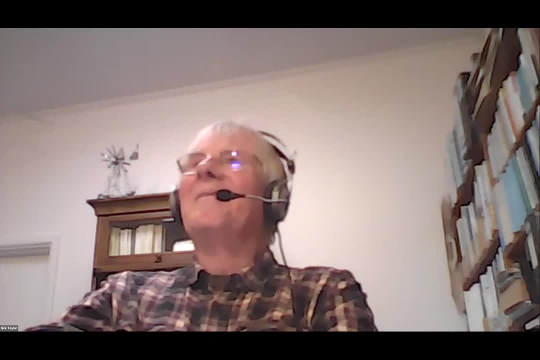 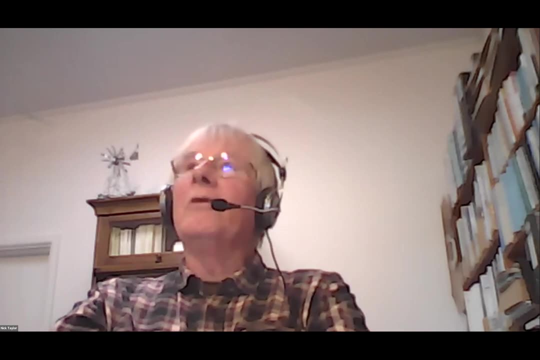 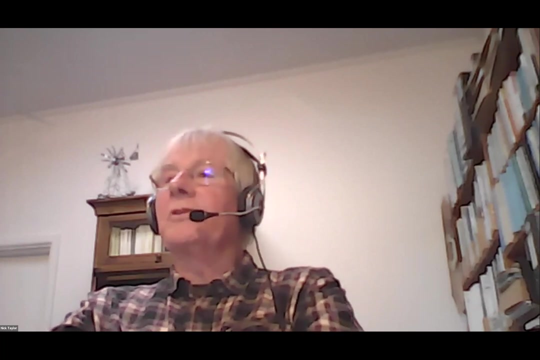 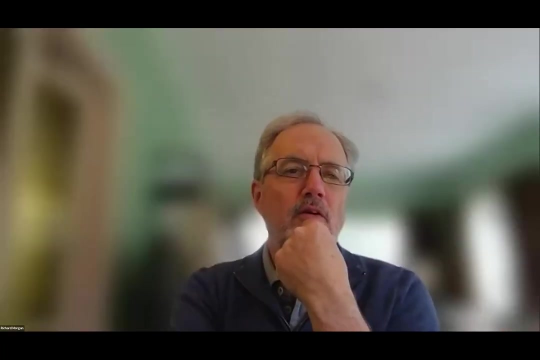 Okay, Yeah, I agree. Lack of probably an attitude crept in over time about the value of the wetland areas for agriculture and also for their intrinsic values as wetlands. So, going back to your question, Nick, what would we want to do about that? 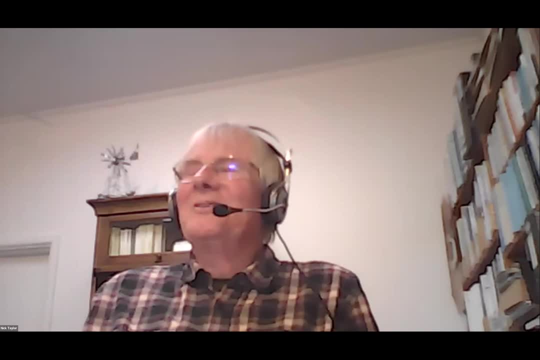 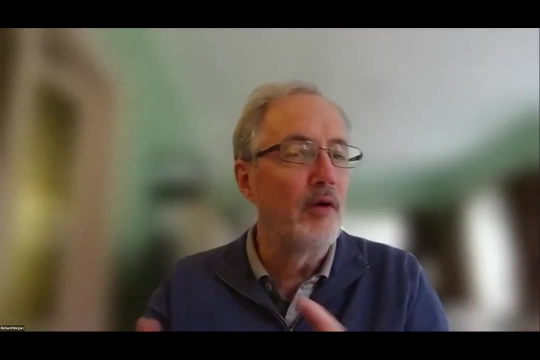 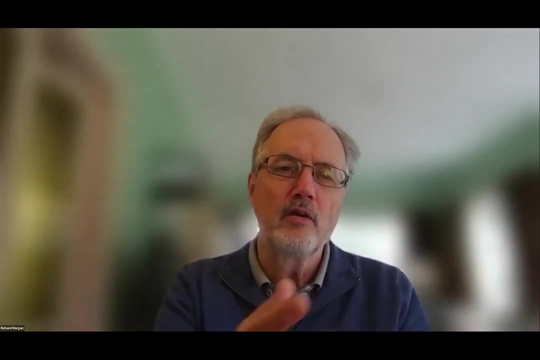 Yeah Yeah, Pest and diseases- All right, Sorry. Sorry, Richard, They're still popping up. That's great. You're asking me to lead off how we might respond to from the management side, I think connecting back to those ideas of cumulative impact assessment process. 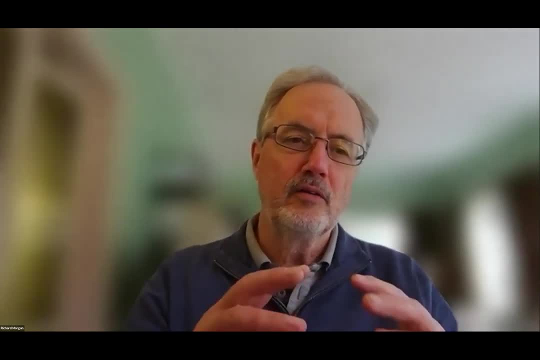 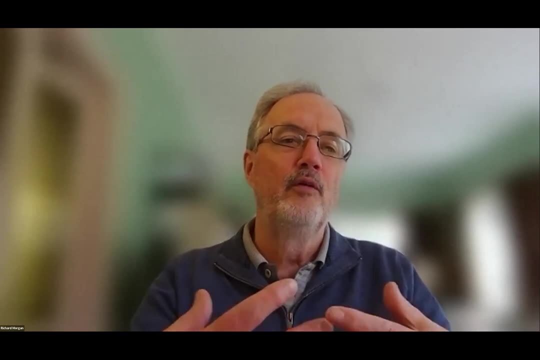 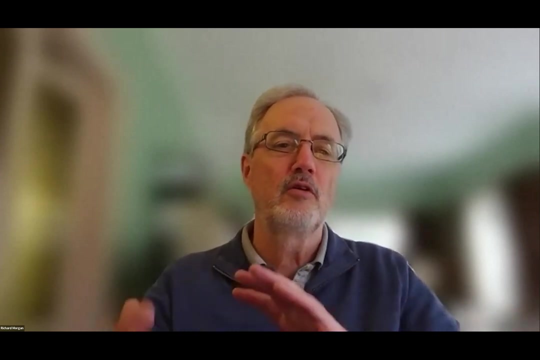 The very first thing is to sort of pose a question with local people, local communities. is irrigated taro a resource that you want to continue? Does it have the value culturally, economically, socially, that you want this land use system not just to survive but to thrive? 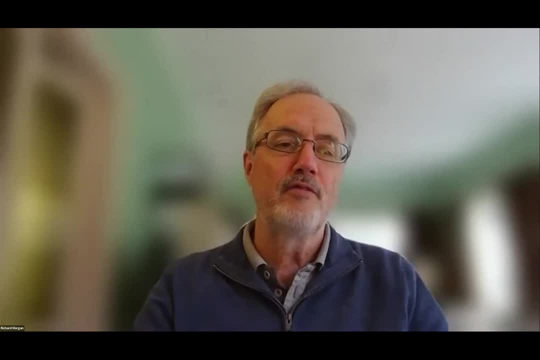 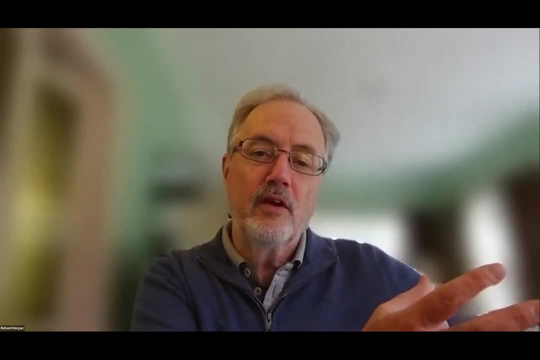 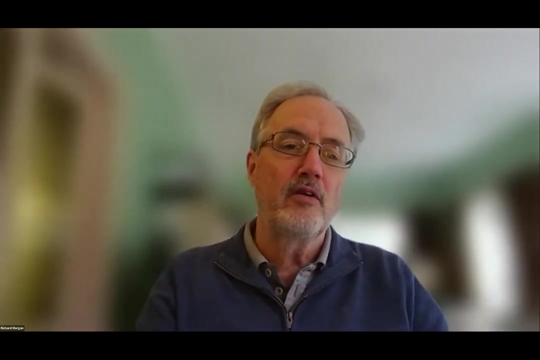 And if so, then that gives us our focus for the cumulative assessment. And then we start looking at that sort of the historic context, the fact it's declined, why it's declined historically, its current state of health, And then we also look at the current activities that are going on that may be continuing to. 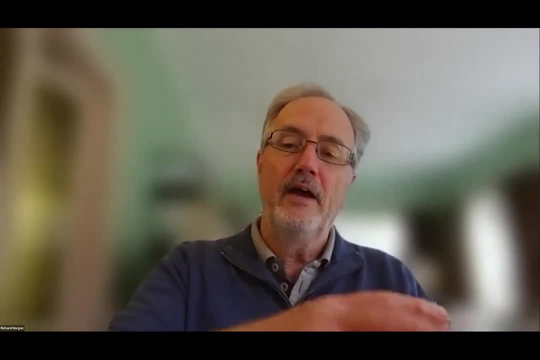 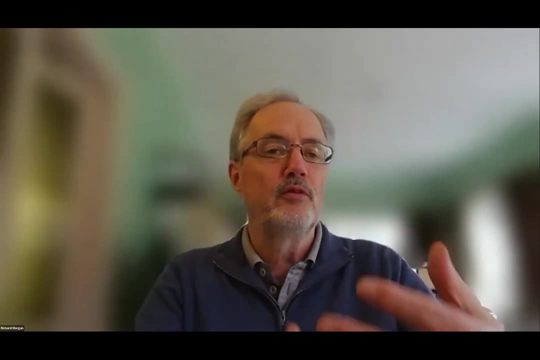 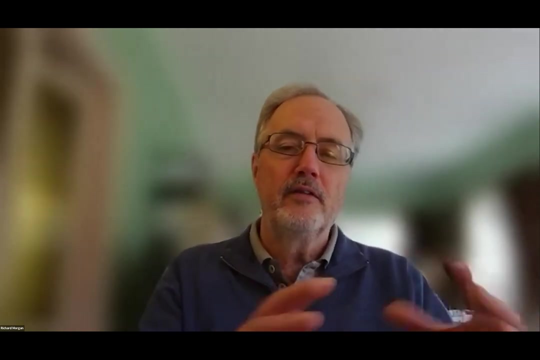 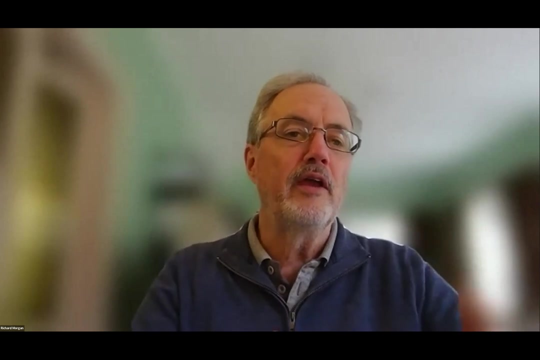 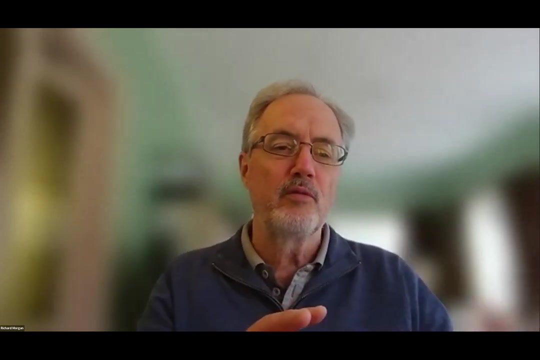 threaten to put pressure on the system And how we might deal with that from a strategic perspective, which in this case would presumably be some sort of agricultural land use plan policy plan at the national level to regulate activities that might threaten production through the different cause effect pathways. 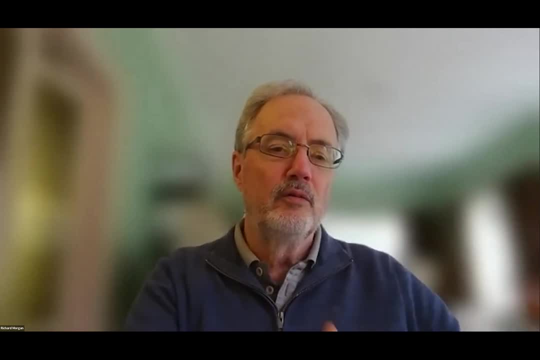 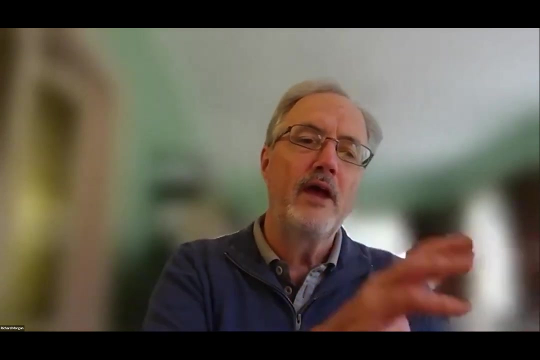 that we've identified, try and reduce those effects through different strategies, regulation, education, Investment And so on. So it's, you know, the model that we had earlier on you can sort of use to address that type of problem. 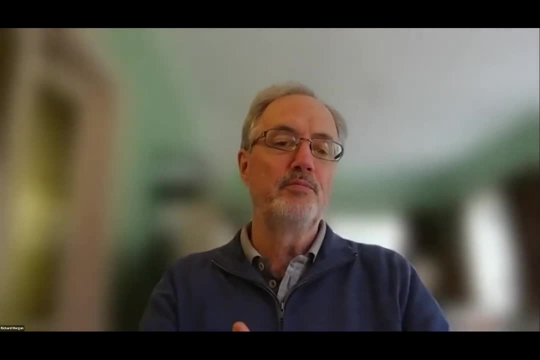 Thinking in terms of the cumulative pressures on the system, the fact that we value this resource and we want it to continue, And we can apply that sort of structured thinking To why we're in the situation we're in and how we might move to get out of it and secure the future of the land use. 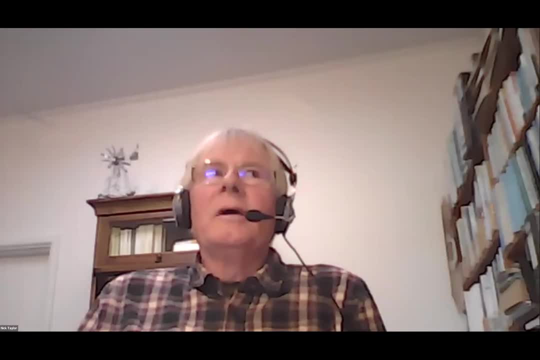 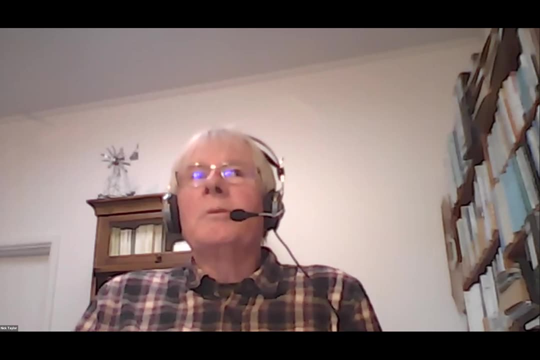 Absolutely Or something like that. Absolutely, And it's probably a combination of policy things going on, So there's probably some policies required. Well, they are developed in many places now around the emphasis on local food production As a food security issue. 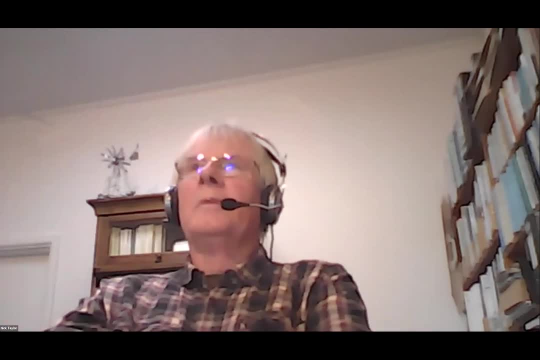 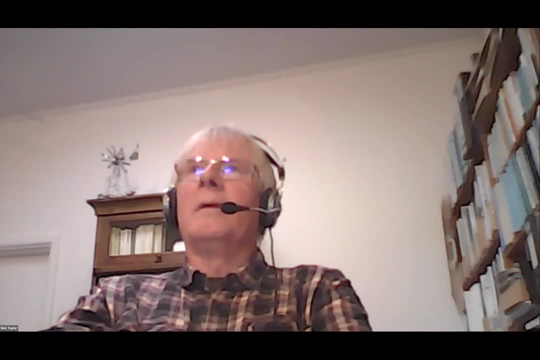 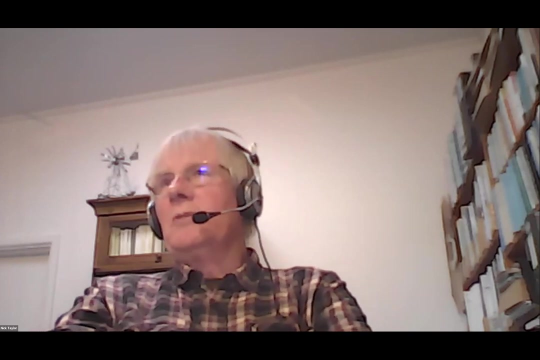 That's certainly, I think, acknowledged, Certainly some regulation perhaps, or rules around land use, urban development and so forth, Probably a lot of things. going back to what the comment was about valuing wetlands, I mean just valuing wetlands for their intrinsic values. 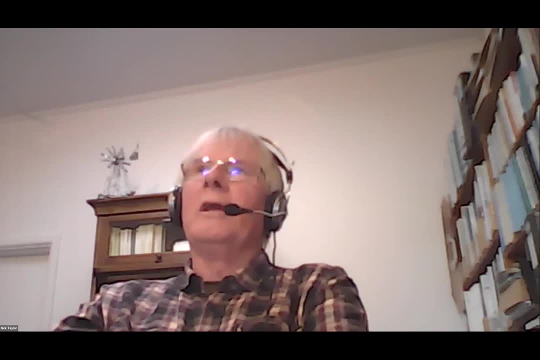 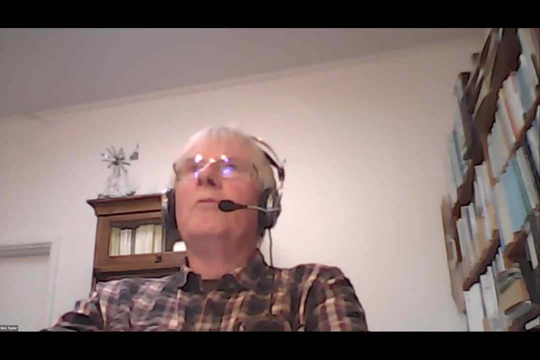 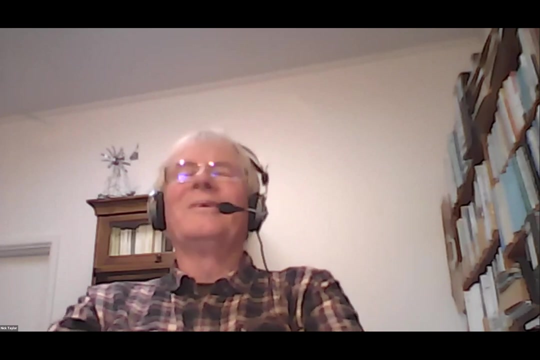 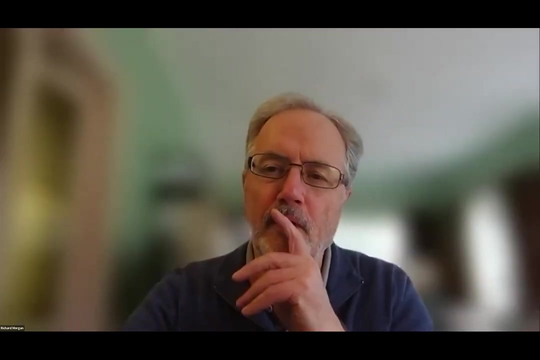 But also for their potential production, Potential productive values of something that is still Irrigated. taro is still recognised culturally as important And people still like to eat it if they can, So, yeah, it's still a valued foodstuff. There's a nice example from Edward at 2.22. 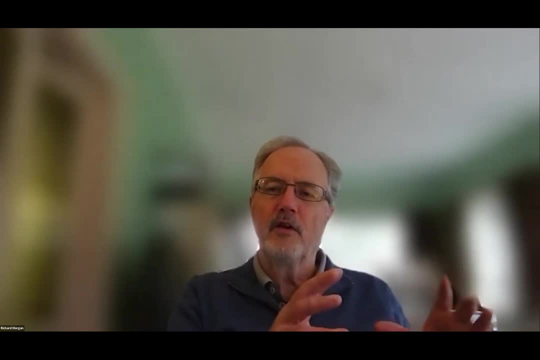 The example from Honiara. It's about flash flooding caused by cumulative impacts from runoff Using the lack of proper planning of the city And again, that's a really nice example of how you do need that strategic overview if you're going to plan for a city or a resource or whatever. 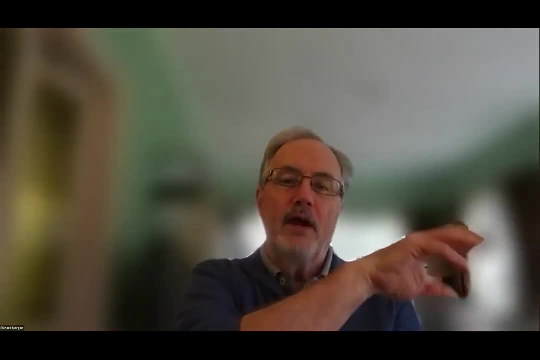 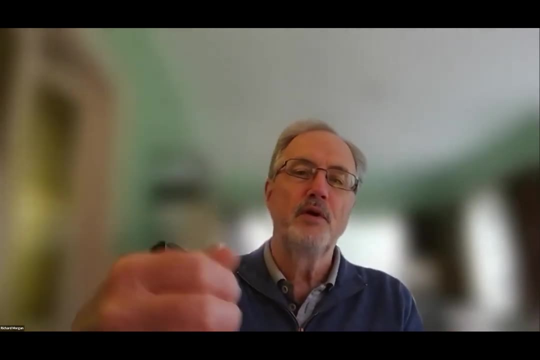 That you have to identify the different impacts, the different threats that are coming from different areas. It might be the same problem that's repeated right across the landscape. So deforestation in steep landscapes such as around Honiara, and rapid runoff and flash flooding. 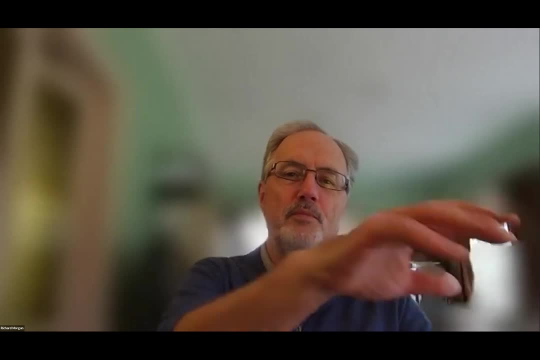 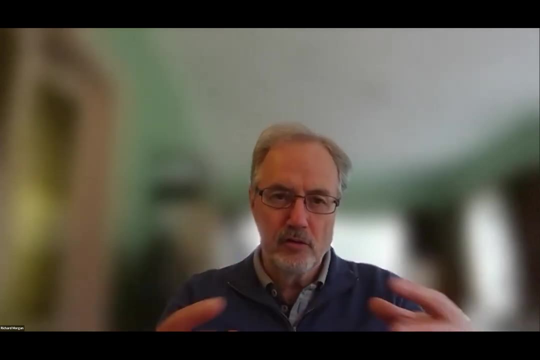 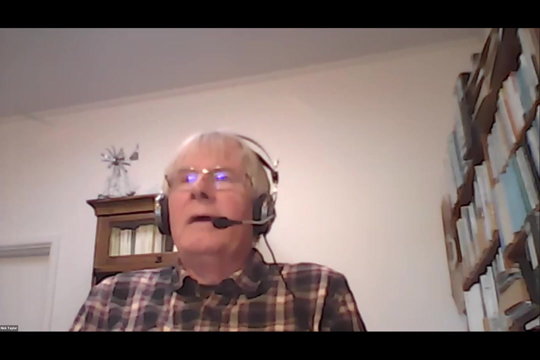 So that connection between multiple activities, multiple impacts and often the need for a coherent strategic response, Just time and time again, That's a nice example, Paul and Edward, Yeah, and I think the point about that is there are the tools to address, say, individual developments. 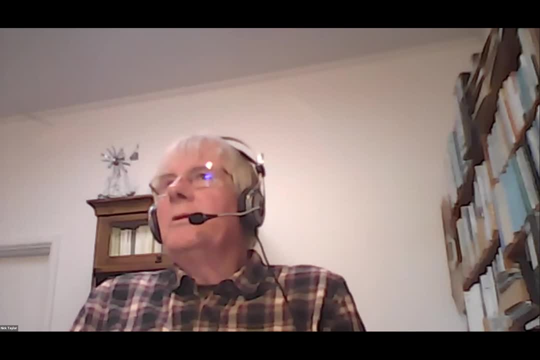 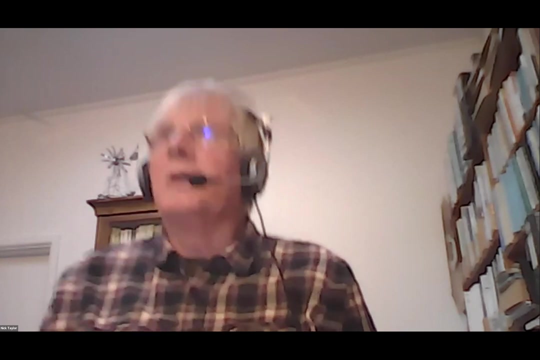 Say a resort development in this kind of land, which has happened in the past, To ensure that the environmental assessment of such a development includes some consideration of the cumulative effects. Also, infrastructure like roading, piping, water piping- In Rarotonga, as in many places, the whole sewerage infrastructure needs considerable thought in the move away from individual septic tanks and outflows. 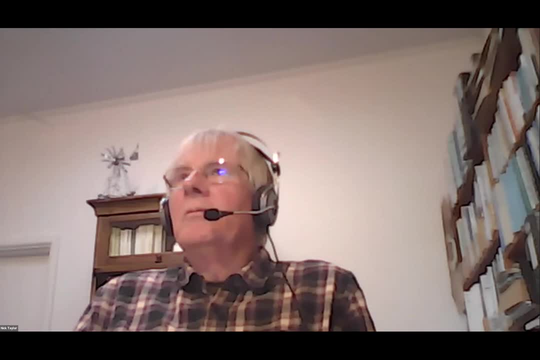 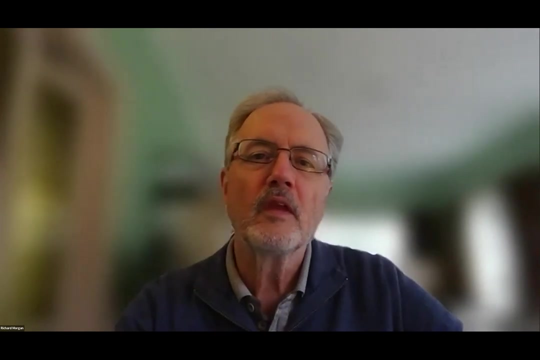 Something that's more of a community or a broader based wastewater infrastructure. There's lots of things to unpack in. here is what I'm saying. Yeah, yeah, definitely, The airport lies on lowland, all the way. Professor, we have Nick as a question, please. 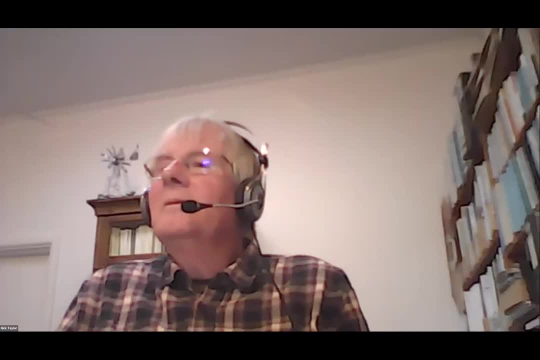 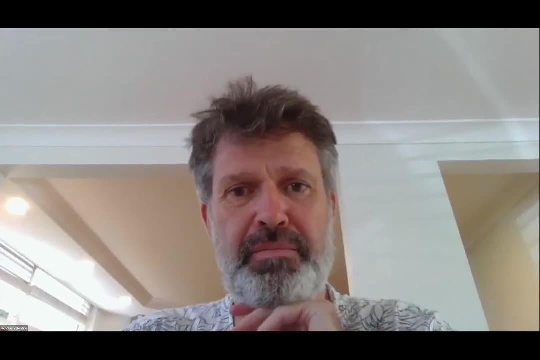 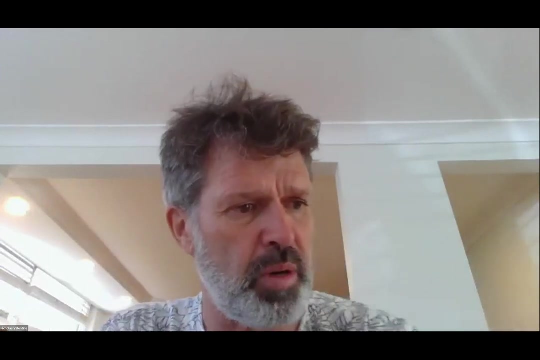 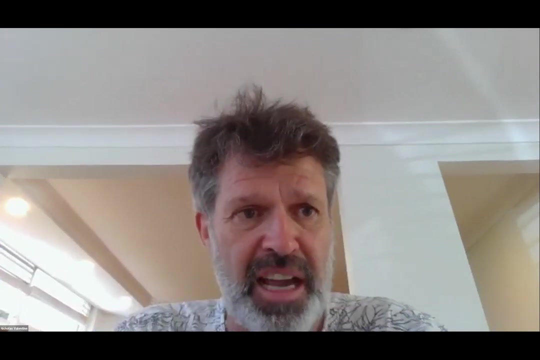 Yes, Yeah, hi, Nick and Richard. It's Nick Ballantyne here, A consultant to the World Bank. Thanks for an excellent session and a very timely one from my perspective, where I'm putting my mind to the impacts of sedimentation on coral reefs in Palau from a development project up there in a landscape of very, extremely high soil erosivity. 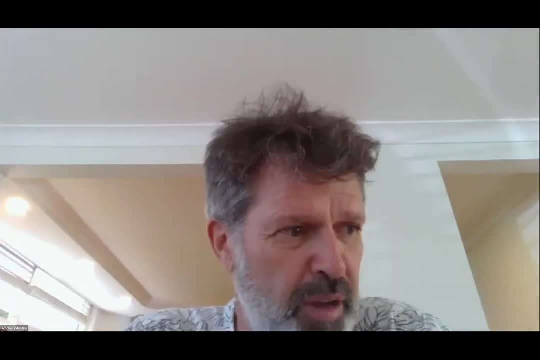 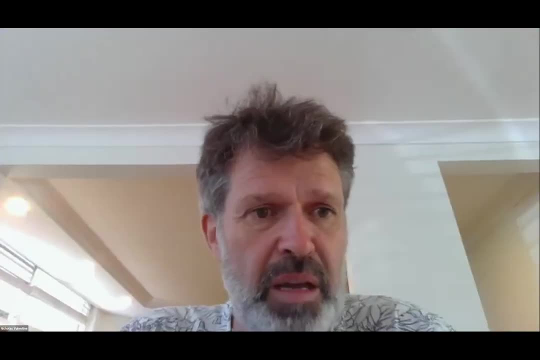 I just wanted to return to your example. I was fairly heavily involved with the implementation of that project with the World Bank And yeah, look, it's one of these vexed issues, I guess, with public infrastructure in the Pacific on customary land. 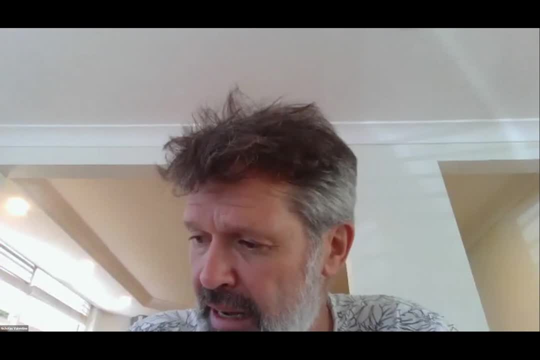 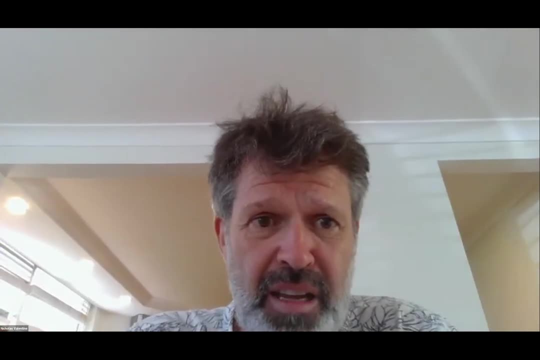 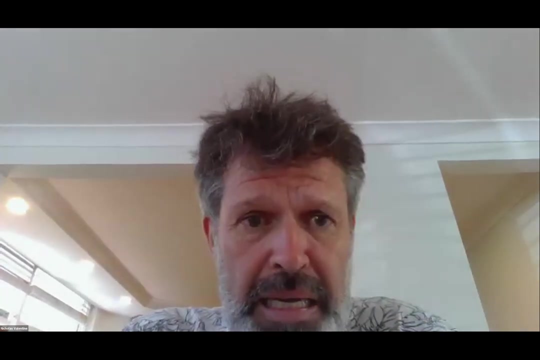 I forget the actual status of the runway in Tarawa, whether it's fully acquired or not, But certainly in Tuvalu the runway is half customarily owned And it was found at the commencement of construction, very inconveniently, that the landowners hadn't been paid their rent for the past five years. 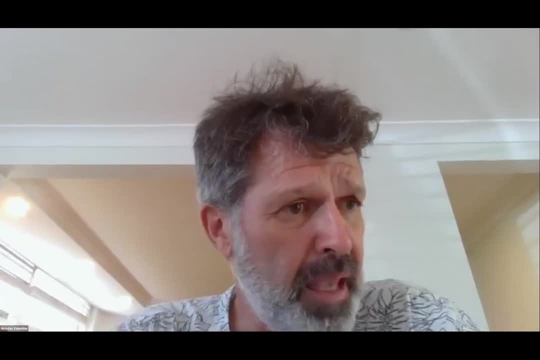 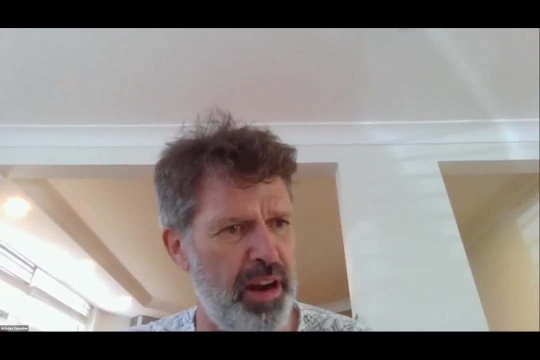 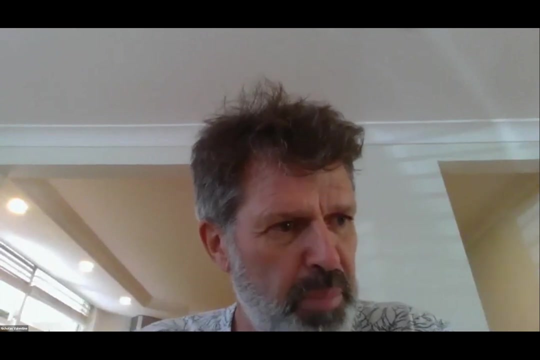 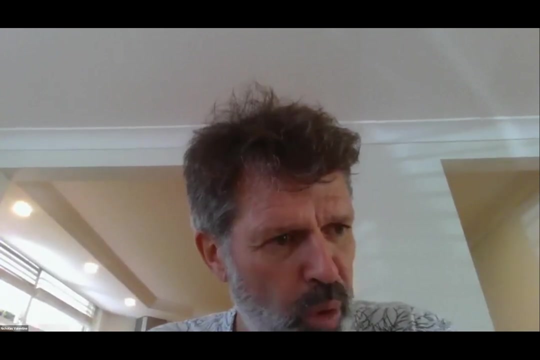 So the contractor had to stop work. But returning to Tarawa quickly, the water reserve you mentioned, there's a number of issues around that of land tenure acquisition, but also cumulative impacts And the nexus with valued components. So in preparing the water supply project for Tarawa for the bank, we investigated the tenure of the water reserve. 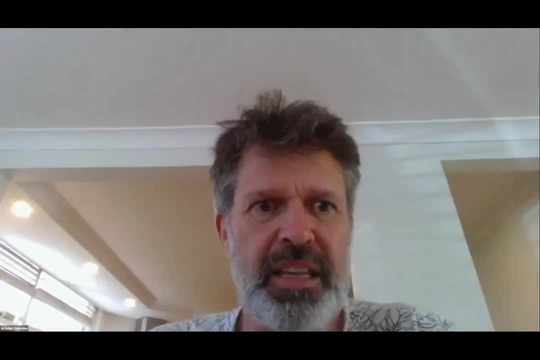 And the government asserted that they had acquired, The landowners said no, it was actually leased. There was no paperwork to verify either way. So it was a bit of a standoff And it was unresolved, But the cumulative impacts that we were trying to achieve. 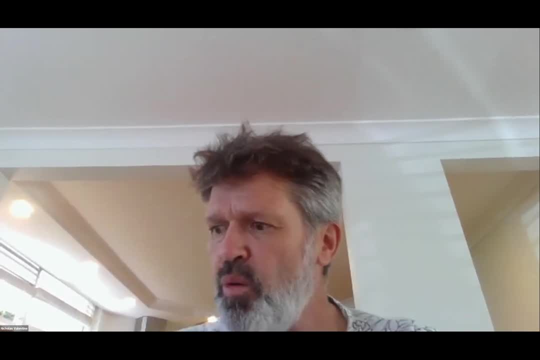 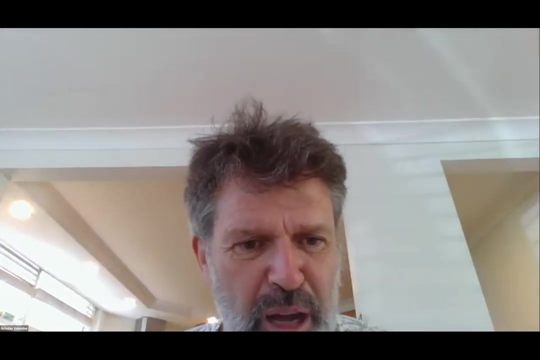 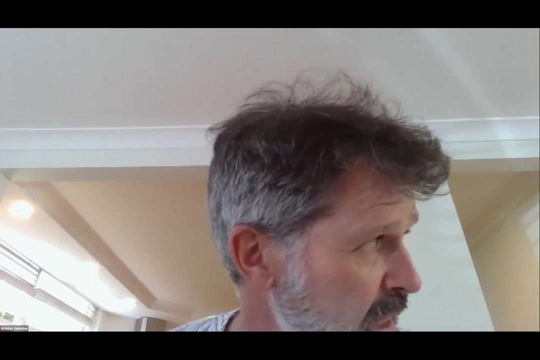 The government to consider were the increasing encroachment on that water reserve. So it's the only remaining natural, largely uncontaminated water supply on Tarawa. The remainder of the water reserves have been rendered unpotable, But there's encroachment. 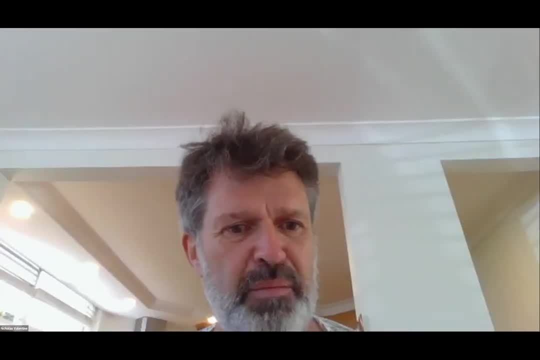 So there are small market gardens, There's small residences, There's a cemetery, There's toilets, dropped toilets, There's encroachment from the fringing settlement, which has actually moved off the water reserve when it was declared. But at what point does that cumulative impact marry up against the valued component of the water supply? 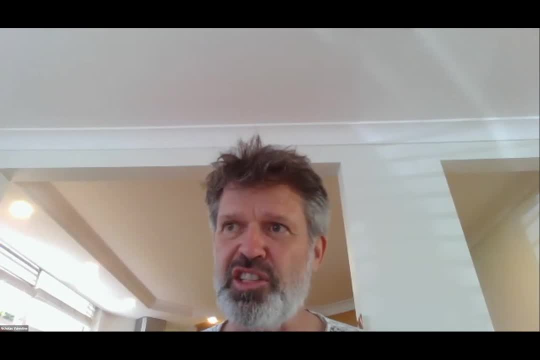 As in it's increasingly in jeopardy. How much does the community and the country at large value that component and are prepared to protect it. Now, with the prospect of desalination plant coming, perhaps they're more relaxed about that. But personally I would not be putting all my eggs in the desalination basket. 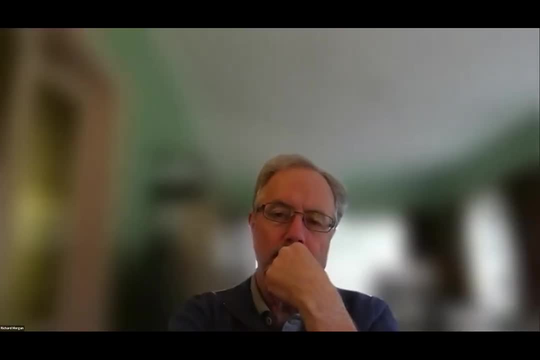 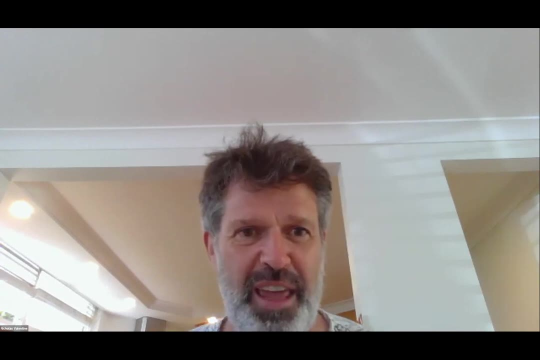 And I would be doing my best to retain the integrity of the only native water supply that remains. So just to add on to that example, There's all sorts of things going on there in that airport vicinity in Kiribati. Over There are 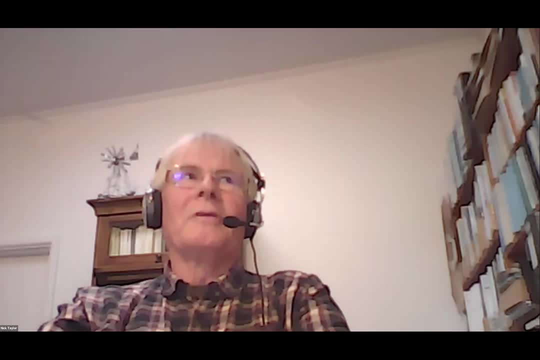 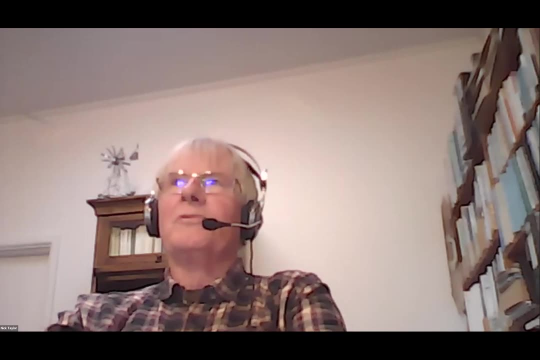 And you're probably aware that to the other side of the runway, to the other side of the airport, there's a big proposal being floated for an urban development project where the existing fish farms are on the south side of the runway. Yep, They will sink, Nick. 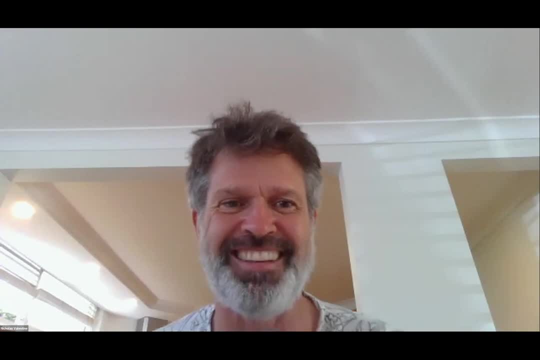 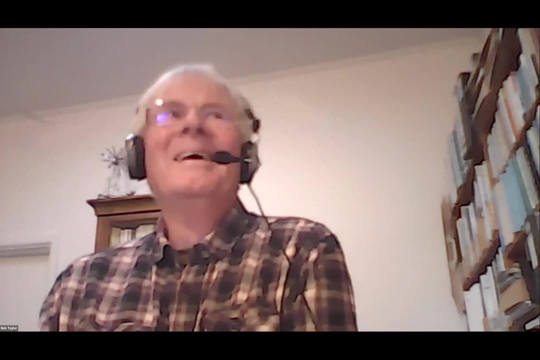 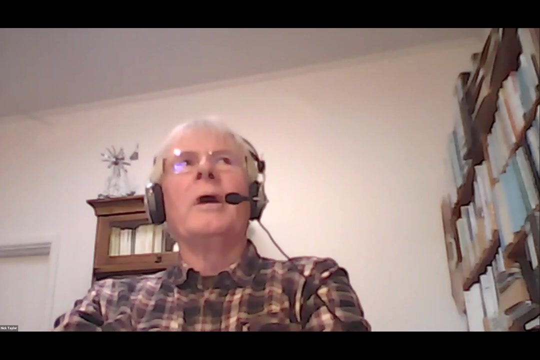 They will sink. They will sink into acid sulfate soils, Let me assure you They may well. But anyway, Yeah, I think. I think it's a great example of how something like that, like what you would think, would be quite highly valued in terms of the fact that it is the only major you know land based water, water lanes other than rainwater collection. You would have thought that would be quite highly valued. I mean, in the end it's up to societies to make decisions about these sorts of things, what it is we value and what we don't. I mean it might be the same thing. You know how much do we value a coral reef that has been affected by saltation, or a wetland or a river system, And in this instance, a water lanes. societies have to have mechanisms that are able to keep the river running, And then we have to have the ability to control the water. 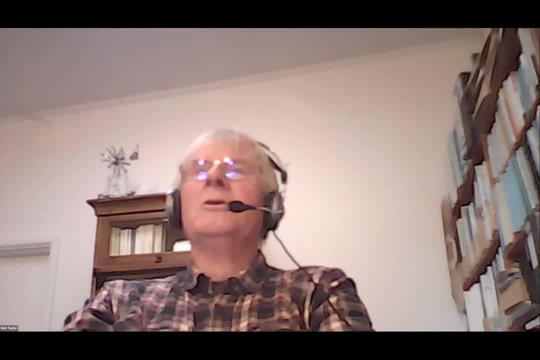 And in that way, we can make decisions about what we value and what we don't, And so I think that's a really good example of how we can do that. Yeah, I mean, I think it's a really good example of how we can do that. 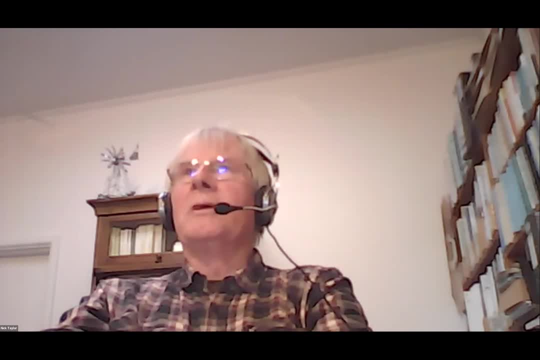 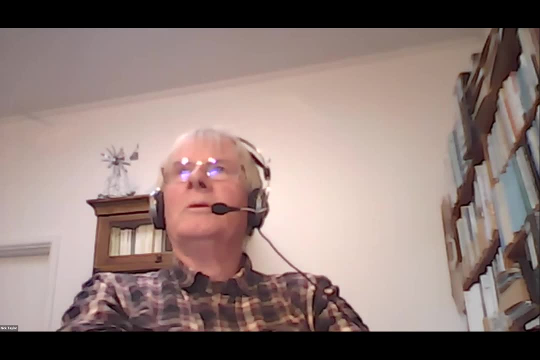 I mean, I think it's an interesting example of how we can do that. I mean, it might be the same thing. How much do we value a coral reef that is being affected by saltation or a wetland or a river system? 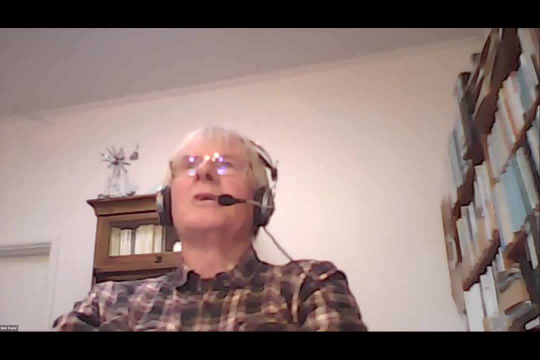 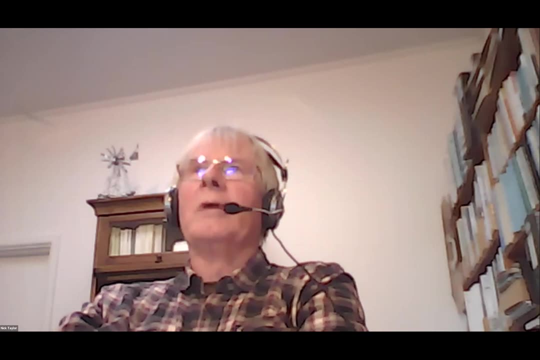 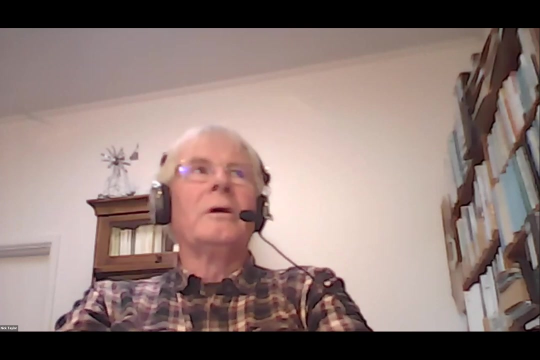 And in this instance a water lens. Societies have to have mechanisms to actually come to those decisions. I guess, and say, well, actually it is worth making, setting some rules and some standards. I mean basically here in Aotearoa, New Zealand. 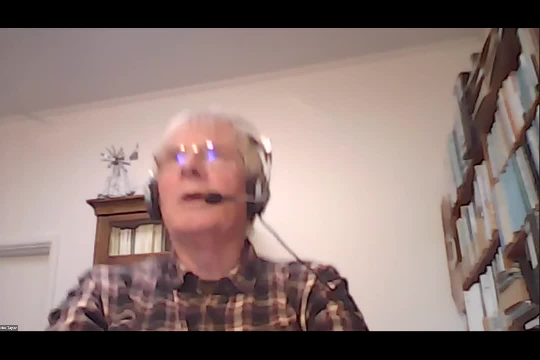 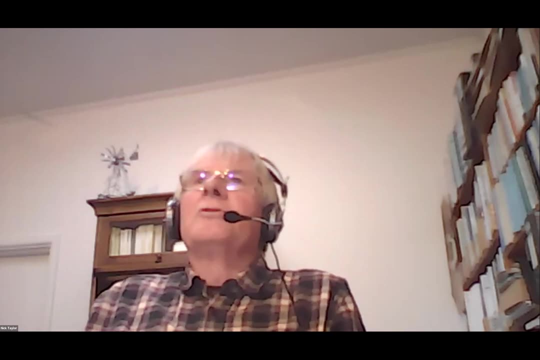 we've gone through the same thing in terms of freshwater management, where, when the cumulative effects have got to the point where you say enough's enough, we actually have to do something about this, And I think that's often the case. So it goes back again to that ability. 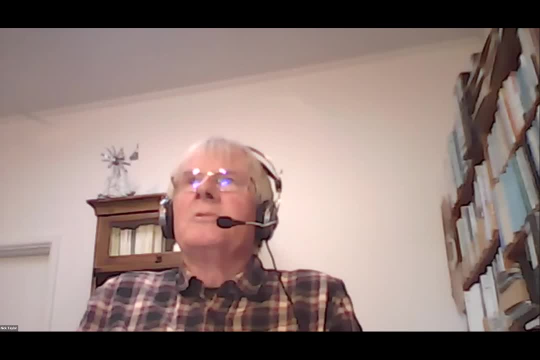 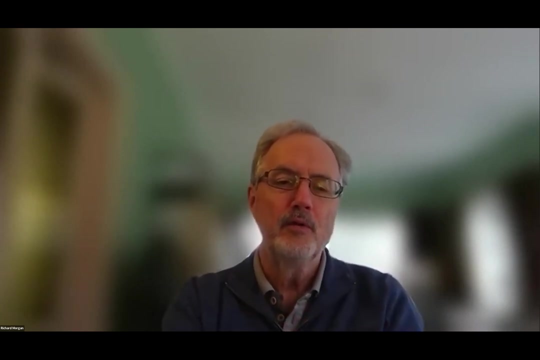 to actually make those strategic decisions and set some standards or some rules, regulations and so forth in place To protect Richard. do you want to comment? I think I'd just add that we value is usually recognised when it's either health that is affected. 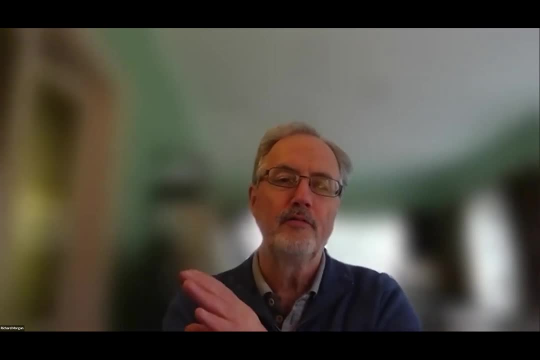 or people's pockets are affected, Either the health value or the economic value- And you know so- if it was seen that there were real health, the effects of the water becoming more, either more polluted or just less available, or the economic impacts of having to pay. 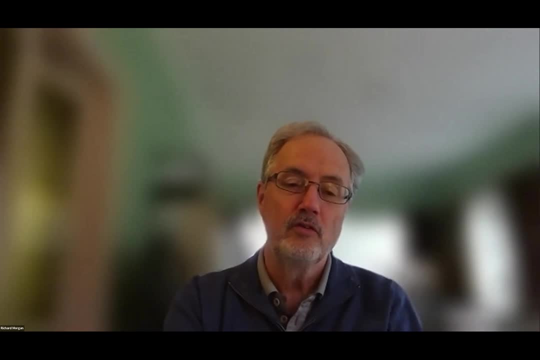 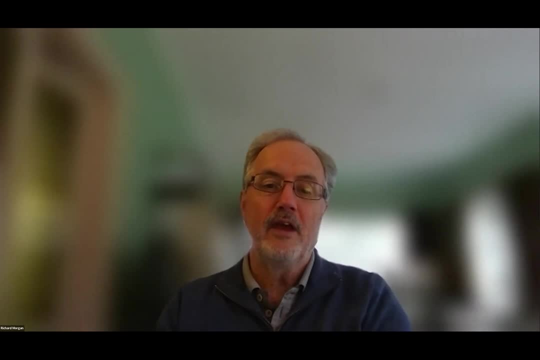 you know the functional value and the economic value of these resources And therefore maybe we have to set some sort of regulation in place to manage those things coherently. But there's got to be some sort of interest- self-interest collectively as well as individually. 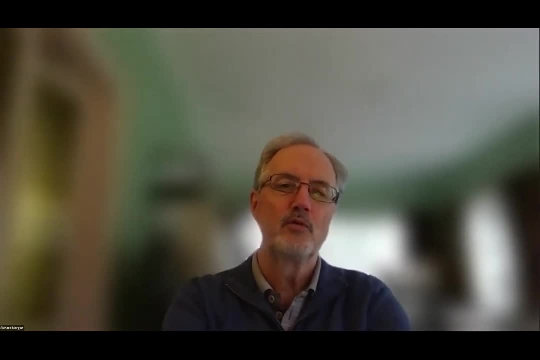 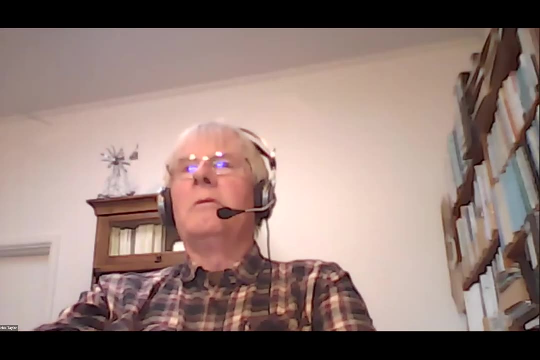 in, you know, managing these resources, How to establish that, especially at a local level, And certainly in a place like Tarawa where there's- you know, I mean, everyone recognises this- this population pressure and this pressure on land. 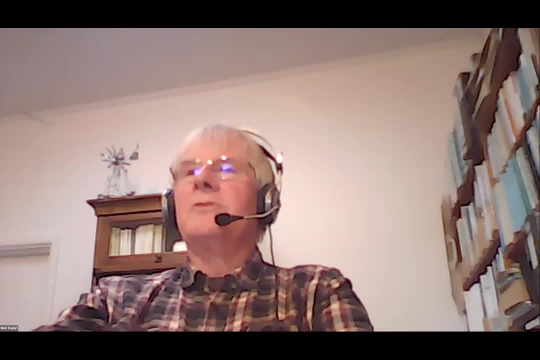 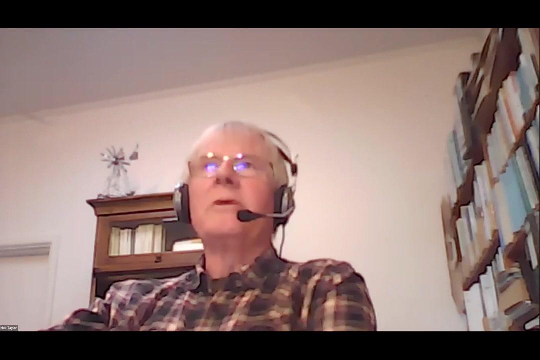 and land available for housing. And, as you point out, that's the Nicholas, that's the, you know. you see that encroachment happening around the roads around the coast and as the roads and tracks surrounding the waterlands area. 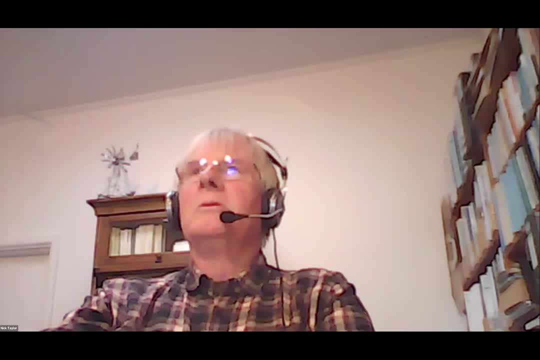 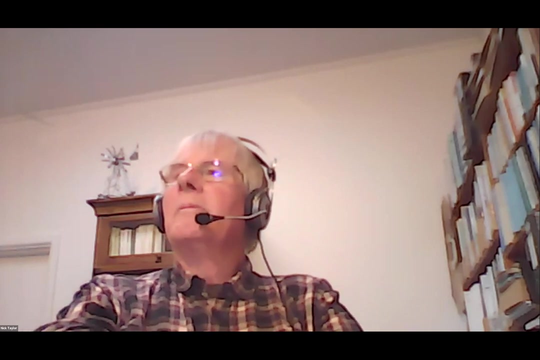 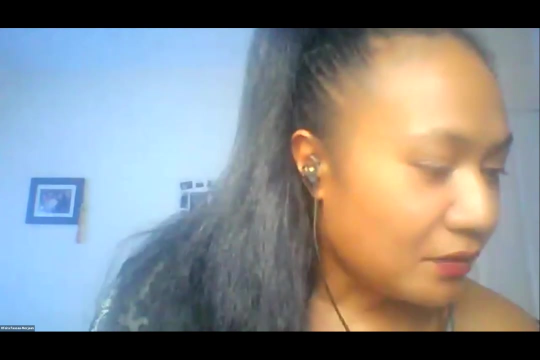 then you know there's been the encroachment with no clear sort of mechanism in place. I guess, unless someone wants to point it out in the group, to kind of constrain that, We have a question here in the chat box. please, Professors. 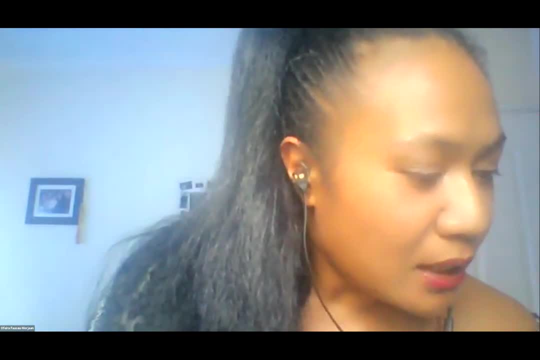 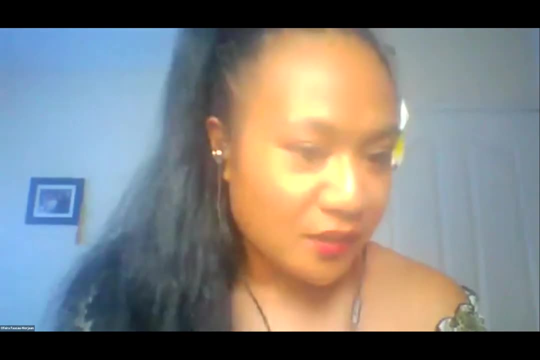 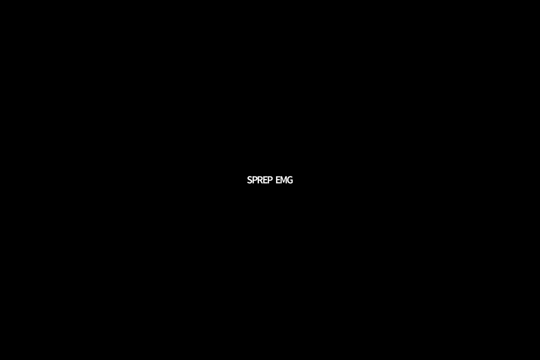 From. she asks: how about others like technology, internet use and receptivity? I'm assuming she's referring to the cumulative impact. So what time is that question? I think that question came in while you were talking about wind farms. Wind farms. 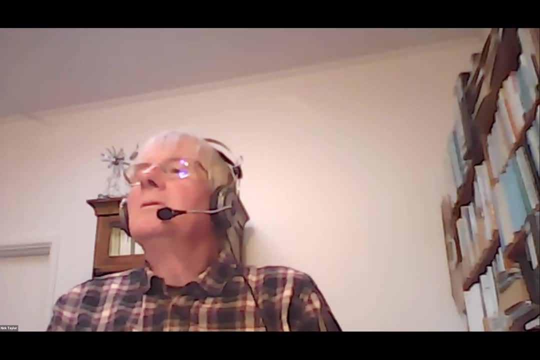 Okay, Yes, So what was the question? Yeah, This is way up. Yeah, Yes, There's like technology, internet use and receptivity Technology, for example, internet use and receptivity. So she's probably referring to the cumulative impacts. 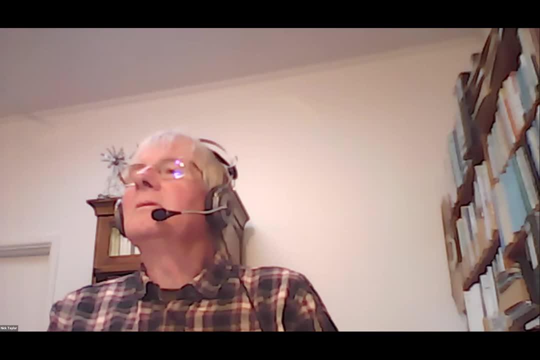 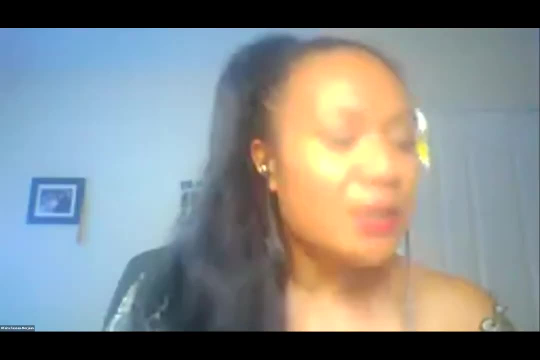 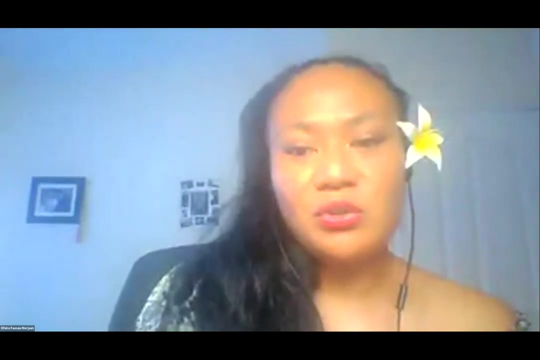 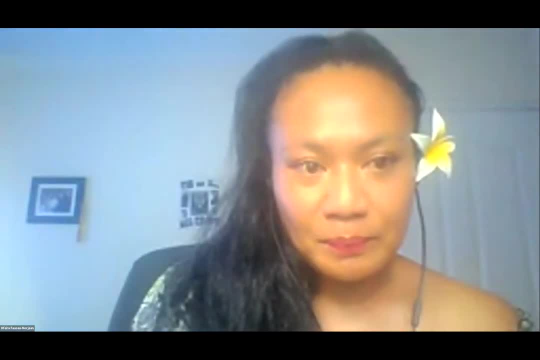 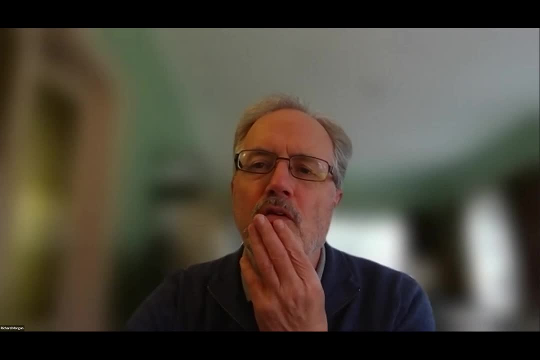 Thank you, Congratulations, You're welcome. Just a follow up. I think I didn't finish. Yeah, You're welcome. Yeah, for your question. Well, Yeah, a big thing in the 1970s and 1980s. 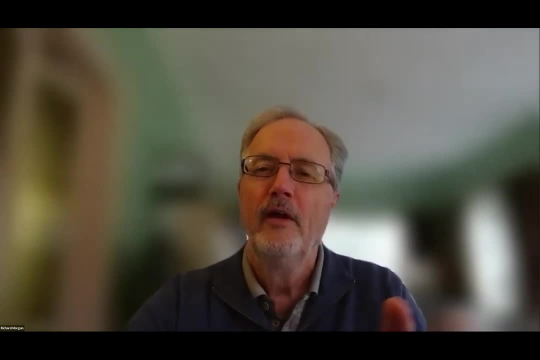 which me and Nick will remember, but no one else here will. But recently, in the last three or four years, there's been a lot more interest in the idea of, if you like, doing impact assessment of technology developments, and certainly from an economic, social. 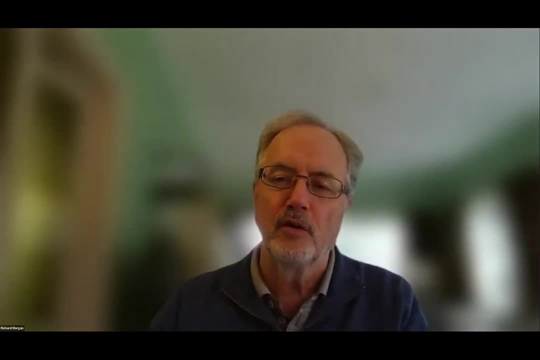 cultural perspective, thinking about future technology development and what it would mean for not just individuals but communities and nations and so on, And that's about all I can say at the moment. I've not really gone into that to any great extent, but there are people who are very aware. 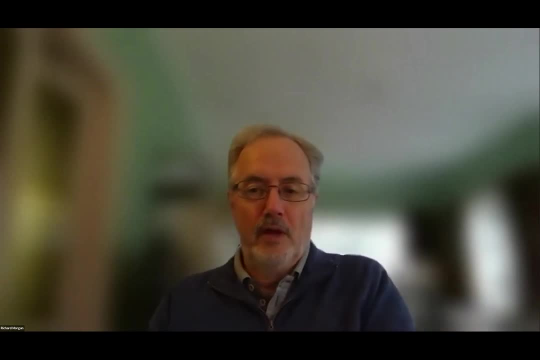 of the potential effects, advantages but also adverse impacts of technology, especially the internet, telecommunications, et cetera, et cetera, how that will change societies, especially small societies, for better or worse around the world. But I'd have to stop and think about what cumulative 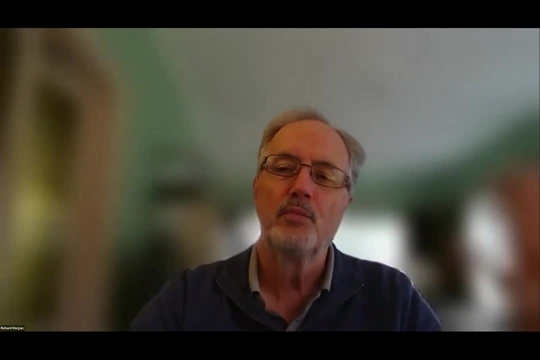 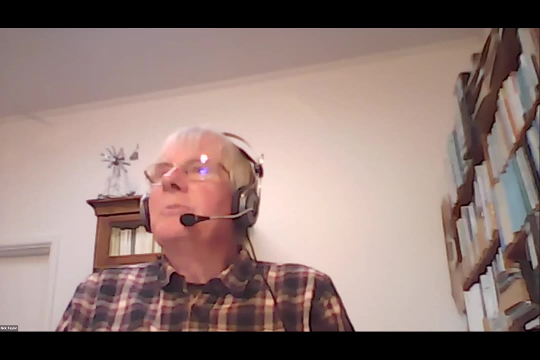 what that might mean for cumulative effects within that sort of broader movement of technology assessment. Yeah, I mean I don't see the principle of a cumulative effect would apply with outside of an environmental setting. I don't have a problem with that, Certainly from the point of view of social impacts. 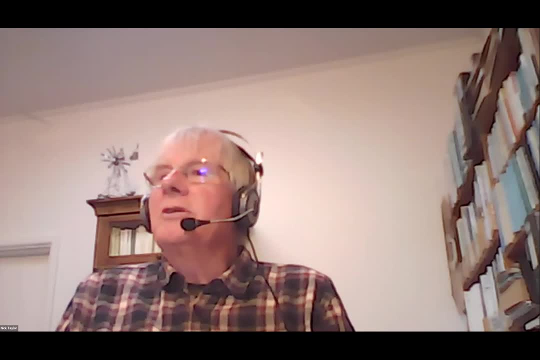 they can be studied in relation to any set of planned or unplanned changes. So I don't have a problem looking at, you know, looking at technological change from that point of view, I think it's a good thing to do. Might come under another ambit or another part. 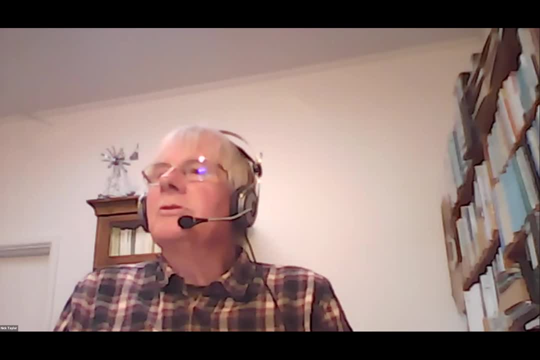 of policy development within a government, for instance. Thanks, thanks, I agree. Is that you Greg? Yeah, it's me, Nick. At 2.07,. just while you're on, at 2.07,, Margaret put in an interesting question. 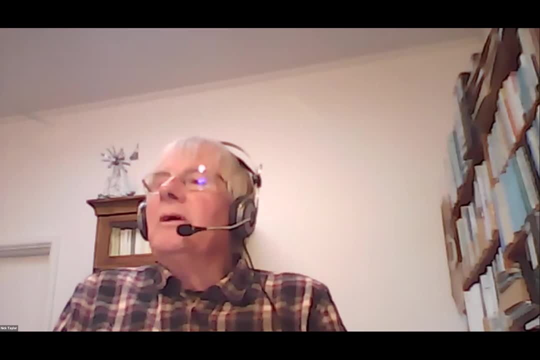 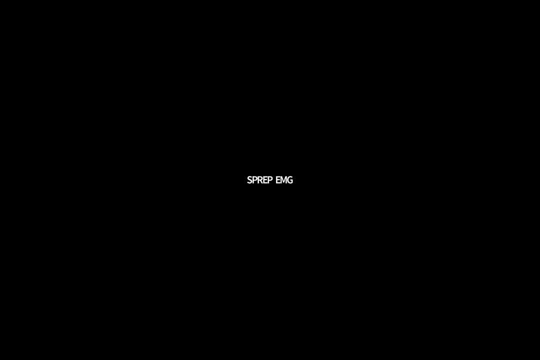 about practitioner, recognition of practitioners in the field and ways to develop and improve guidelines, which I think probably falls more into the SPREP bucket. Yeah, so she's also put another question. There's another question that Margaret's just come in, so I'm just going to go back to that old one. 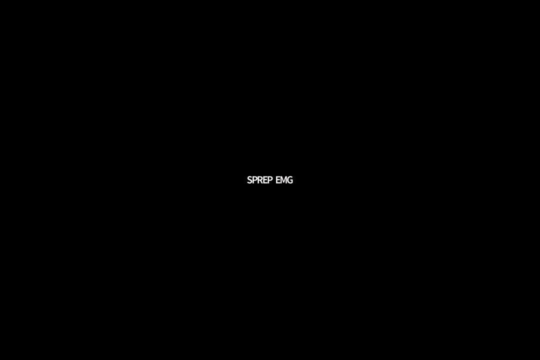 But there's so many questions keep popping up it's hard to track back to that one. Yeah, it is So. yeah, as regards to guidelines, well, yeah, that's something we're constantly working on and trying to assist countries. 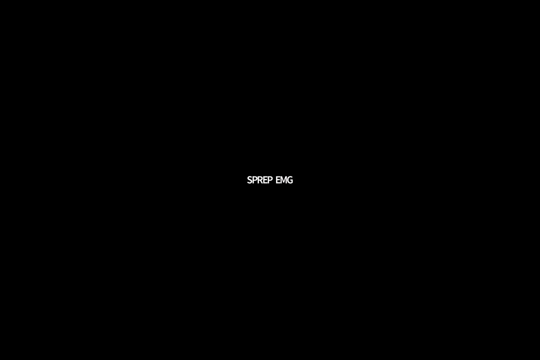 with development. They're developing up their own sets of guidelines when they ask for them to align with their regulations. And then there was the question in regards to- I guess if she's talking about accreditation or recognition, it depends. It depends on which side of the- what that specifically means. 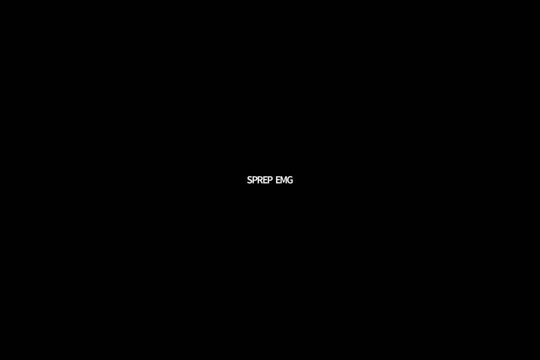 Like we're looking about getting guidelines formalised and approved and that's a government process. We're talking about getting you know accreditation for skill sets. that's a qualifications matter. So yeah, I can't see the actual question. 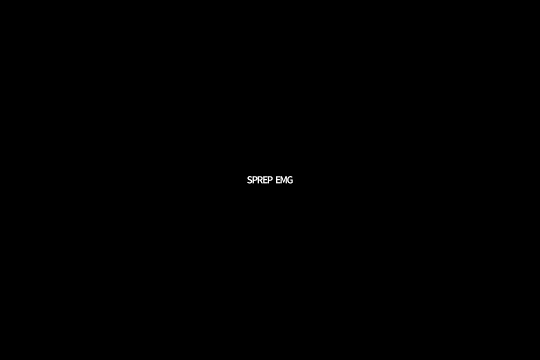 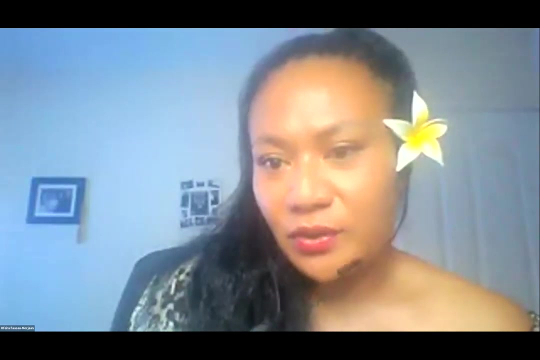 so it's difficult for me to know if I'm missing the point. Just trying to track back, Greg. I also replied to Margaret that I think our question will be suitable for our session next week on accreditation. Maybe we can discuss more about that. 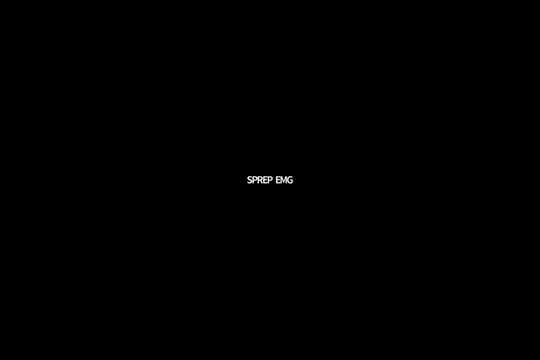 Yeah, I was wondering if that's what she meant As well, Because we do have Lockie going to be presenting on accreditation and different schemes. There's another question, though, that Margaret has posted about. can we please share an example of strategic regulatory change as a result? 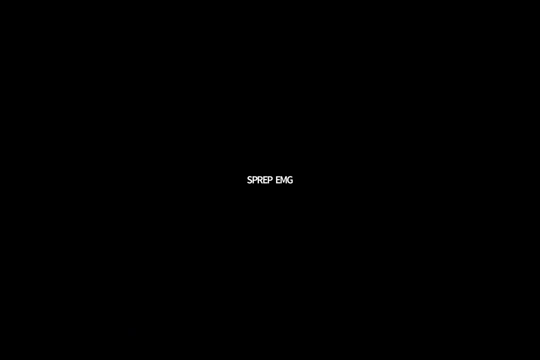 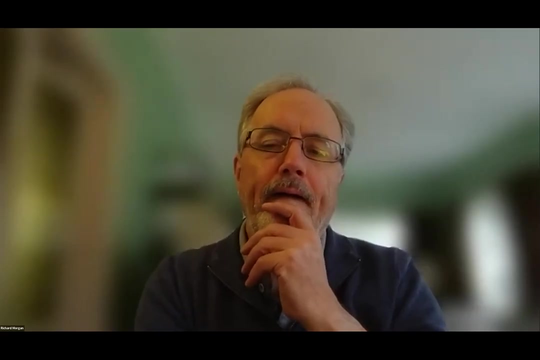 of a cumulative impact assessment. So I guess that would fall under the SEA branch- of how you use cumulative assessment to look at a policy plan. So, Richard Nick, do we have an example from you, a really good example, probably from Canada? 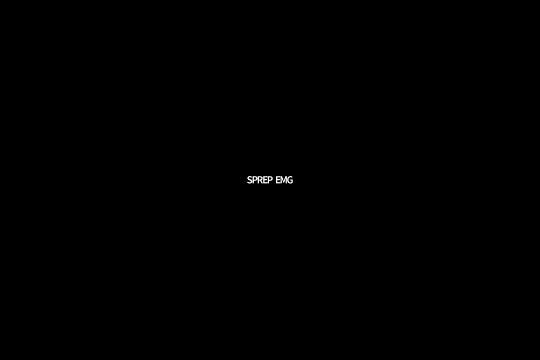 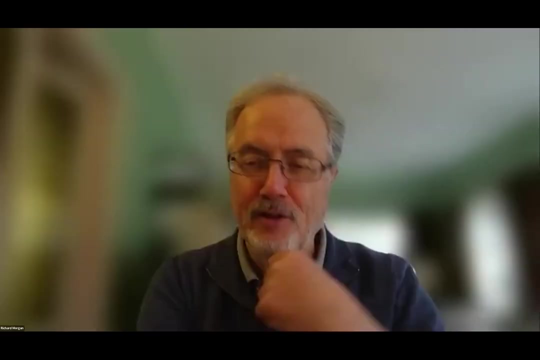 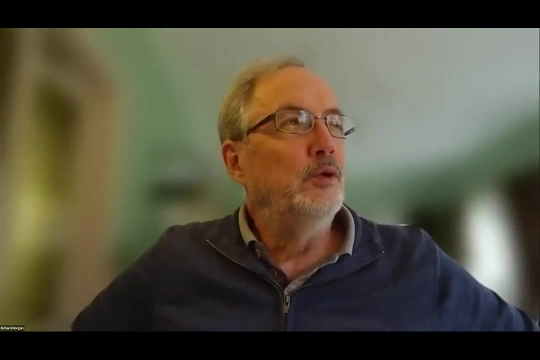 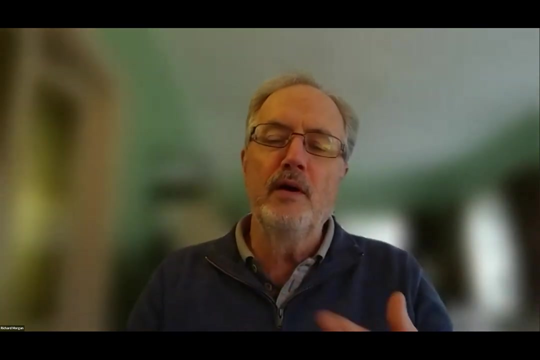 of where that has been applied. Actually, I've got a Kiwi one, Okay, For a change. And it may not be formally known as strategic assessment, but what about 15,? just over 15 years ago, there was a marine farms were. 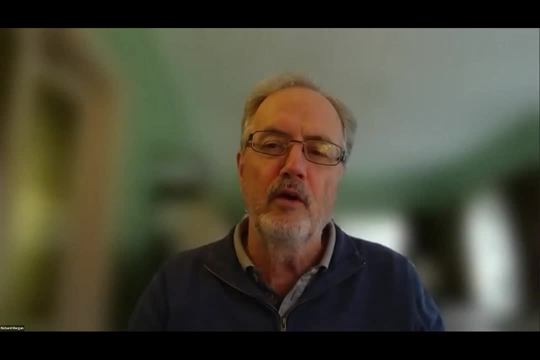 were really spreading very quickly around the coast of New Zealand, especially in certain areas where the fields are, And people were getting really worried that we were getting that traditional project by project- expansion of marine farms- And that no one was really looking at. you know. 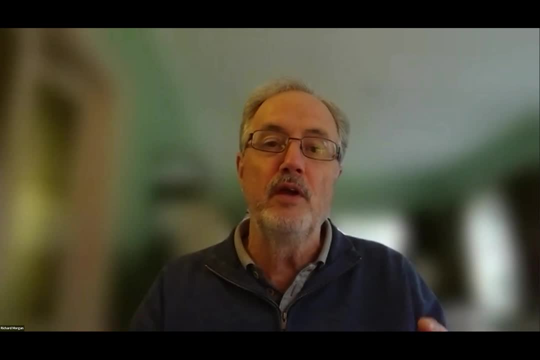 what the, the, the overall effect of that might be, especially in areas, big embayments, where they were filling up with different types of marine farms And there was no real overview of what the cumulative effect would be. So government of the day instituted a moratorium on consenting fish. 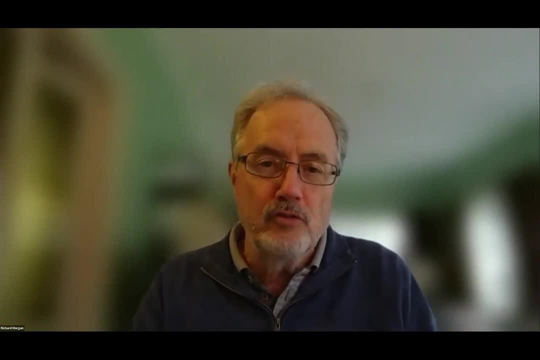 farms. So, and they were really, they were really, they were really really good at it And they actually said to the regional councils who are the ones who authorize these. They said: all regional councils have to stop Processing fish farm applications until you've got a. 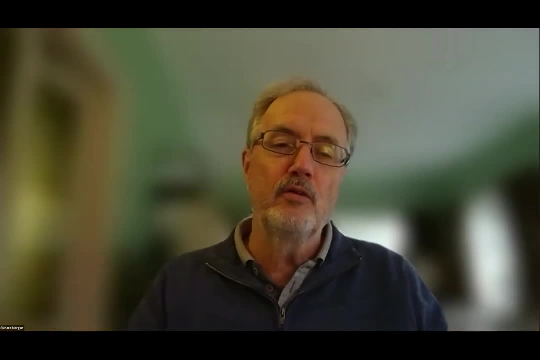 a plan for your area And that required the councils then to That had these applications To look at the Number of Marine farm operations, Look at the capacity of the Marine area To sustain Farms without adverse effects, And then introduce some sort of regulatory process. 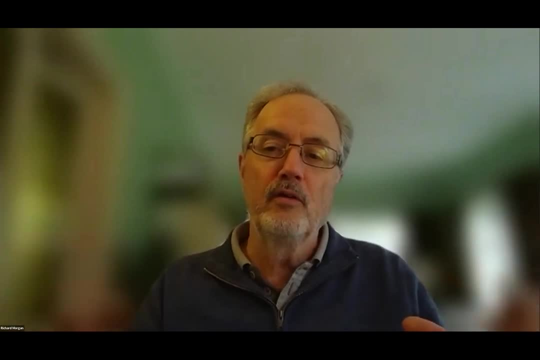 To deal with Fresh applications areas and then opening the door and saying: well, we can accept more farms as long as they're within a certain you know, certain number, of certain type, and therefore we, we are managing the cumulative effects in that way. 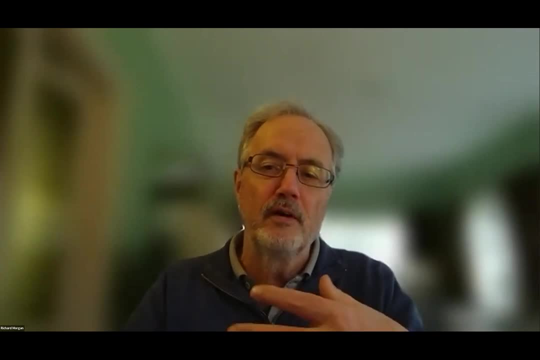 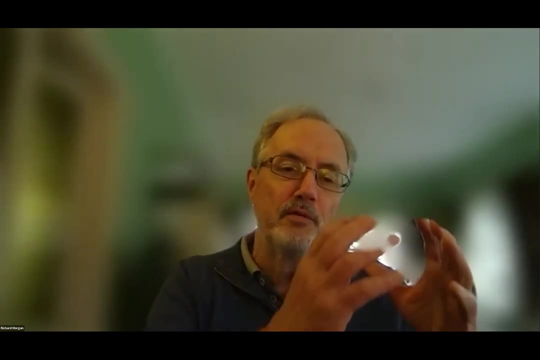 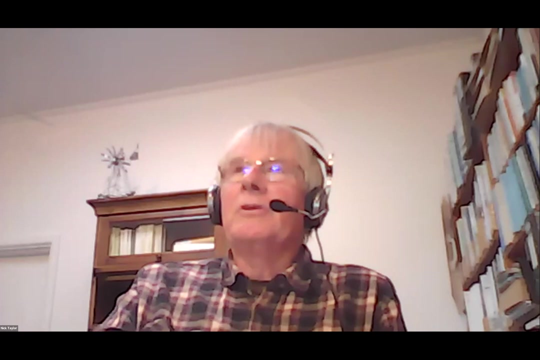 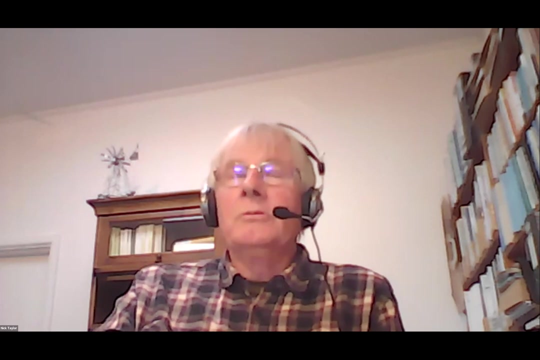 And that for me was always, has always been, one of the better examples of a regulatory response stimulated by a growing problem of incremental sort of growth in a sector like that. If I could just add to that, Richard, too that- and a good example out of that was a council like Marlborough District Council that put in place rules and rules and policies. 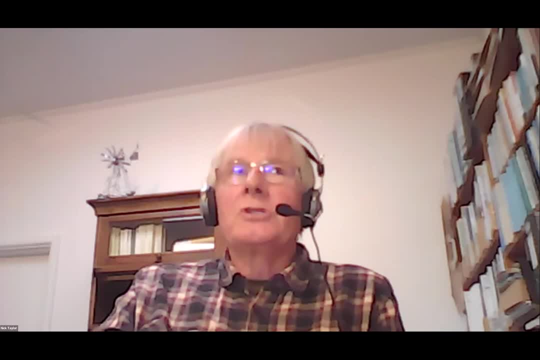 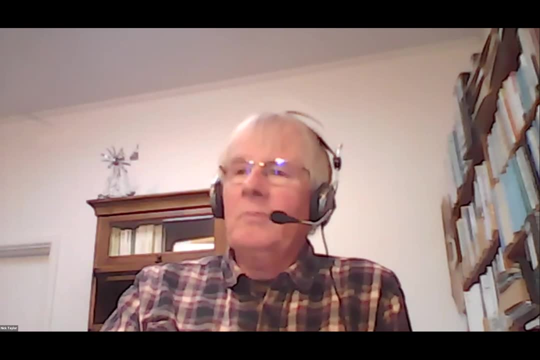 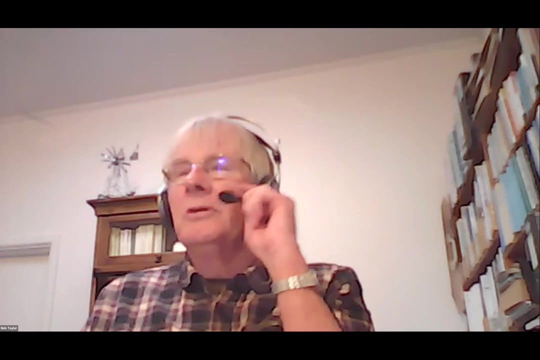 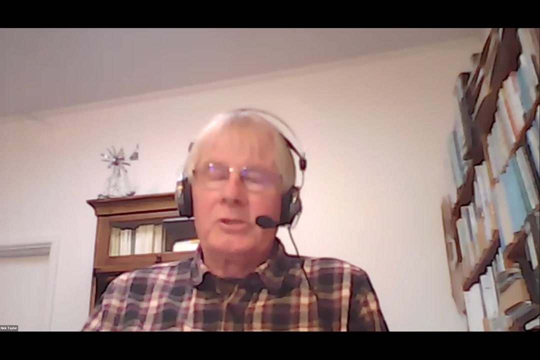 and rules in their plan And then they were challenged in the Environment Court because people still wanted to- excuse me, go outside of those rules, And that actually has led to some serious analysis of cumulative effects relating to individual proposals for new marine farms. so I'm talking about effects on, for instance, benthic fauna and ecology. 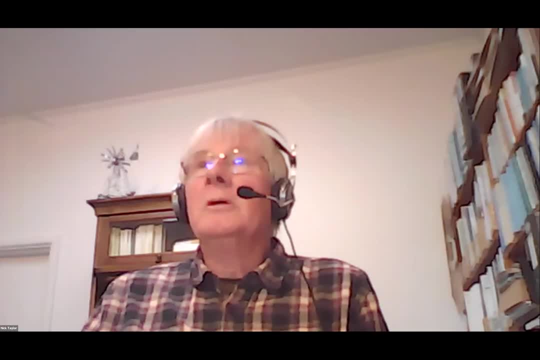 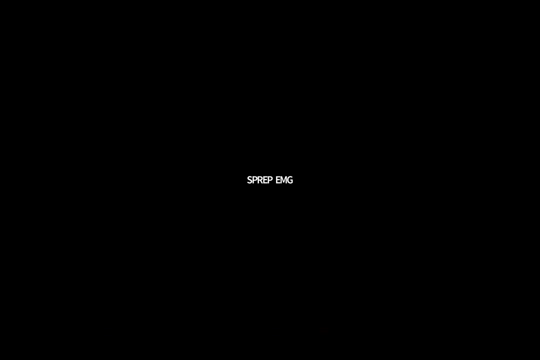 on on visual effects, navigation effects, recreational boating effects, commercial fishing effects, all of those things have you know, and now, I think, looked at much more thoroughly, I think, yeah, that's a really good example you brought up, Richard. 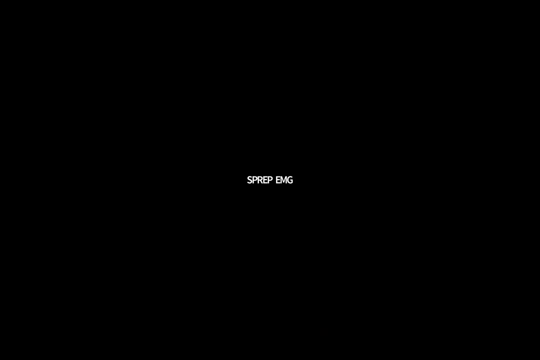 I think it's one that's probably played out across the globe multiple times with essentially industrial scale aquaculture but run by multiple operators. I don't know if any of you have heard that, but actually this is a really interesting thing that I did do- and I think I mentioned this earlier- and that is when I was working in Scotland, and that's when the system collapsed, basically through disease was. 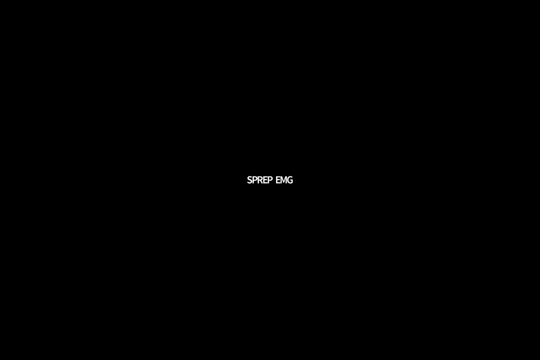 happened when I was working in Scotland and that's when their system collapsed Basically through disease, was the same thing to look at the cumulative impacts and have come up with the area management agreements and stopped all work. and Chile went through a similar thing about 1012 years ago, and then Australia has just been doing it, probably about six to seven years ago in Tasmania. so every time, unfortunately. 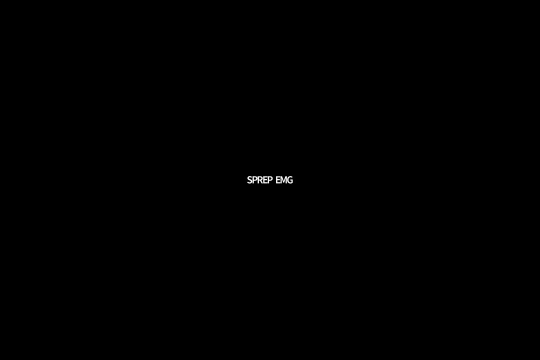 included in assessments for projects or any developments. um, i got one which was when we were starting to do a whole wave of new ports in south australia. they had a whole heap of ideas of new ports and again in wa with the iron ore boom that was happening. 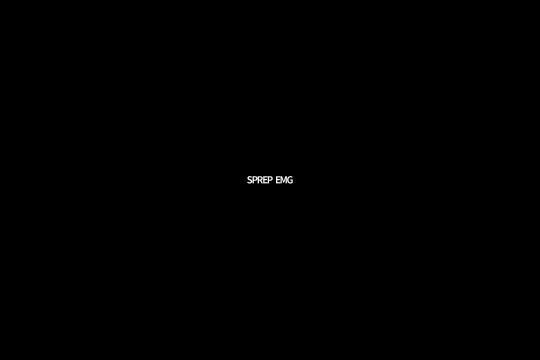 about five, six years ago, there was a lot of new ports coming online or proposed to be coming online, so we had to start implementing cumulative impact assessments to look at what the impact of having multiple ports operating would be as opposed to what had previously been there, which 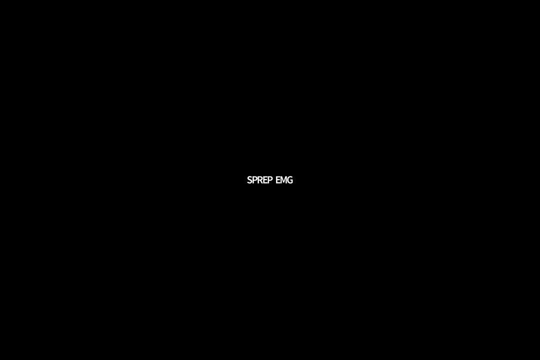 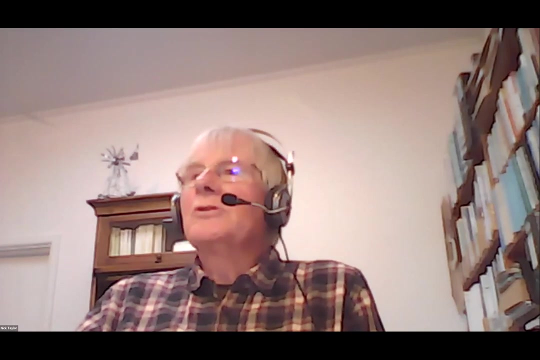 was maybe one or two ports and a few discharge points. so cumulative impact started being triggered by the, by the regulators. then, within australia, and the state regulate regulators but, um, within an island setting, i guess that's going to be up to the regulators to decide. i i think we should say here too that, um, it's not quite not a question of saying: 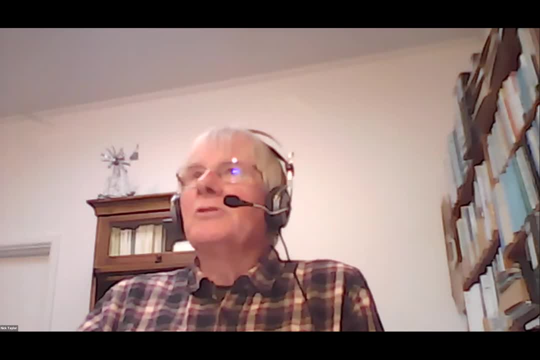 when should we? you know what? what doesn't require cia? i would say, turn it around and say: every impact assessment. cumulative effects is something you should look at in any environmental assessment, unless there's a good reason not to now. i think we should be assuming that a cumulative effect 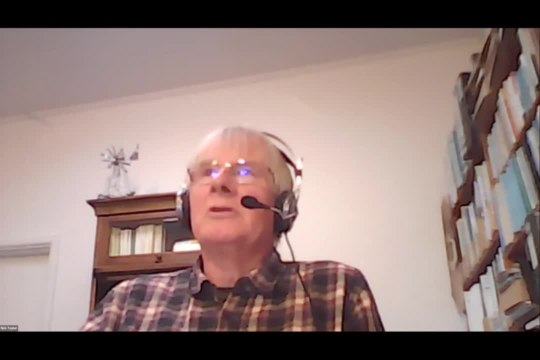 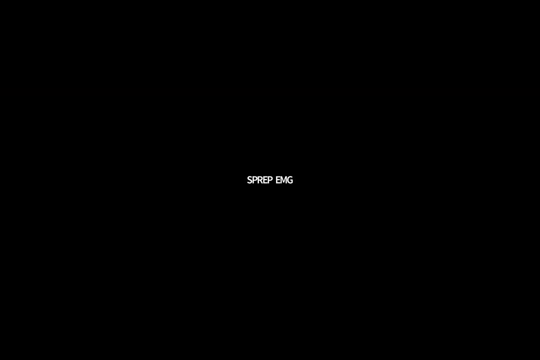 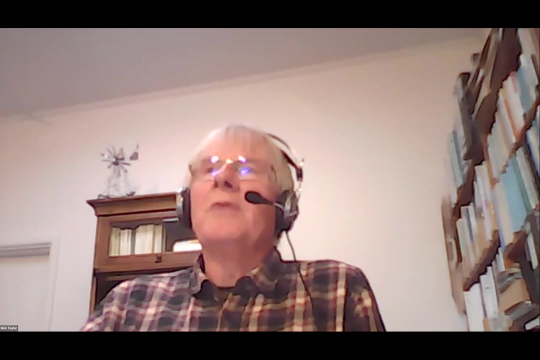 is a normal effect. it's something that is very common and if you look at most projects or even most um strategic assessments, particularly strategic at a strategic level- but i would be- i would think you'd most of the time you'll find some sort of cumulative effect if you. 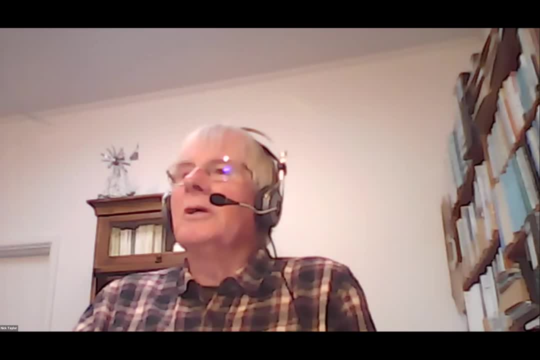 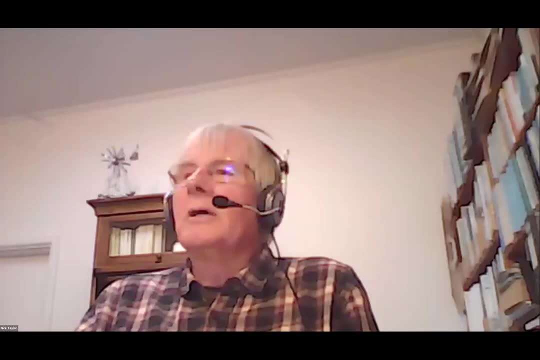 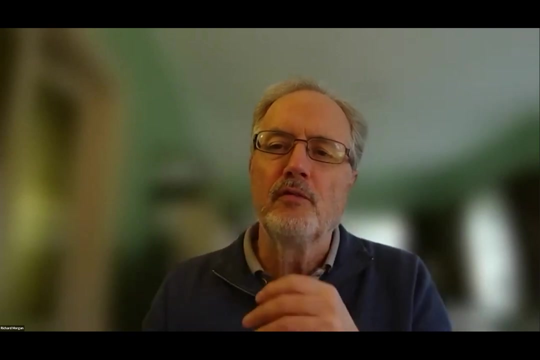 start looking for them, and it's just not something we've sufficiently um considered. i see there's a question about aggregate queries. do you want me to answer that now, before you do that? the question from marista there is: um is cumulative assessment required even for small scale projects, and i think that follows on from what you've just said. 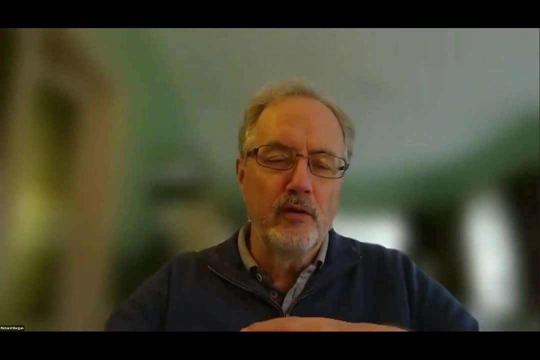 um, that we're not talking about necessarily doing full-blown area-wide, resource-wide assessments when we're coming in at the project level, but we always, whatever size the project is, as we go through the analysis. one thing we need to be aware of is the wider context, so even our. 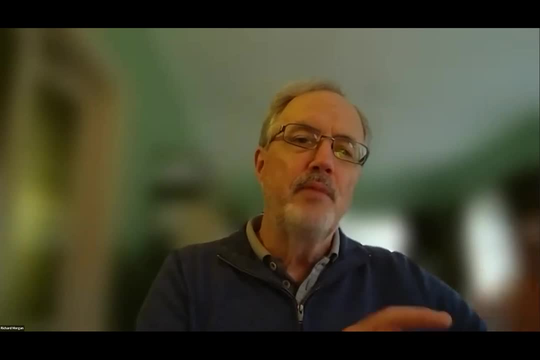 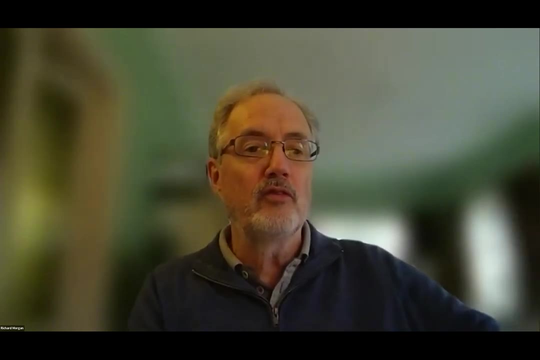 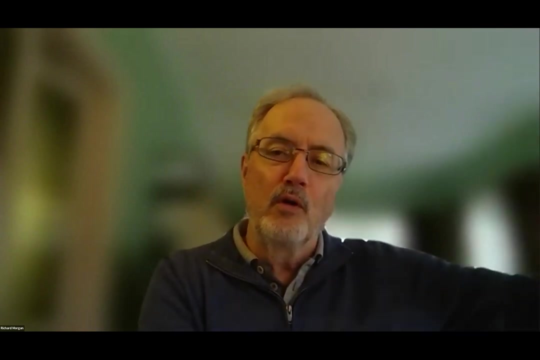 what look like smaller impacts. when we look, if we scan around the broader context, we might recognize that they're actually quite significant. um, you know, we might be affecting that rather rare species and and when we look around the wider context, uh realize that this is the only place that 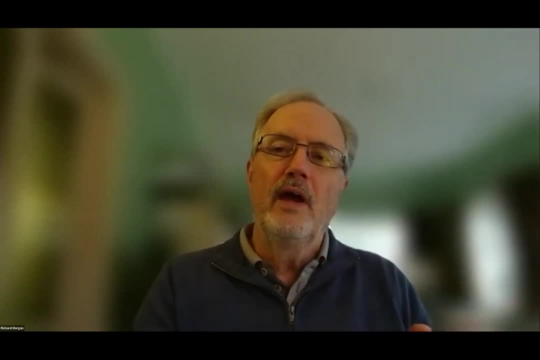 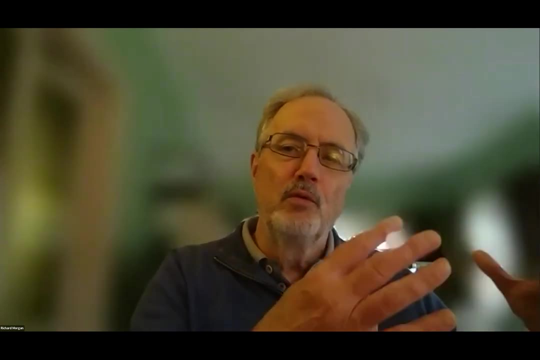 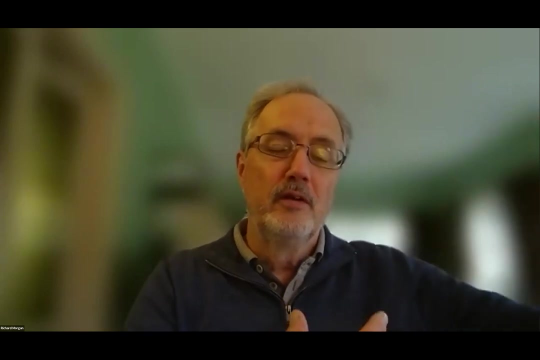 species occurs. so we've always got to have, uh, some sort of recognition of the wider context, but it doesn't mean we have to do a full-blown big production number every time, and it may be that we we have to alert the authorities to a bigger issue whilst we confine ourselves to managing our 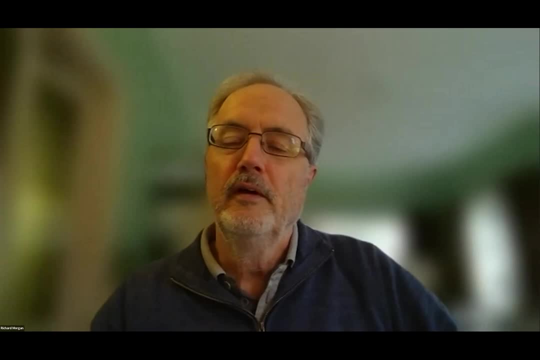 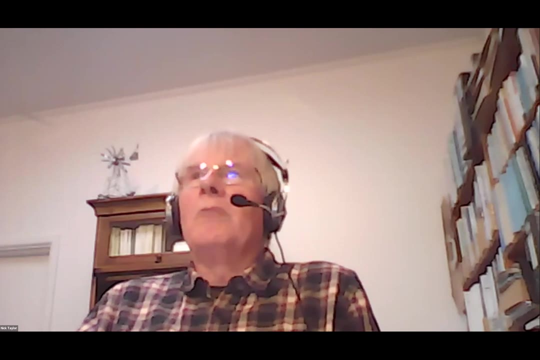 project and our mitigation as best we can? i think so, and waterfront development is a classic example of that, where you get, you know, if you one project on its own might have not a great impact on the coastal environment, but then you add another one, and another one, and another one, and 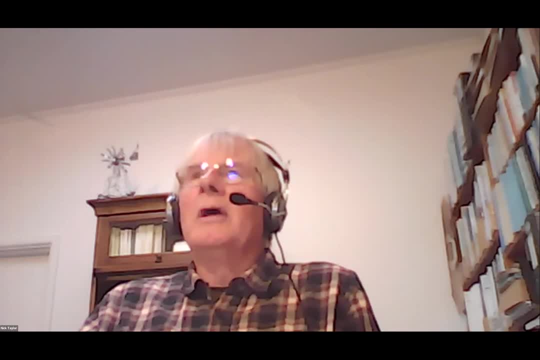 every island group. i'm sure you and and certainly all around new zealand as well, you will be aware of the impact that that accumulated sets of development is having. yeah, um, it's classic tourism. i mean, tourism is another classic one where the individual projects don't seem that big, but when you put them all together, 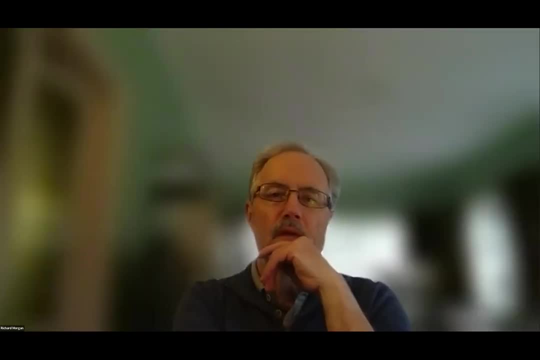 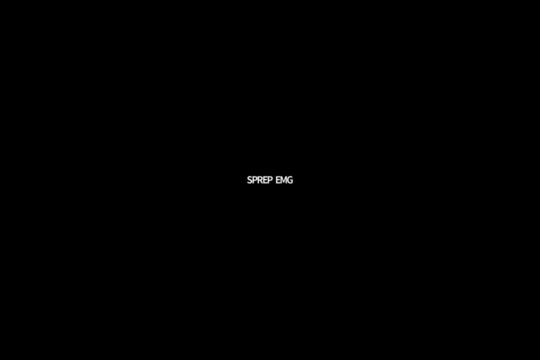 yeah, um, thanks richard and nick. um, i guess, yeah, those those little those examples are of, yeah, cumulative impacts and i think, in the pacific context, on the small islands and for the smaller projects, um putting it into context of what things to think about in the toolkit of 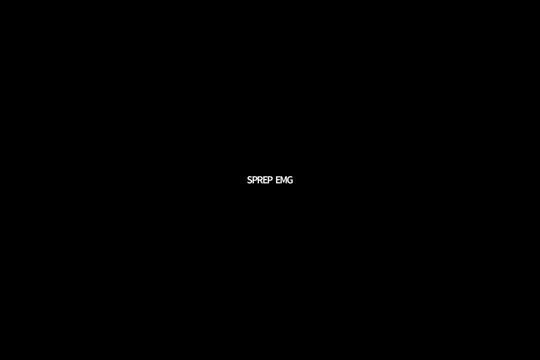 what is a cumulative impact is water, especially for the atoll countries. it's the impacts on the water resources, either, albeit long term, or even just during construction. so one of the things we always talk about when we're helping the um- the regulators look at a project- is: where are they going to get the water and the aggregate for to construct? 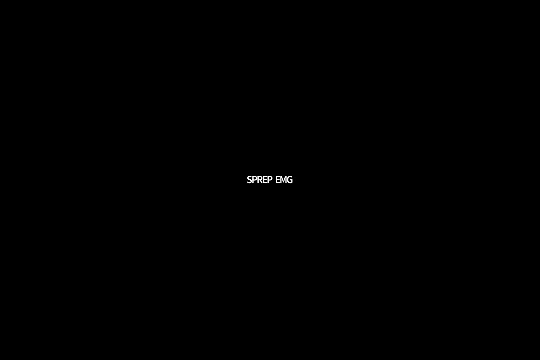 the facility that that's planning on being built. if they're going to be mixing concrete, they have to be usually taking water from somewhere, so how do they manage the water? so that's one of the things we constantly get them to think about beyond the project footprint is: where is the water coming from and where is the aggregate coming from? and 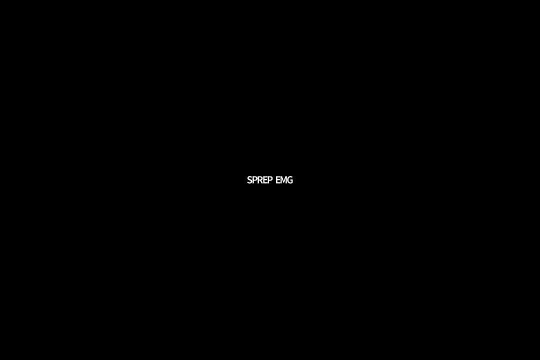 how are they going to deal with that? because, um, that's a, that's a cumulative impact across that, that small country, and where are they going to bring that resource from and how is it going to impact them going forward? so we, yes, cumulative impacts are something that 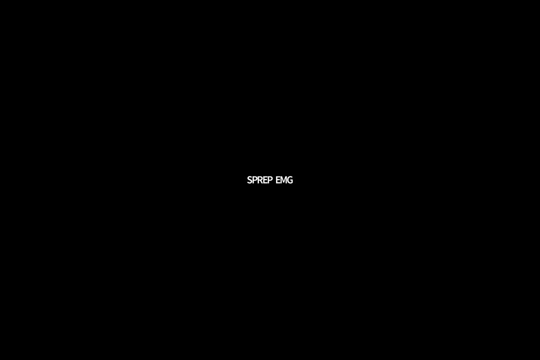 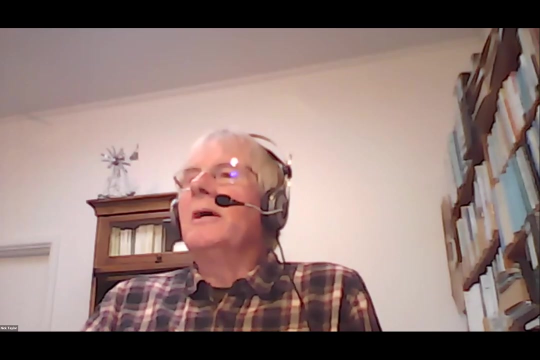 have to continually think about, even on small projects, but they don't necessarily have to do a full-blown impact assessment specifically for cumulative impacts. it's just think about the broader picture. just quickly answering that aggregate one, because there's an interesting aspect to this um the. the case i was talking about was a um decision by an environment court. so whilst 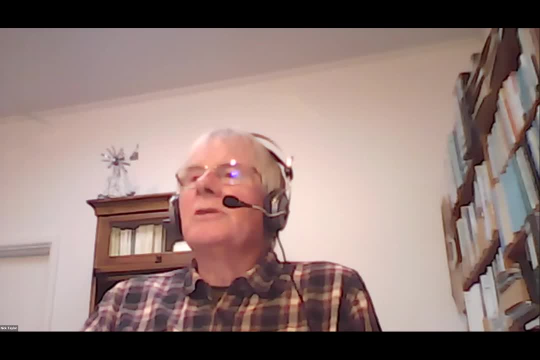 it didn't necessarily lead to a legislative change. it led to a legal precedent under the act- the resource management act- that manages these things, um. so, in effect, um, future judges or decision makers would have to have this kind of a decision about what to do and how. 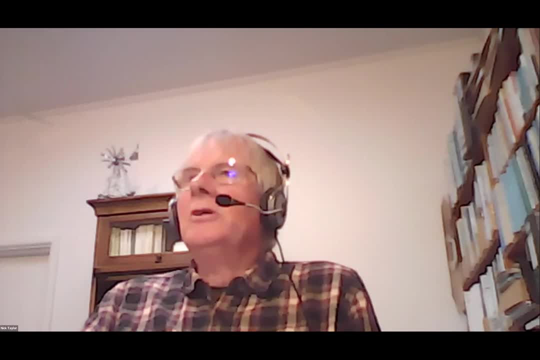 have to take account of the fact that this judge has clarified some issues around what is a cumulative effect and how it should be considered. so you know all of that does add into the legislative framework and also the district council has since revised their plan. anyway, they were that's a regular process, that they do that and I understand there are some new rules about. 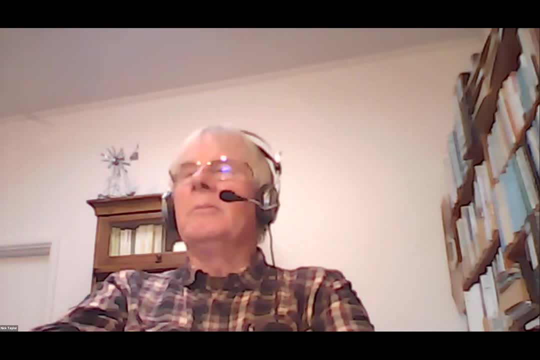 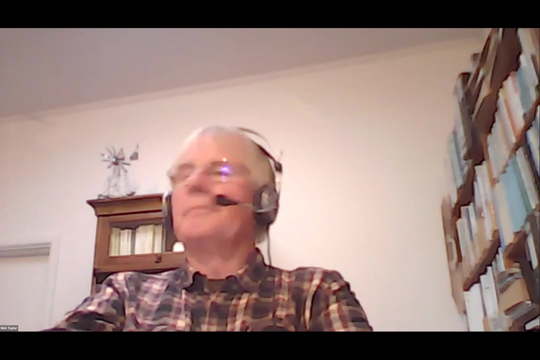 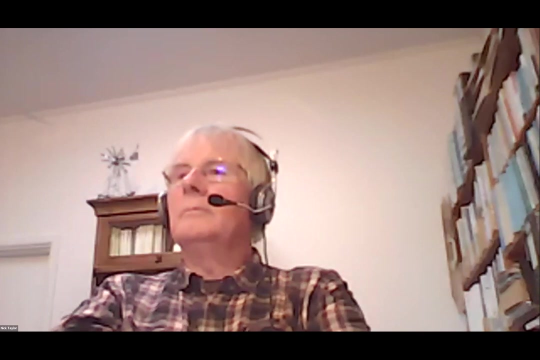 quarries, but I'm I would need to go back and check them, but I'm pretty sure they now institute some rules around distances of the quarry boundary from residential properties, but I'd need to check that. I guess we don't have any more questions. I think that's the last question we have in our 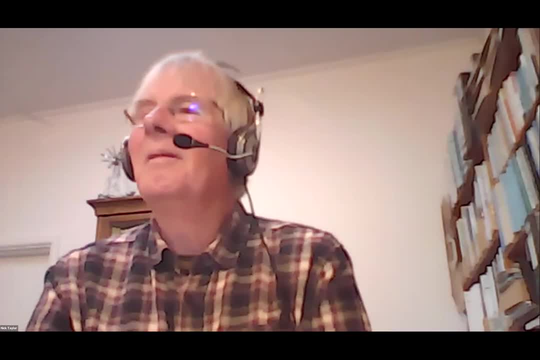 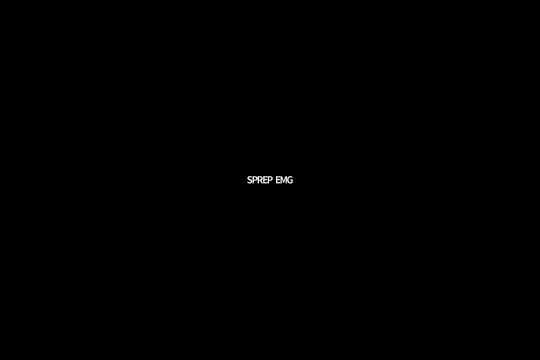 chat box. Greg, how are we doing with time? we have gone over our time, we have gone over, but you know that's a good sign. it's, it's a, it's a healthy conversation. I did see that Rachel had to leave and she has asked that. everybody who 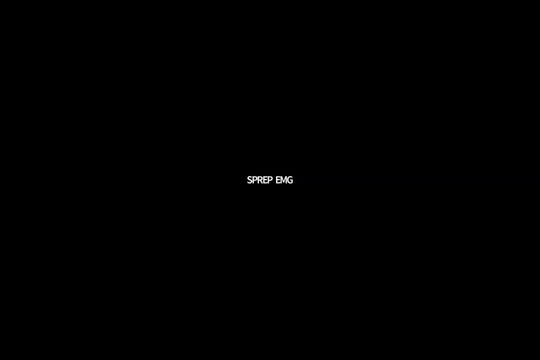 has participated in today's meeting, that they use the link to or follow the links that are emailed out, either in this chat or in the emails that we'll send out later to respond to how you thought this actual presentation went, and you know. please answer those questions, because it really helps us. 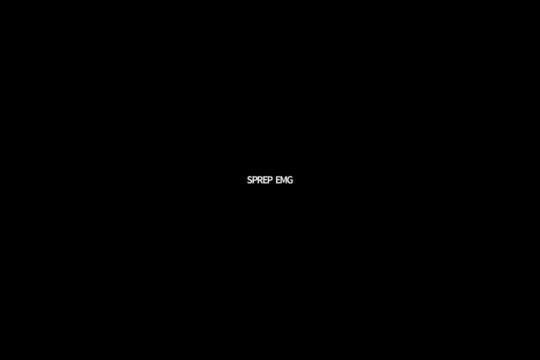 to make and plan better presentations for future sessions. but yeah, unfortunately we're going to have to wrap this one up because the the actual link for the zoom only runs for about two hours max. we can extend. but I'll have to go in and do that. yes, 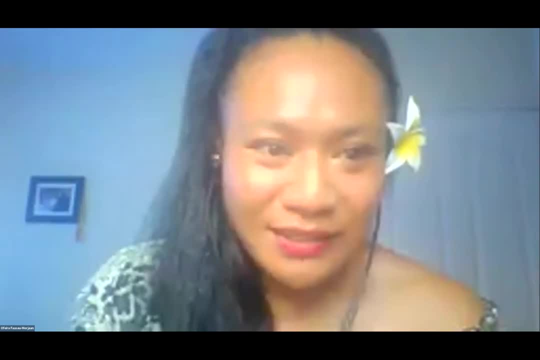 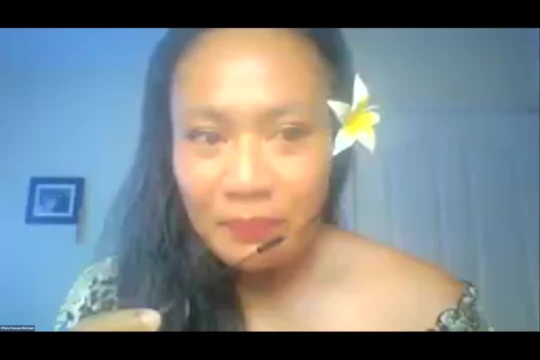 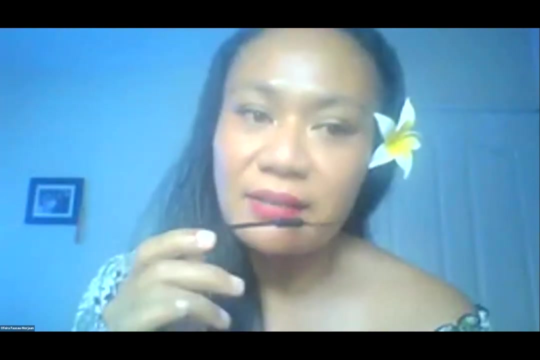 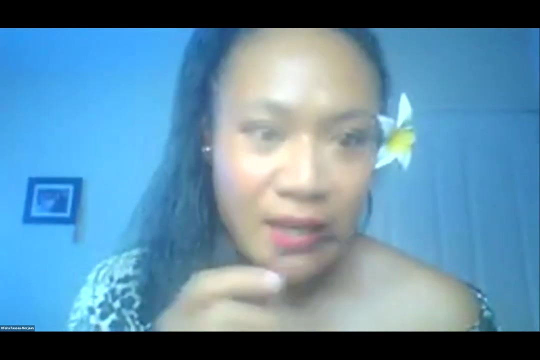 yes, unfortunately we'd love to continue this discussion, but we do have a forum on the PNBA portal where you can post some more questions and then perhaps our presenters, professors, can discuss further your questions on the on that portal. but in saying that, I think I will now take the opportunity to. 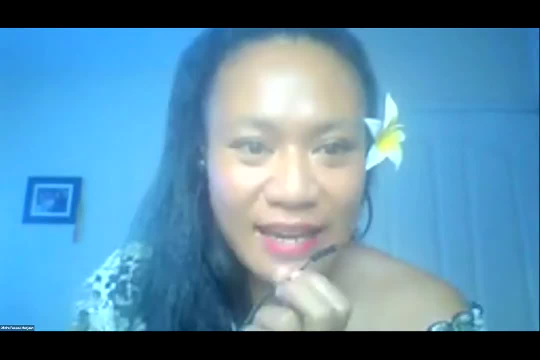 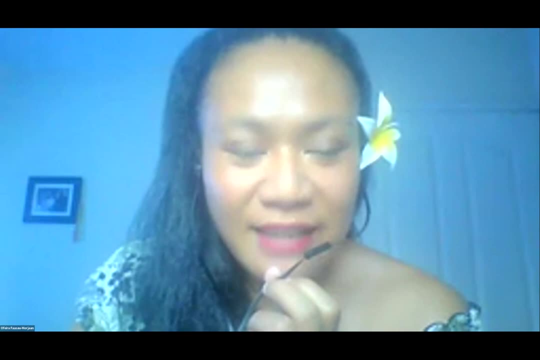 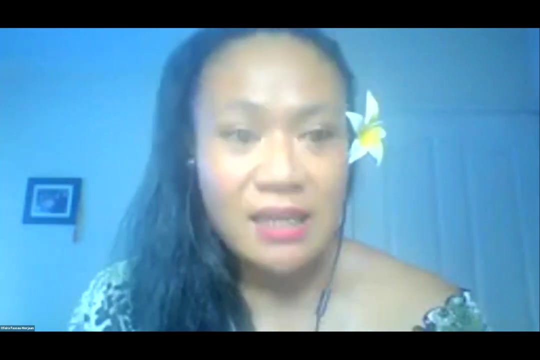 thank everyone who has joined our session today, especially professor Richard and professor Nick. thank you so much for your time. this session has been very helpful for us, especially talking from experience. most of us as well have mostly focused on project-based assessments, but not really on the cumulative, on the resource-based, area-based value component. 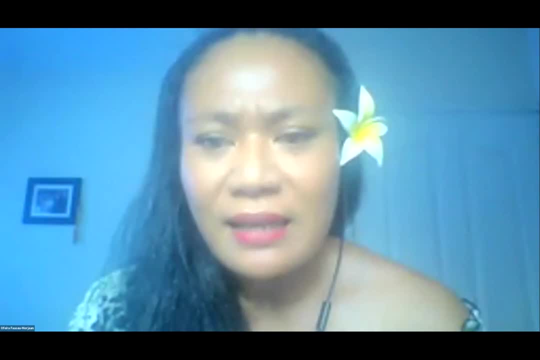 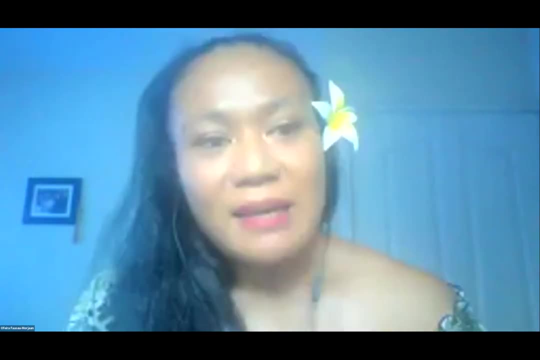 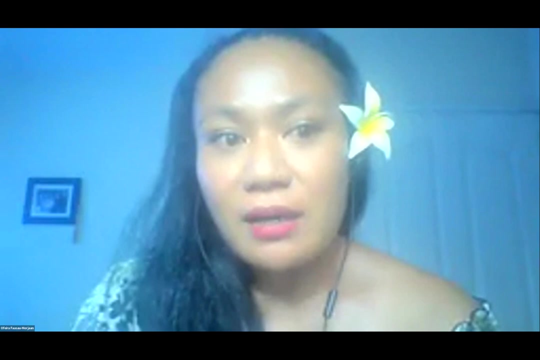 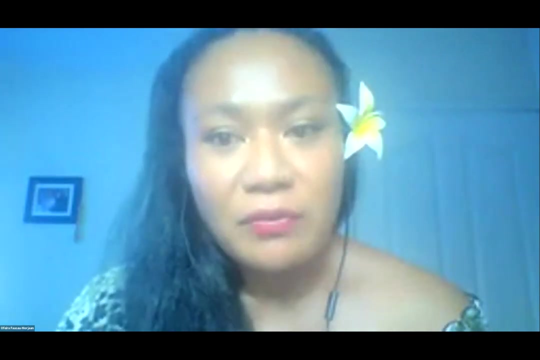 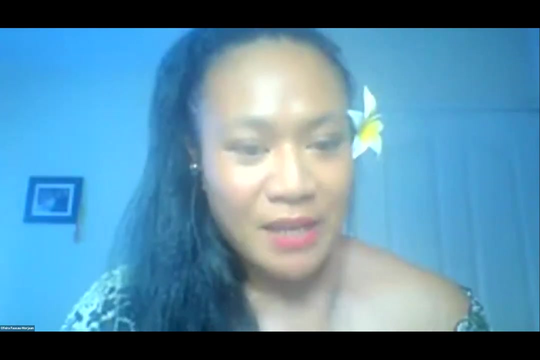 based assessments, and so I think this will be a good starting point into exploring more about this and using this chance to learn more about it and apply it and our work. so thank you very much for your time and for sharing this very valuable knowledge with us, and we do hope that we will have some more of this. 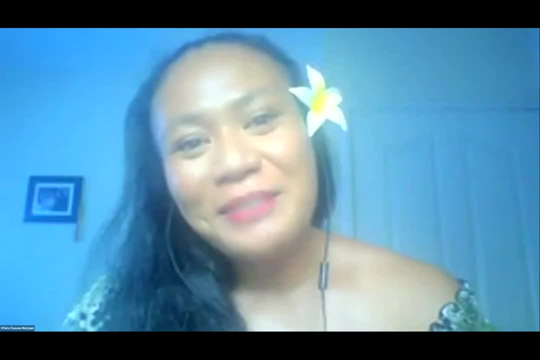 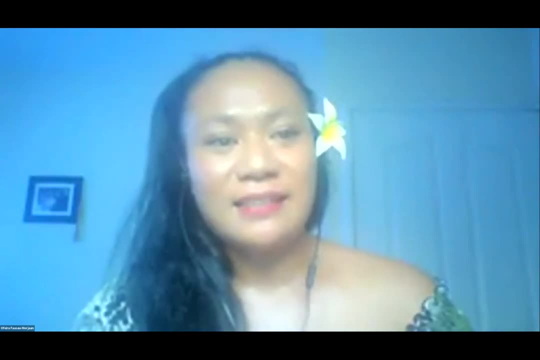 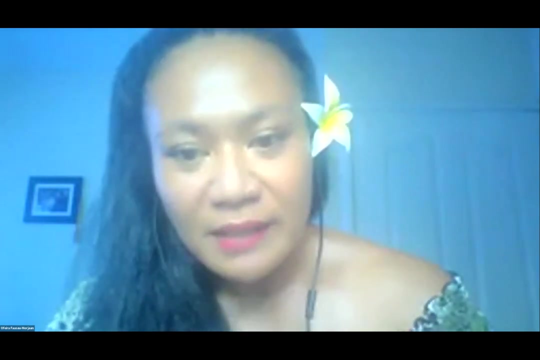 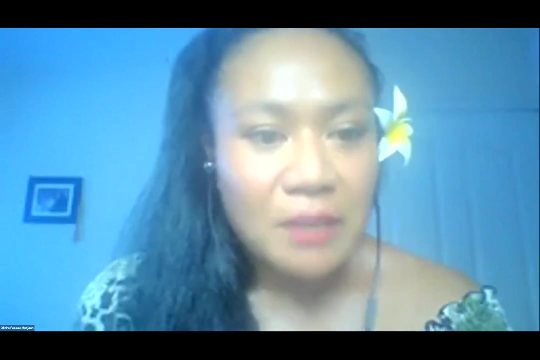 training sessions with you both in the future. thanks, Greg, for for finding some opportunities for that, but yes, so thank you very much. and And just reminding our participants that we have our session next week is on the Certified Environmental Practitioner Schemes, which looks at the Environment Institute of Australia. 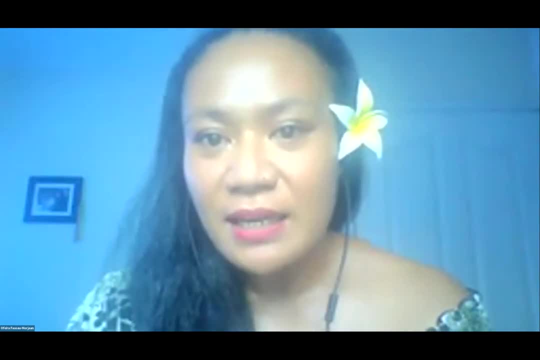 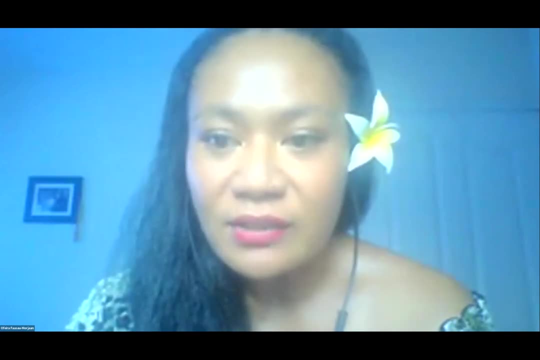 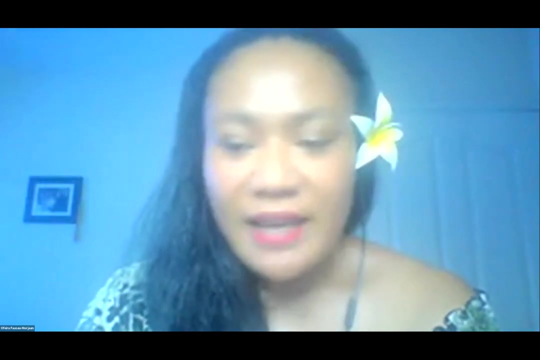 and New Zealand's Qualification Accreditation Scheme. So that will be another interesting topic And we have also a guest speaker on the day. So please tune in And don't forget to fill in your survey forms and submit to us. And yes, so I'll just hand it over to Mr Greg if you could do some closing remarks of Taiti. 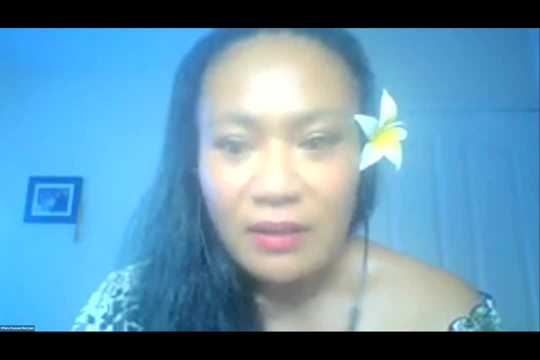 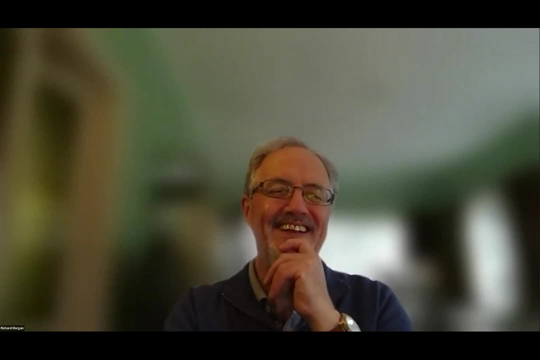 Thank you, Are you there? Are you there, Greg? He's gone. Greg, You there, I'm freezing, Drop back. Can I just say? Hopefully everybody is still able to hear me. I can see if you're happy to leave. 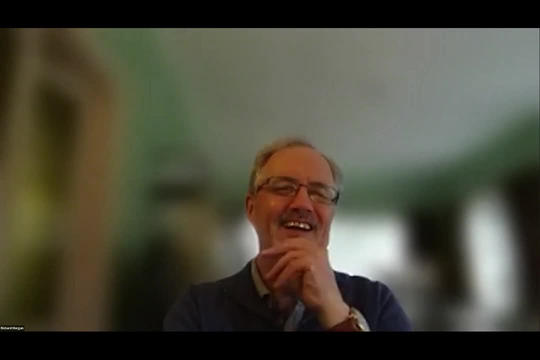 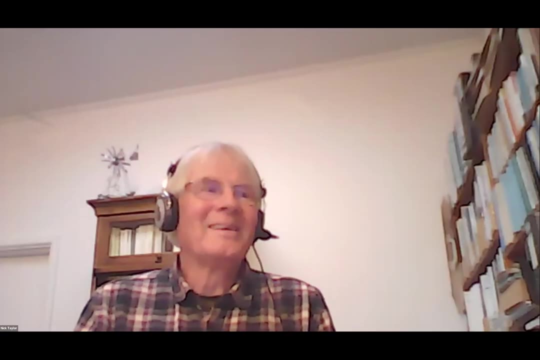 I'm here. Can you hear me? I'm still here. I'm here, Some audio issues. I am here. Oh hi, Greg, Thanks everybody. Professor Richard wanted to say something. Yeah, I was just going to say. 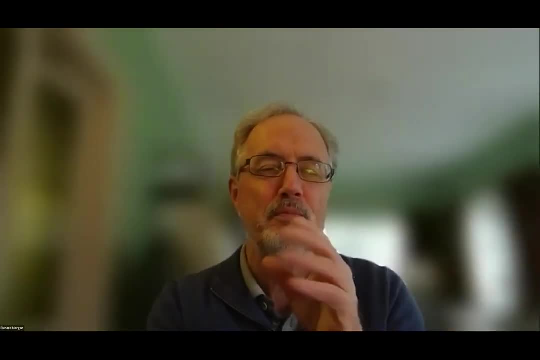 It's been. you know, on behalf of Nick and myself, thank you for the opportunity to talk Great questions And thank you for all those nice messages people are sending through appreciating what we've done. You know, it's always good to have feedback, even at our age, positive feedback like that. 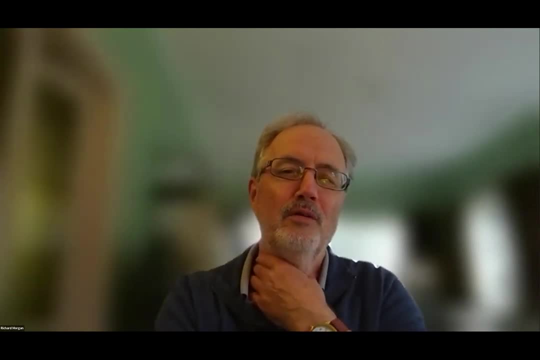 I'm sure we'll get an opportunity to talk again with you all. So take care, everybody Over to you. Greg, We've gone again Me Adelaide back into beyond. Thank you, Sorry about that. Apologies, We have tradesmen on site. 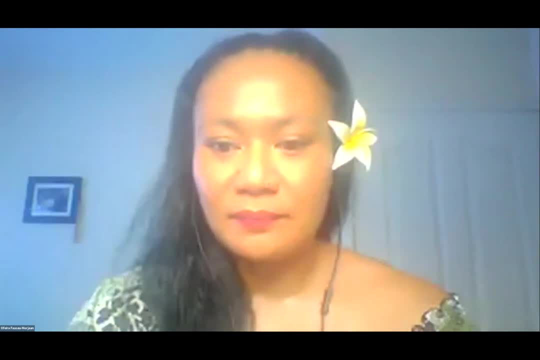 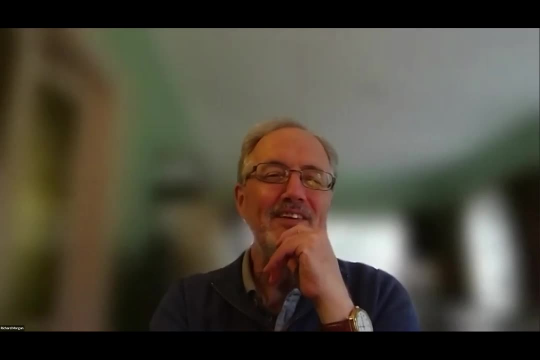 No, I'm still here. Just thank you. It's the light entertainment at the end of this. No, it's not that. Can you hear me now? Yep, We have tradies on site at the moment and they keep interrupting the. 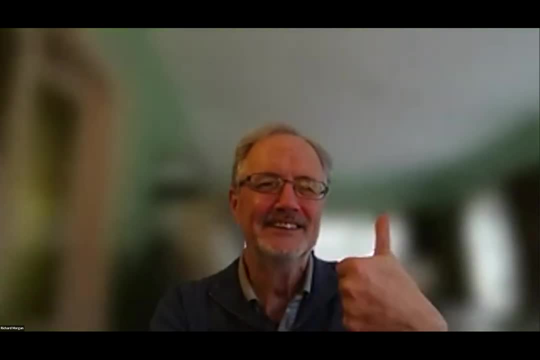 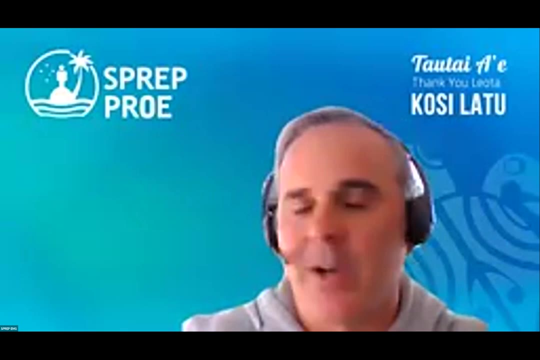 Yeah, It's like this. Can you hear me? Can you hear me? It's a running joke. Yeah, Pulling together those slides and presenting entertaining as always, really informative to, I hope, very relevant for everybody who is listening in. 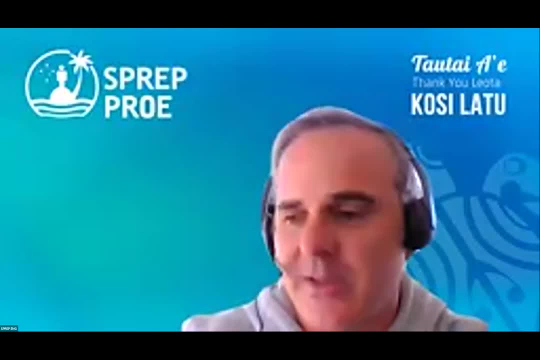 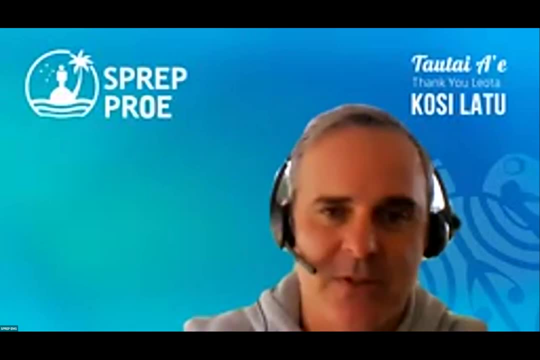 I hope everybody gained something from that And please use those links that Richard provided. They will be really useful. I know he always. He always finds great sources of information, So really I encourage you to go out there and track down extra information. 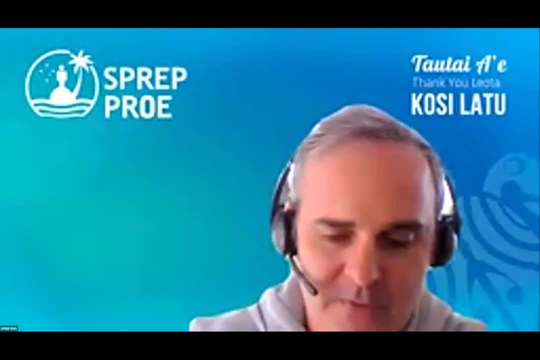 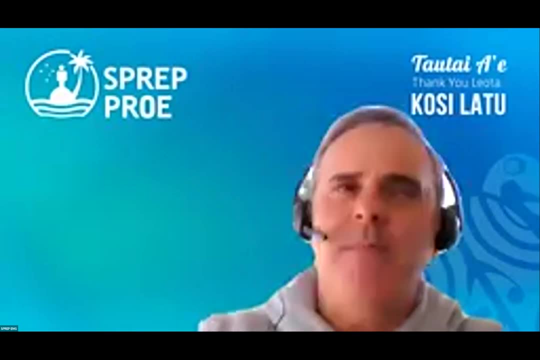 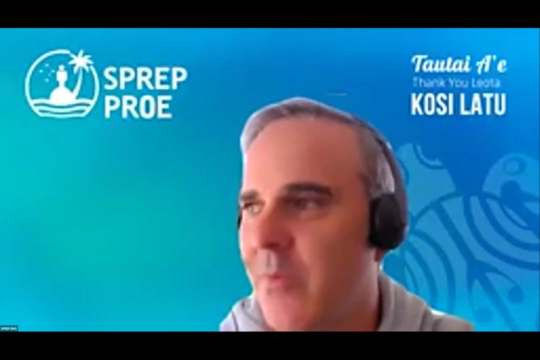 And, as Afera alluded to, we will be continuing conversations on the P&EA chat forum. If you want to post more questions there, Ivan and myself will have a look at them. I'm not sure, Richard and Nick, if you actually are signed up to the P&EA and go in there and check them. 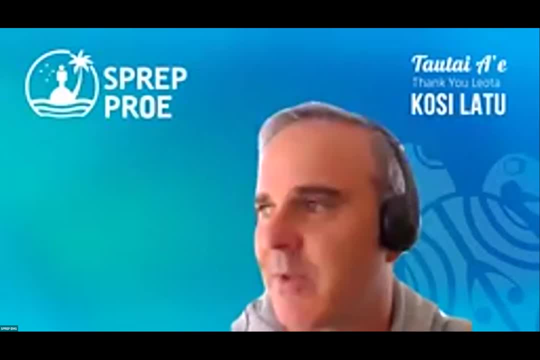 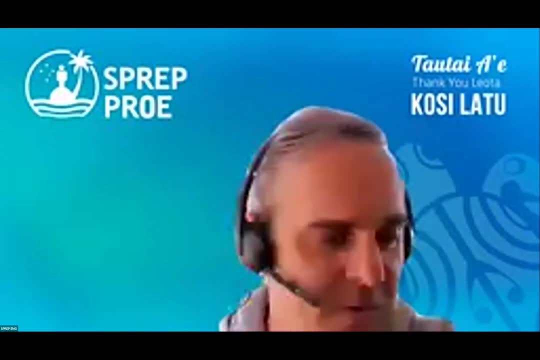 But if you don't, we can still take the questions and email them on to yourself If there's something particular you'd like to know, If there's something particularly difficult for us to answer. And also big thanks to Nick Valentine again for tuning in from his COVID quarantine in Lord Howe Island. 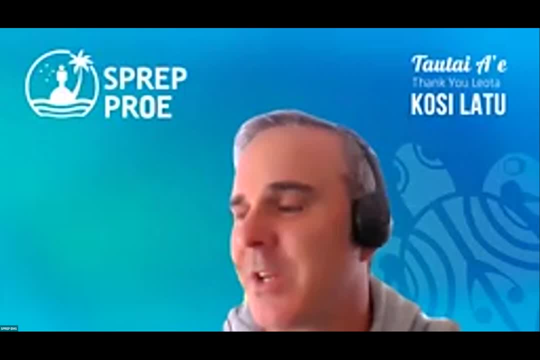 I hope he's actually feeling better. It was really good for him to join in and contribute, especially about Bonriki. Thanks again, Nick, And I'd just like to ask everybody to give a quick round of applause to our two wonderful presenters and thank them again for their marvellous presentations. 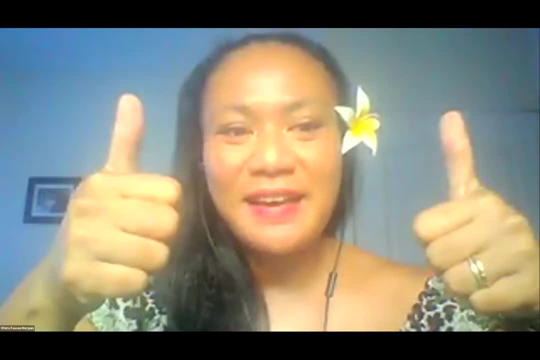 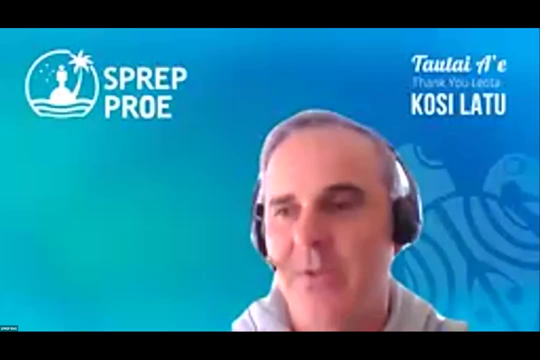 Thank you everybody, Thank you Thumbs up, And with that I'd like to thank you all for joining. Thank you, Nick, Wish you all a good day, Stay safe where you are and hope to see you all again soon next week for next week's presentations. 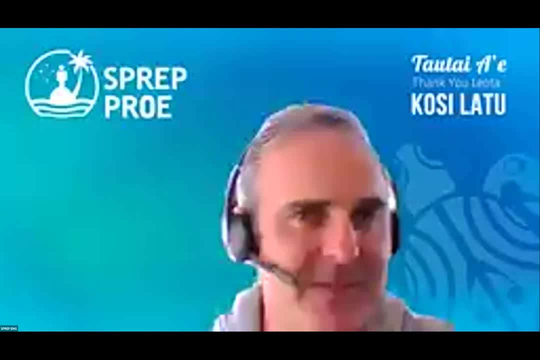 Thank you all and have a lovely day. Bye, Pass off the fort.